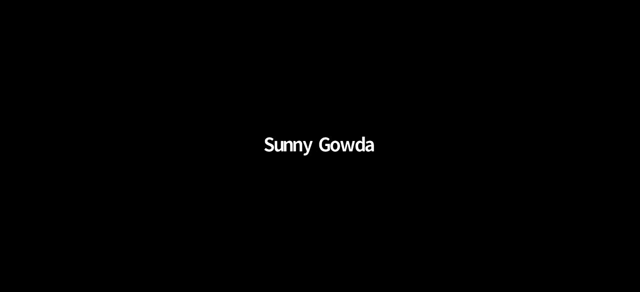 masonry wall in the year 2017.. He has worked as a project engineering in ARC Norway consultant and matrix consultant for about two years. Later, he worked as an assistant professor in RV College of Engineering for about five years. Presently, he is working as a lecturer. 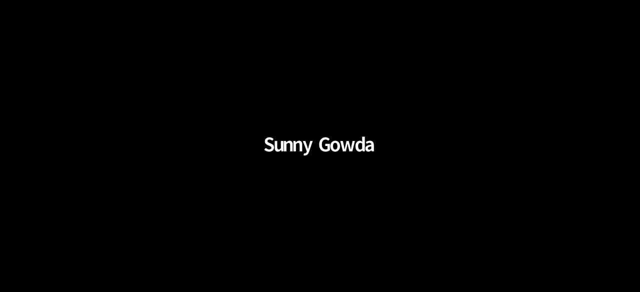 and assessment ed in Higher College of Technology, Muscat. His main areas of interest were alternative building materials, sustainable building materials and masonry structures. Many of his research projects were funded majorly: Strength of Hollow Concrete blocks for high-rise building as got 17.42 lakhs under VTU grant scheme and around five projects were funded in KSCST. 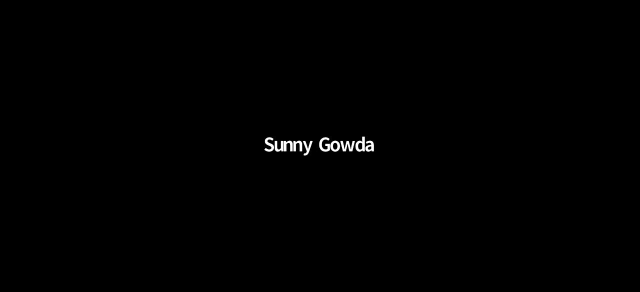 for the students under his guidance And he was the coordinator for HCU DCO Chair Program, which is set up at Department of Civil Engineering for about three years, which was granted for about 35 lakhs. He has guided for about 15 MTech students and 30 UG students. He is the member of a reviewer board in International 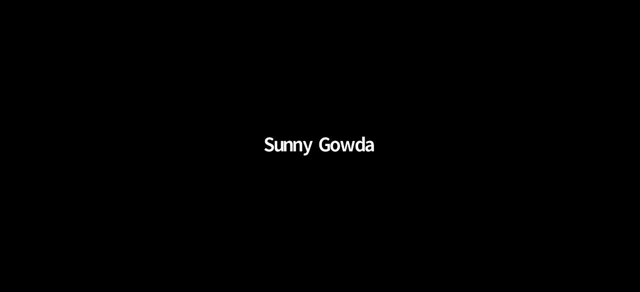 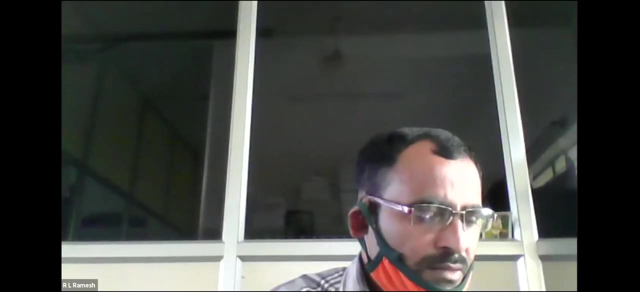 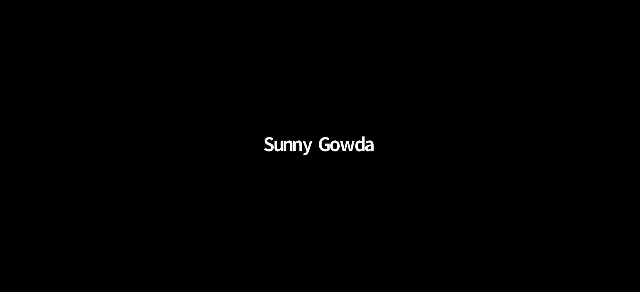 Journal of Scientific and Engineering Technology General. He has published about nine papers in various national and international journals. He is awarded as Best Young Researcher of the Year 2012 by ISET RVCE chapter. So, on behalf of Civil Engineering Department, EWIT, I once again welcome you, sir, for the webinar. Thank, 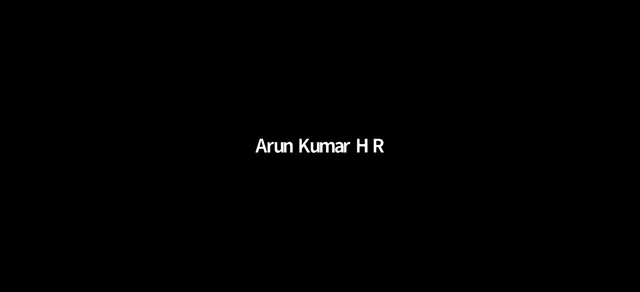 you, sir. Thank you, Sunny, sir. Now it's time to start the session. Dr Manjunath S Amalkul. sir, we are eagerly waiting to start a session. Yes, sir, Over to you sir. Yeah, am I audible, sir? 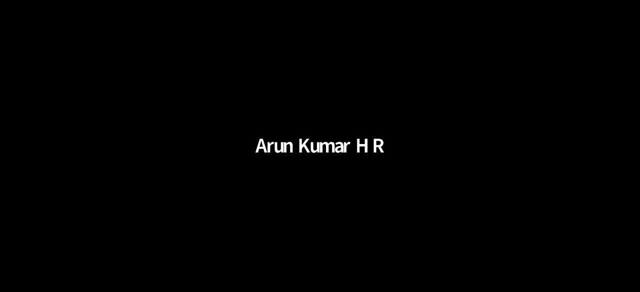 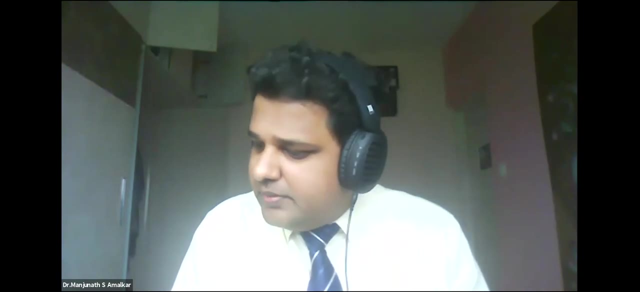 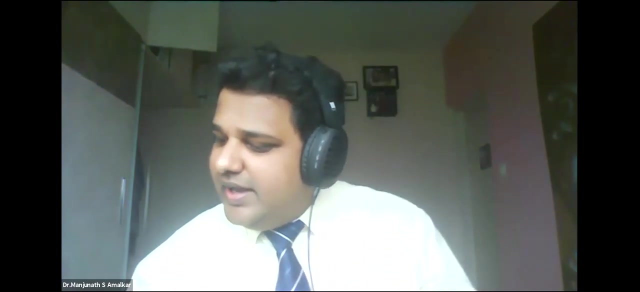 Yeah, yeah, Okay, Yes, sir, yes, sir, Yeah, perfect, Okay, Start and share your screen, sir, Yes, sir. Before I begin the presentation, I would like to thank the management of the East-West Institute of Technology, particularly Dr Chenna Keshavallu, who's the principal. 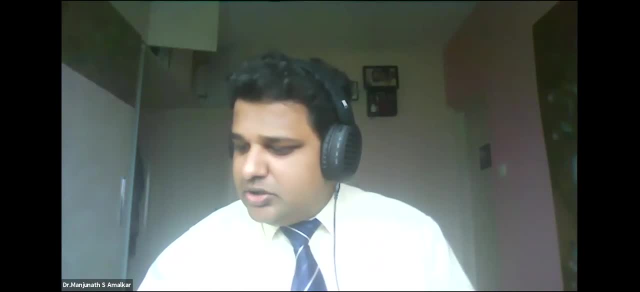 and director for East-West Institute of Technology, Dr Purushotham, director of East-West Group of Institutions, And my special thanks to the professor and head, Dr Nagaraj Gupta, for having given me this opportunity to share my thoughts on the set topic. I would also 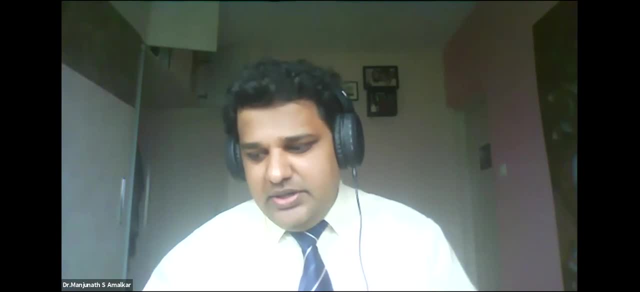 like to thank Dr L R Manjunath, the chairman for ICI Bangalore chapter, and also Dr R L Ramesh, the secretary for ICI Bangalore chapter. I would once again thank all the management of East-West Institute of Technology for providing me with this opportunity. Thank, 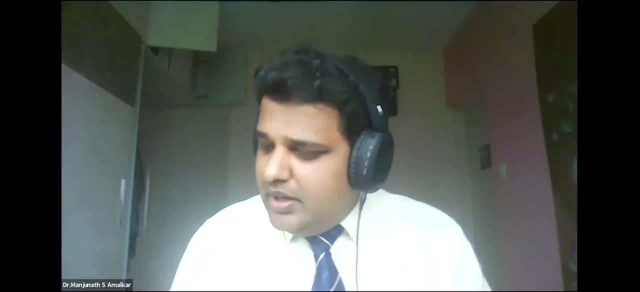 you, Thank you, sir, Thank you, Well, thank you, sir, Thank you also for providing this opportunity. And well, I would now, having said, and also I would also thank Mr Sunny Gowda for having given introduction. Well, now let's begin. 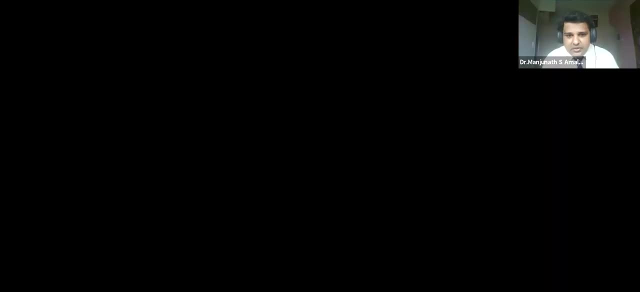 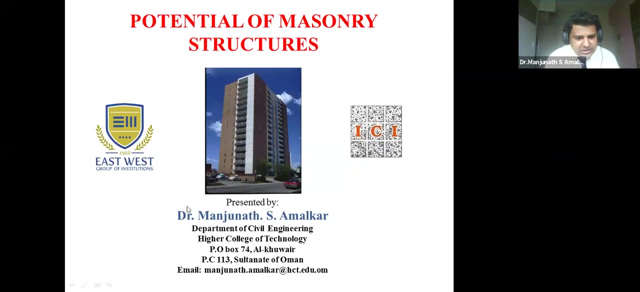 with the presentation. Can you see the screen? Yes, sir, yes, sir, Yes, sir, Okay, perfect, Yeah, Okay. Well, once again, welcome to all the participants for this one-day webinar. Because of the pandemic situation, I think you know, I think we have had this opportunity. 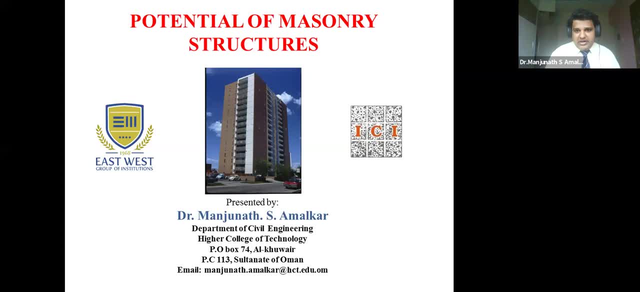 to have the online, you know- seminars or the webinars, in order to keep our academic knowledge going Well. on that thought, you know, today we would be discussing about the potential of masonry structures. Well, when we talk about potential, well, in this presentation, you know, we would look. 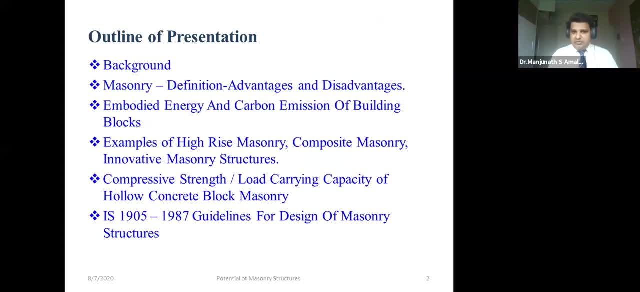 at both aspects. One is the structural potential as well as the architectural potential of masonry structure. The presentation outline would go something like this: We would look into the background of understanding the fundamentals of masonry, Wherein we would like to define what is masonry, what are the advantages and disadvantages. 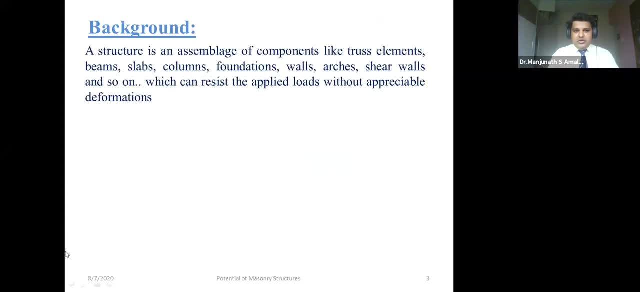 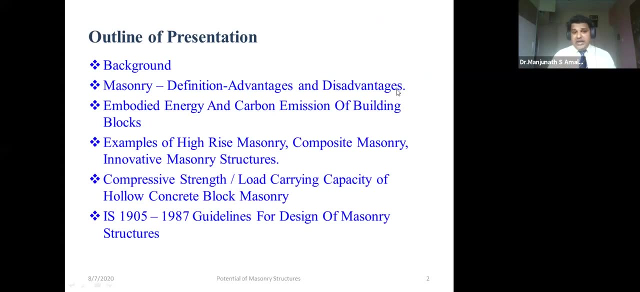 of masonry, And talking about- you know masonry- I think one has to also look up upon it as an eco-friendly material. So we will also see what are the embodied energy and the CO2 emission. you know which? 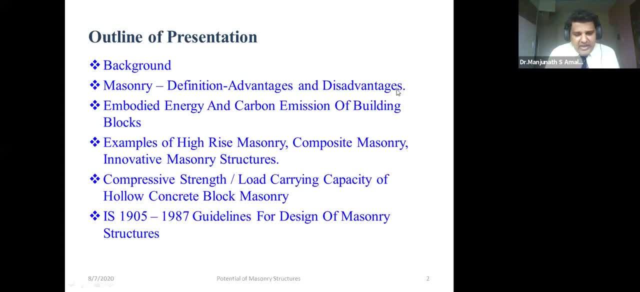 is emitted using some of the building blocks, what we have which can be used for building blocks And, of course you know, talking about the potential, we would also see what are the some of the examples we have in high rise masonry, or maybe some of the examples for 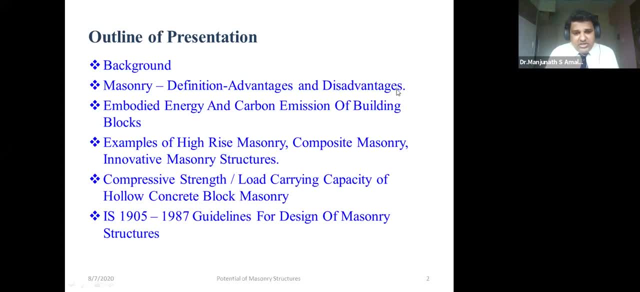 composite masonry and some of the innovative structures which are, which are of greater importance. Finally, we would look into, you know, a little bit of the design concept. I would not, although it's a broader topic. I would just, you know, briefly talk about. 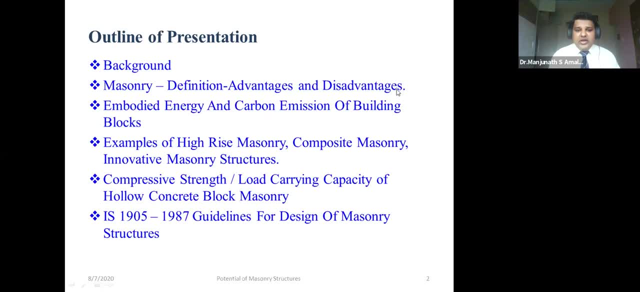 you know, briefly discuss about how do we go about assessing the compressive strength of masonry in general- And you know I would have some numbers on hollow concrete block masonry as well- And, in a nutshell, we would also look into the. you know the guidelines as prescribed. 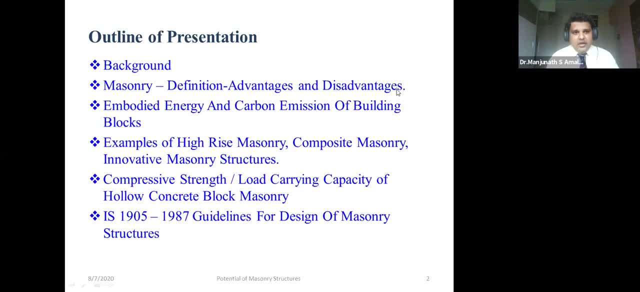 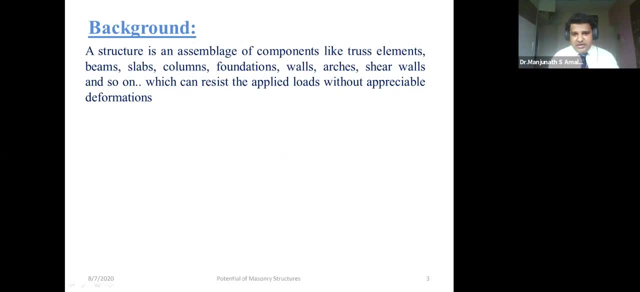 by the Indian standards 1905.. Well, all of us know what is the definition of structure. as it goes, a structure is an assemblage of components. Okay, So structural components maybe a beams, slabs, columns, foundations, all these are. 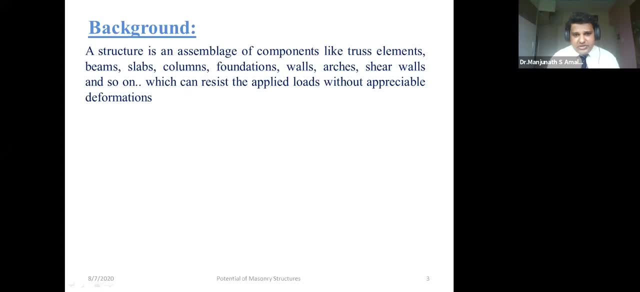 assembled together And that that is what constitutes a structure. And these are the ones which are are applied or other, or rather the ones which resist the applied loads without any appreciable deformations. You know, we have come across various forms of structures and you know. just to talk briefly, 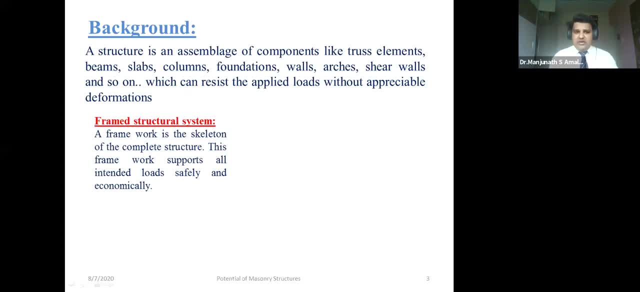 about the following: The forms which we usually use, well, one which everybody is familiar with, is the framed structure, where it's also called as the skeletal structure, where the, the members, the structural members, like I just mentioned- the beams, the columns, the slabs are the ones which 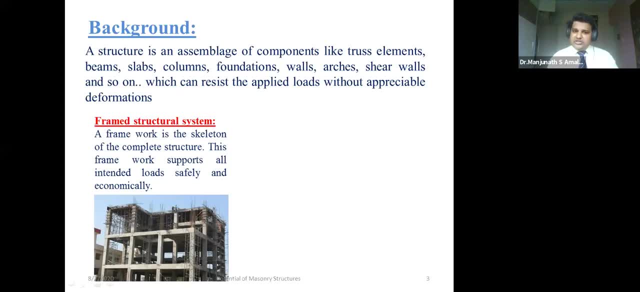 are supposed to carry the load. Well, wall just plays a role of a partition or just an infill. So this is a typical. I'm sure each one of us have seen Such structures, which is a typical RC frame: the structure, but the other option, what? 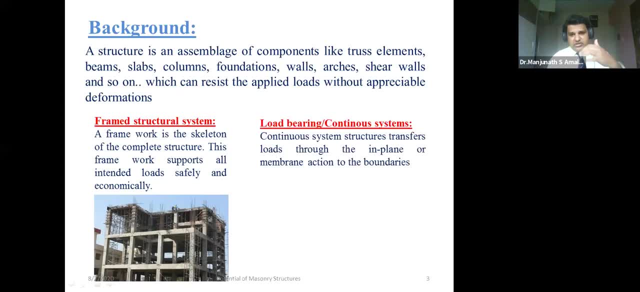 we have is a load bearing structure, or sometimes, you know, you can also refer to this as to a continuous system. Now you heard, the loads from the slabs are directly transferred on to the walls, or to an in-plane, or to the member action, to the boundaries. not typically one such load bearing. 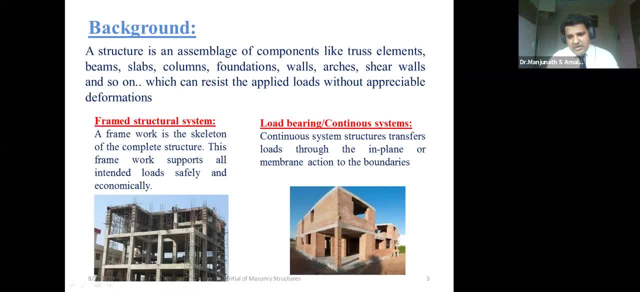 structure, Would that be of a, of a, of a masonry building, What we have here? Okay, So, uh, where the the loads from the slabs are directly, you know, resting on the walls, and the walls are the ones which are supposed to be carrying the loads. 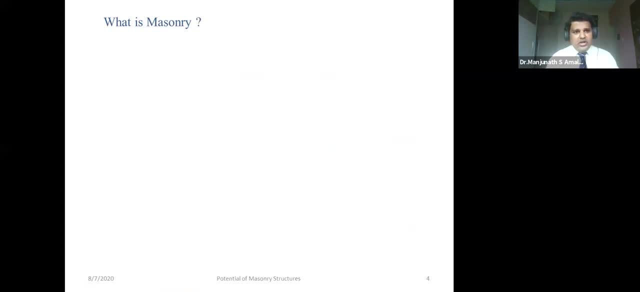 Now, having looked at the forms of structures, and let us go uh, understanding the term masonry. I'm sure all of us have heard this word: masonry. well, uh, we, can we? uh, we usually call commonly, uh, as it as, walls. 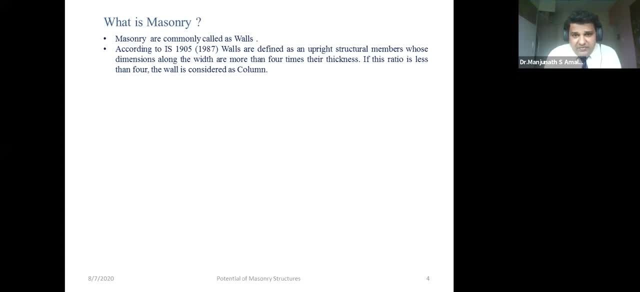 And as for the chordal, uh rest, Uh. recommendation: walls are defined as an upright structural member whose dimensions along the width are more than four times their thickness. Now, if I'm looking at this as a element, uh, which I would want to call it as a wall, well, 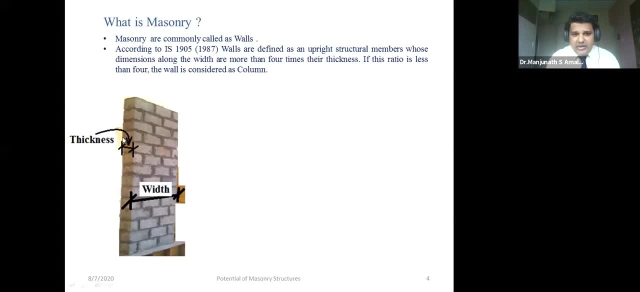 it's width. you know, uh has to be at least four times more than the thickness. Well, if, if, if this condition satisfy, that is when we can call uh an element as a wall. Uh, on the contrary, if, if uh it is uh, let us say, less than four, then we would have 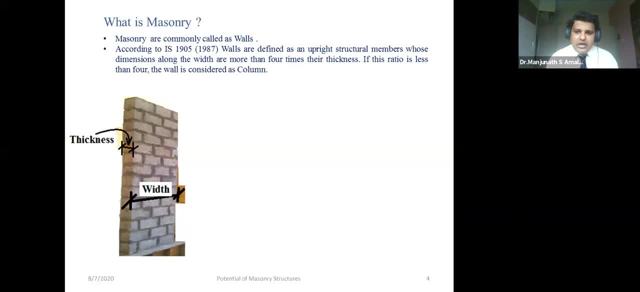 to design it as a column, a masonry column or a pier, And based on the configuration, structural configurations, uh, and of course the functions of the walls or the masonry, can be categorized as something called as load bearing walls and non load bearing walls. 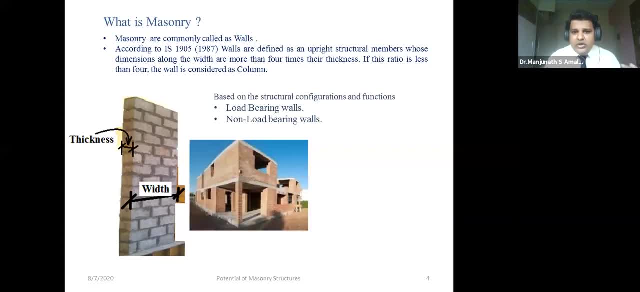 Now, what are load bearing walls, as the name goes? you know, though, these are the walls which are Supposed to bear the nodes. well, the nodes from the slabs which are being directly placed on the walls, and the walls are the ones which are have to take all the load onto itself. 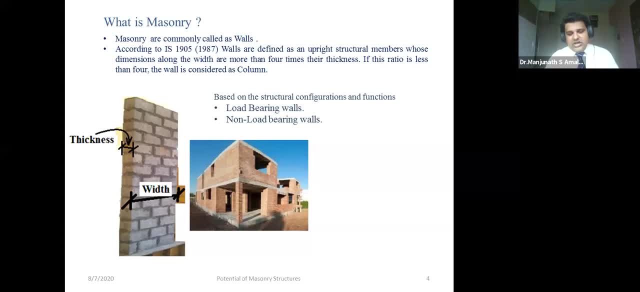 And then, of course, you know, uh, you know, subsequently, the walls are being constructed one above the other, and they are the ones which are the members which are resisting all the nodes. Well, the other option, as we, as we I mentioned in the beginning, is a non load bearing wall. 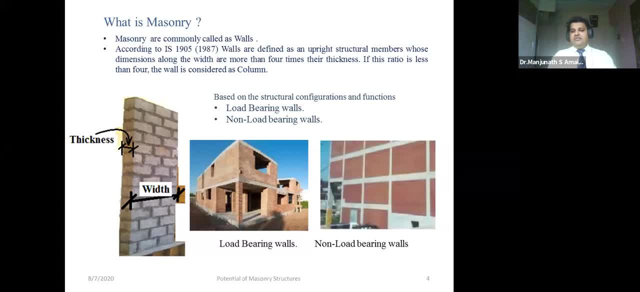 And as the, as the name goes. So again, uh, it is a one which is being used just to fill the frame and it is not, you know, expected to carry any load. All the loads are carried by the structural members, that is, the beams. and then to the. 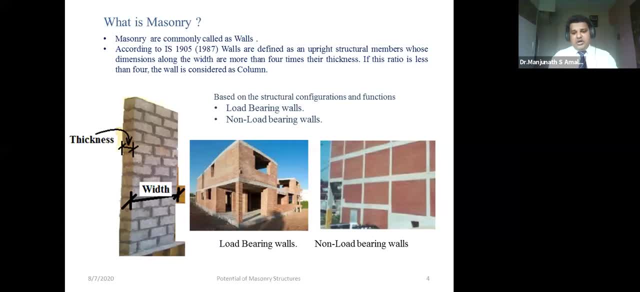 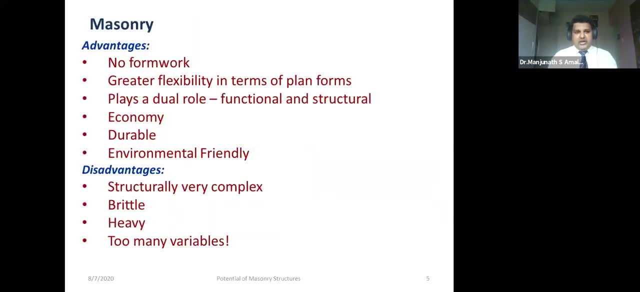 columns and then to the foundation, when, uh, you know, the walls are just, you know, filling in the frame Moving ahead. Now let us understand. what are the advantages and disadvantages? uh, advantages of masonry, Well, uh. 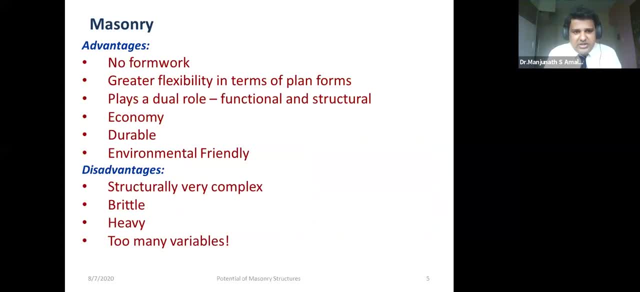 Advantages: Yes, Uh, because it's a prefabricated structure. well, there is no form work uh required. There is no curing, unlike uh concrete structures. Uh, well, there is a greater flexibility in terms of the plan forms. 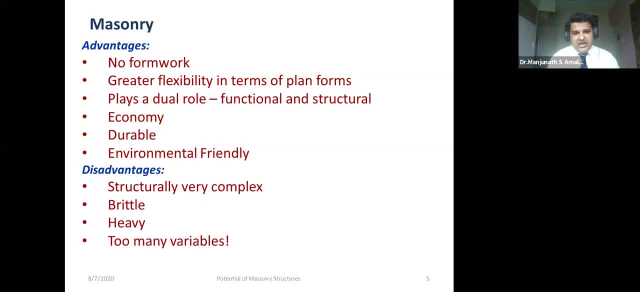 Uh, it has both, uh, functional as a structural load role to play And, yes, it, it- you can say it- to be economical. also, again, depends on what is the building unit, unit is trying to use And uh, of course, it is durable. 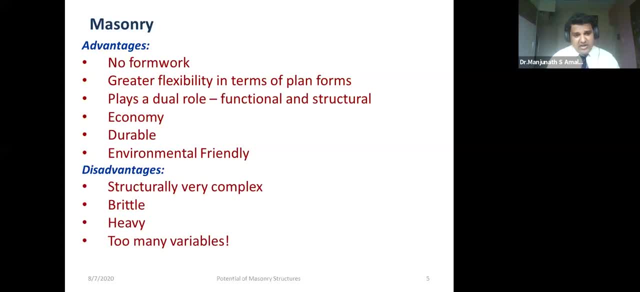 Because we have. we have several examples of masonry structures which have been maybe built uh, uh, several hundreds of years, if not more, uh, which are even standing to do to this day. Yes, For for that, uh, from from that we can, we can say for sure that it is certainly durable. 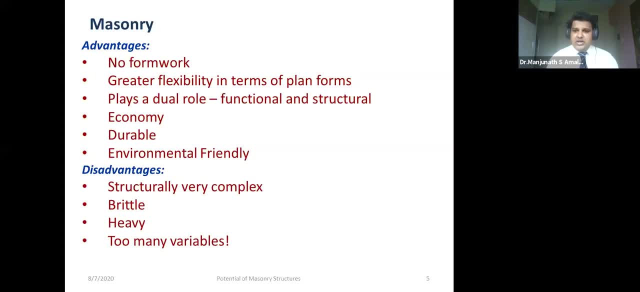 And uh, of course- and we're on mental friendly- because you know, there is uh, uh, you know uh, less number of, uh, less amount of energy, uh, which is consumed, and uh also the carbon. 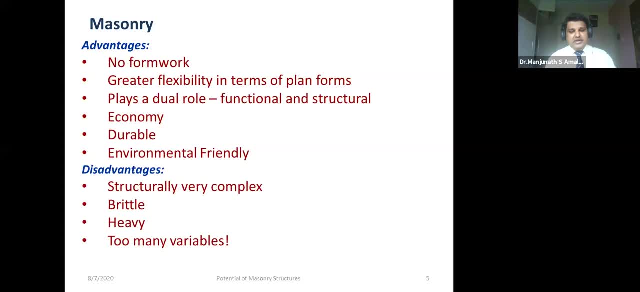 dioxide emissions- Uh, carbon dioxide emissions is also far less uh than its uh other counterparts. Uh well, at disadvantages like any uh uh technology. uh, it will. well, we have this uh disadvantages with masonry as well. uh well, uh, you know, it is structurally. 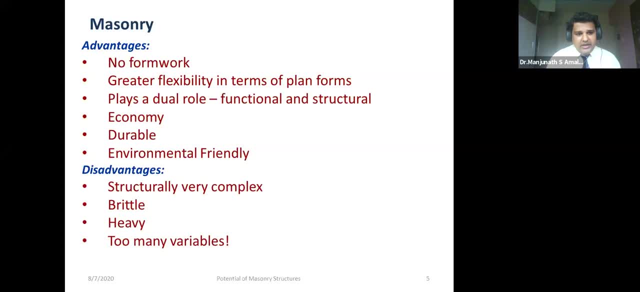 very complex. Uh, of course it is brittle, uh and uh, because you know, if you have to construct it for a high rise masonry, well you know, you end up getting, uh, a very heavy structure. 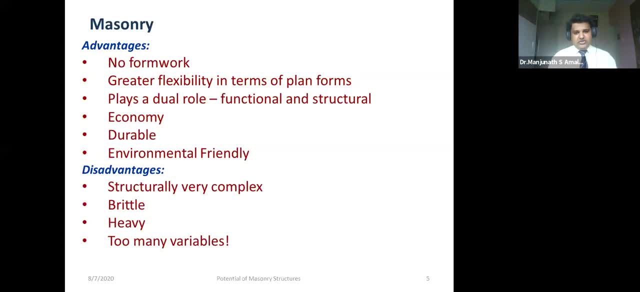 for sure. And uh, of course, there are too many other variables which are also involved: making uh the design, uh you know, a little more complex. uh, when these are the disadvantages of masonry, Let us uh try to compare the two, uh, you know, material. 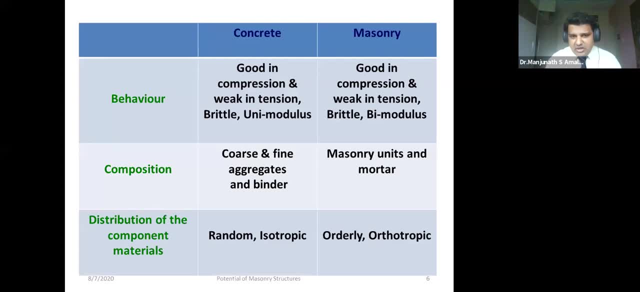 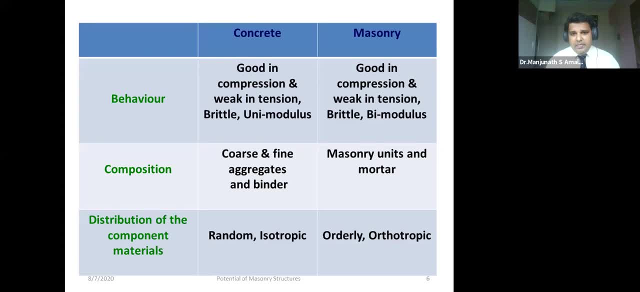 masonry does not do double right And I had any question at the end. This showing the common That the side only works when they're consistently in the expression in compression. They are equally both, equally good in compression and a cause you know, in concrete one can. 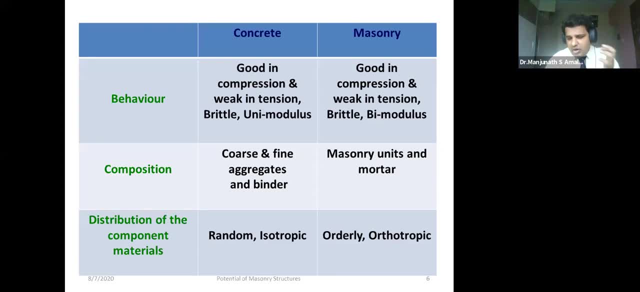 go both with uh, you know, making uh, uh uh better, Jesus mix design And uh, you know, one can achieve a uh better strength. but it goes with uh at modulus material, while the masonry is a bimodal and in terms of its composition, 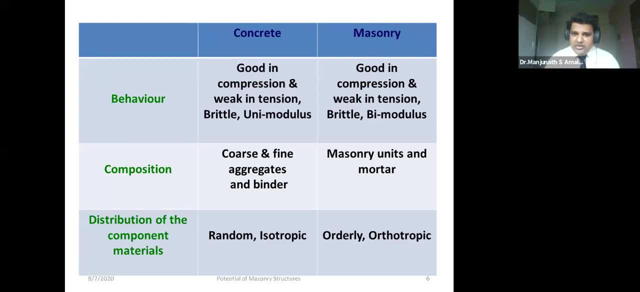 well, you know, as we know, all know, concrete is made up of fine aggregates and the coarse aggregates. of course, with a binder, well, depending on what is the binder used, you can have a cement concrete or other. you know other types of concrete as well. well, in masonry, you know, we look at these are the masonry. 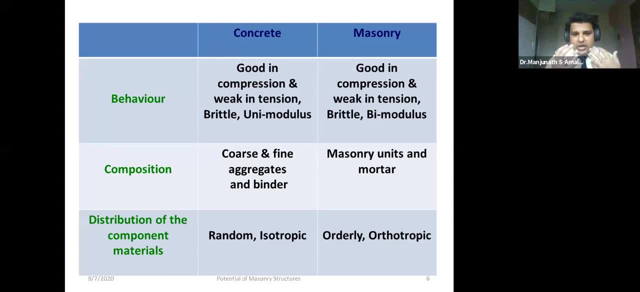 units and the mortar as two key. you know ingredient composition and masonry units. you know, can you have various options. we will, of course, see a little later what are the options one have when we talk about masonry units. of course, these masonry units have to be stitched together, so that is where the role of 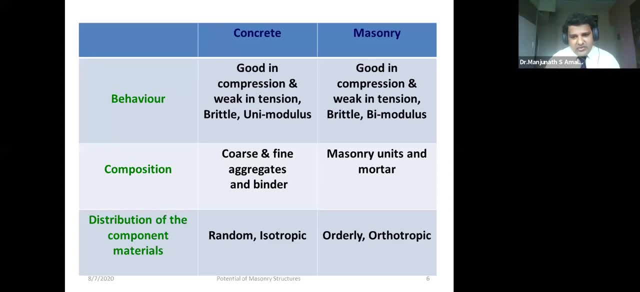 mortar comes in. well, we also have different mortars which one can use for going about with the construction of masonry, and you can see that the masonry units are made up of fine aggregates and the. and talking about the distribution of component materials, yes, concrete it's. 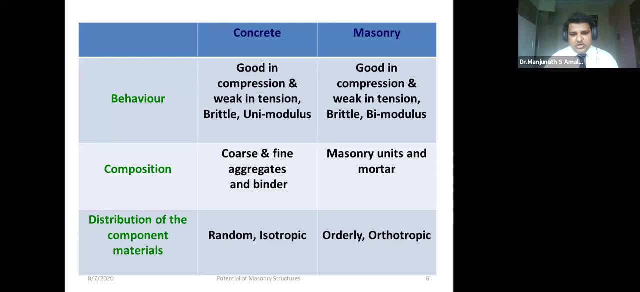 very random and of course you know it is isotropic, having same properties, all possible sections, whereas masonry, well, the distribution is order, orderly and well it behaves like an orthotropic material. you know one of the options we have in masonry units. well, you know we have a 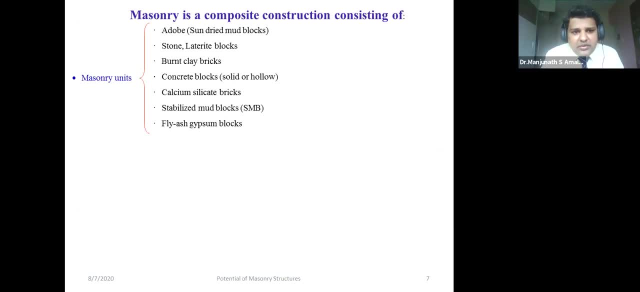 we have you know, seen or maybe heard our and seen these options. well, we have adobe. these are basically rammed earth or which is sun-dried mud blocks. we have the stone or the laterite blocks. we we use very oftenly the clay, burnt clay. 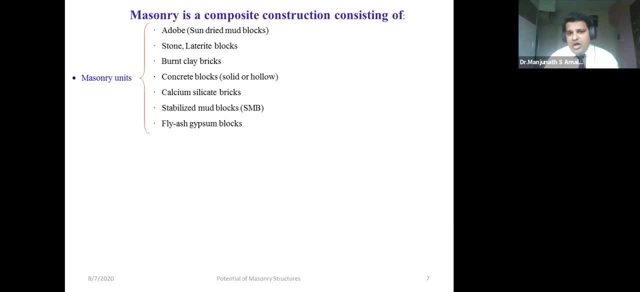 bricks, of course, concrete blocks, which can be solid as well as hollow, and you have the calcium silicate blocks. then you have stabilized mud blocks, you have gypsum blocks, or you have a quadcutter block. you have, of course, we have the, because there are a few more additions which have not been included here. Geopolymer blocks are the. 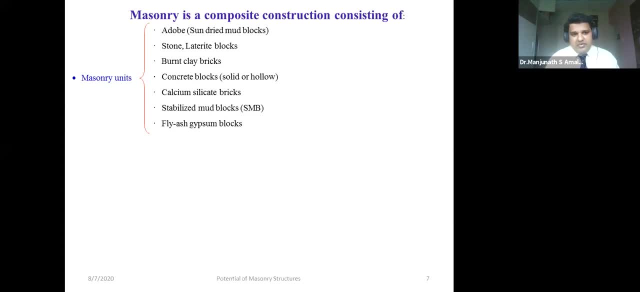 the new ones which have been added into the list of masonry units. Well, you know, what is the block or what is the type of unit one has to use will depend, purely depend, on what is the requirement. and of course, you know, talking about stitching the masonry. well, you have a mortar which does the job. 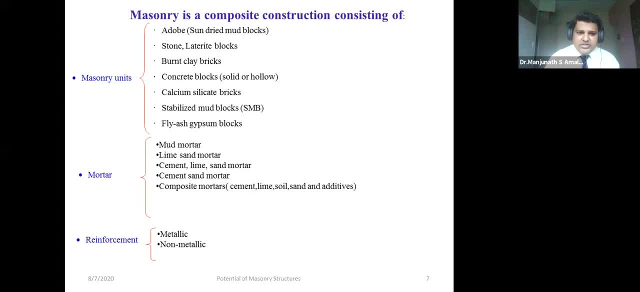 for us, and you know, traditionally we have been using the mud mortar, the lime sand mortar, and then, you know, after the after the invent of the cement, you know we started using the cement or cement sand mortar, or sometimes, you know, we also try to use the composite mortars. 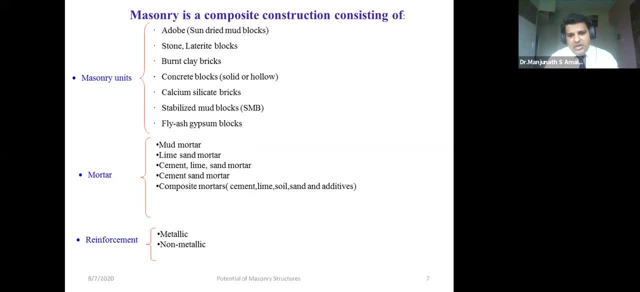 which is a combination of cement, lime sand. of course, you know, depending on the requirement, one can go ahead with some alternatives also. Well, when talking about reinforcement- yes, we do have, you know, structures built out of masonry and you know it could also be reinforced. when we talk about reinforcement, one option is, of course, the metallic one, which is traditionally 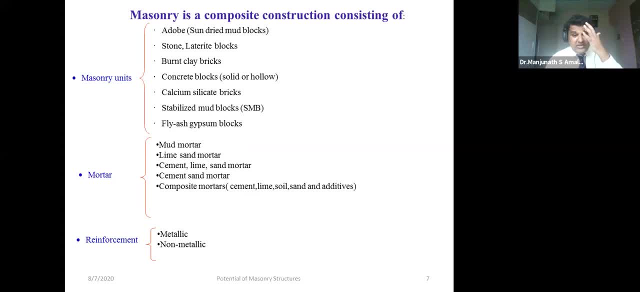 also used. I mean, it's also used as a reinforcement in the concrete structures. well, the same can be used even in masonry structures. but that that is about the metallic option. well, you know there have been, you know, bamboo sheets or bamboo strips which have been used as 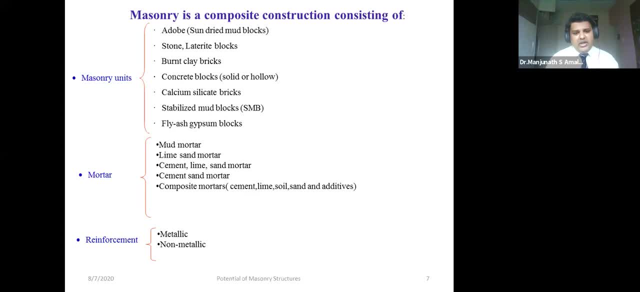 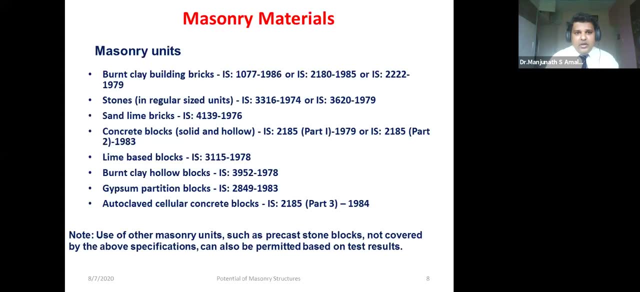 reinforce. reinforcement, you know, in order to make it a little better when it comes to any lateral loading. well, I just bought what up this so has to refer. when it comes to any of the design of masonry or any of. well, this is just bought. for that reason, 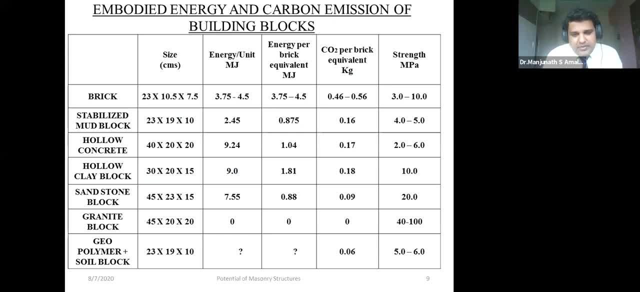 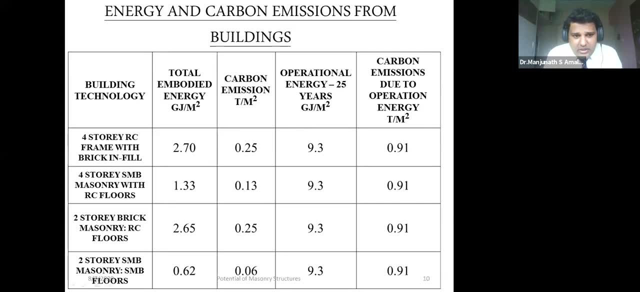 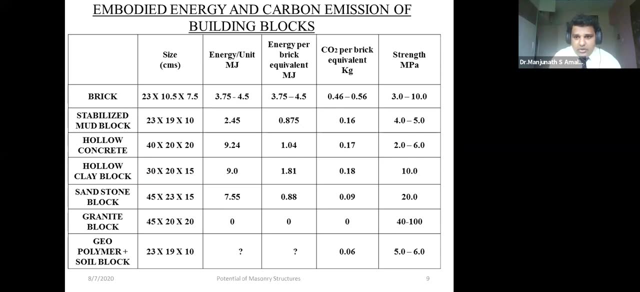 now talking about, you know, masonry as an energy efficient building. now, this is a very important aspect which has to be understood. it has to be understood hello. well, you know this is a very important aspect. if you look into, you know the ones which have we have been using. 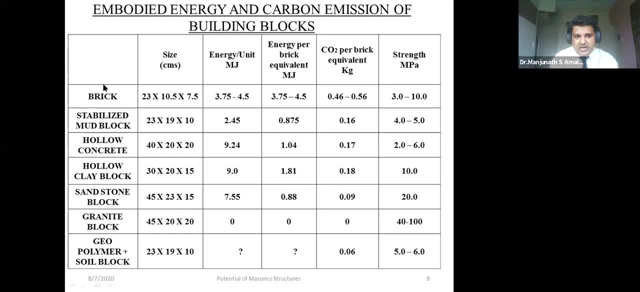 the bricks. let us let us try to compare the energy consumed with keeping brick as a standard and let us try to look at the other alternatives you have as a building material or a building block. now you know this particular table gives us, you know the amount of energy, what is required to 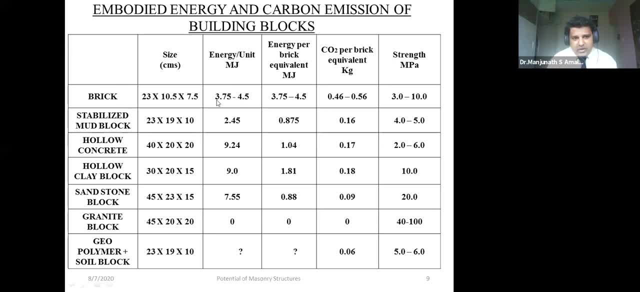 produce a unit, block of masonry unit. now, if you look here, you know the amount of energy is somewhere around 3.75 to 4.5 megajoules. well, what, what is that which constitutes this energy? one is, of course, you know, the transportation. 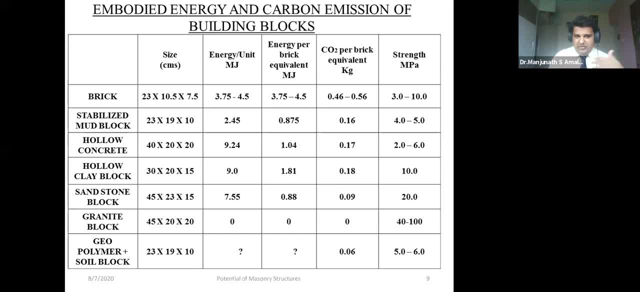 cost. and the other one would obviously be, if you're talking about bricks, it would be the brick, or the burning cost of the big, rather the burning energy required, you know, to produce the bricks. well, these are basically the two parameters which which has to be analyzed or which has to be taken. 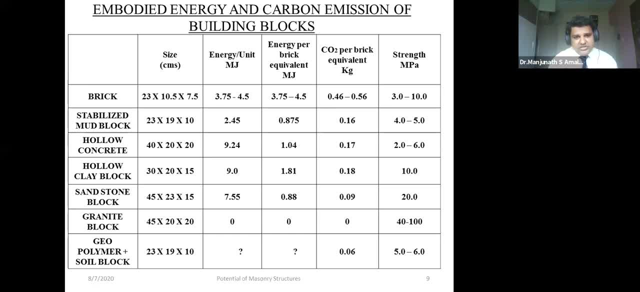 into account one, while one is trying to find out how much is the energy required. now, looking at the carbon dioxide emission for a big is somewhere around 0.46 to 0.56 kilograms, and if you compare you know the other alternatives as equivalent to the brick. well, you can notice that there is a 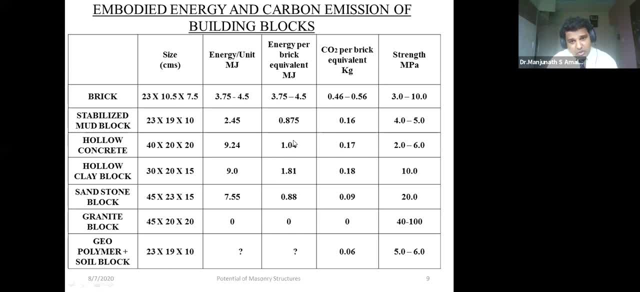 significant reduction in the energy required, as well as there is a significant reduction in the carbon dioxide emission also. well, you know well. this shows that if, if one can use these alternative blocks, they would be a significant reduction not only in the energy consumed, but also in the carbon dioxide emission. 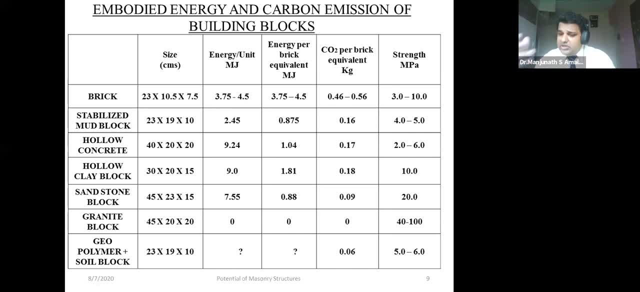 well, this is quite important to understand because you know there is a dubious distinction. you know, i know that india is the third largest emitter of carbon dioxide, after the united west and china. but you know, for that reasons- i think you know, one has to be taking, taking the environmental also into account. one has to be very conscious when, when we select, try. 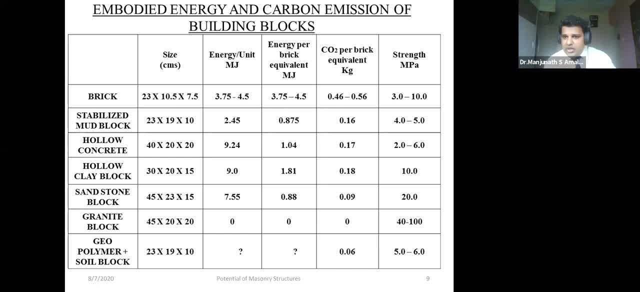 to select a particular unit block. well, the last column here gives you a range of strength, uh, you know, for various, for all these um blocks. however, i think the ones which i did mention, geopolymer blocks and the soil blocks, these are the new additions of masonry units. well, one has to, you know. 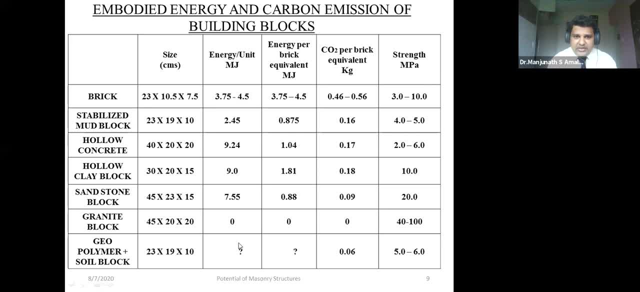 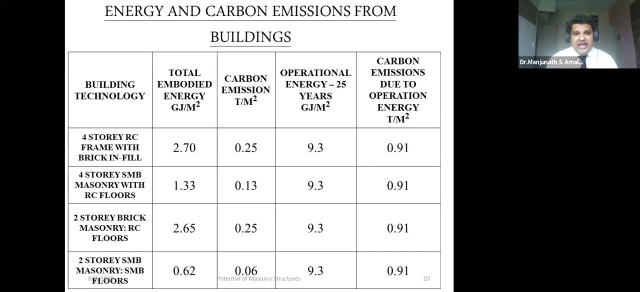 will try to you know, find out what would be the amount of energy which would be required to you know, produce such blocks. well, the strength is quite promising, which is five to six mpa. let us look into what is the amount of energy now if it has to be used for a big, for a particular building. 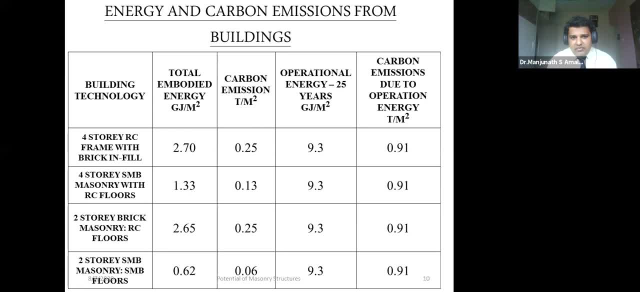 technology now keeping you know we. i have these four columns here now: the two with respect to the operational energy and the, you know, carbon dioxide emission. these are the operational energy, so i have kept this as constant. well, well, it is nine, taken to be a 9.3 gigajoules per meter square. 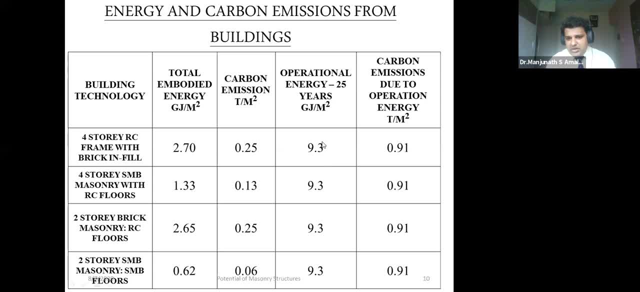 well, the number is got from. you know, just uh, looking at an average indian family using uh how many kilowatt heart per annum. and then you know, looking at a period of 25 years as an operation, uh well, we end up getting this value of 9.3 gigajoules per meter square. but like keeping this as constant, let us look into the. 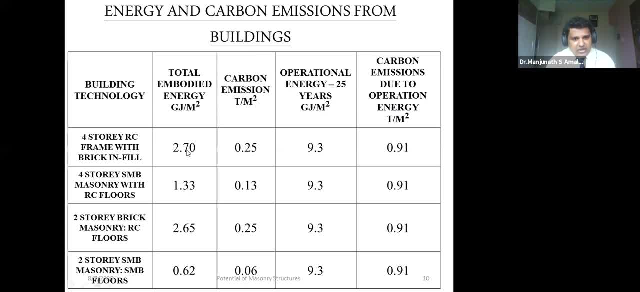 building technology and how much of energy- uh, you know, it is it- it is used and what is the amount of co2 emission. now, if i have an option, like i'm going with a four-story rc frame with, uh, you know, a brick in film like the ones where we talk about, talked about the frame structure. 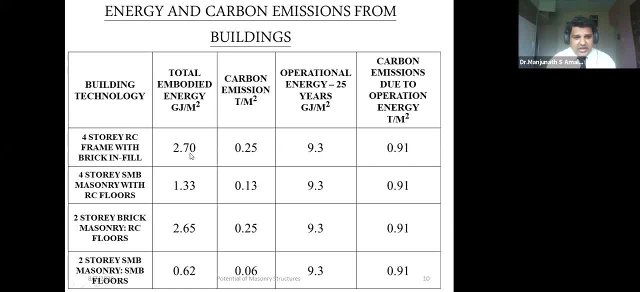 well, the total embodied energy is 2.7 gigajoules per meter square and the co2 emission is around 0.25 tons per meter square. now, if i have to, let us say i, i go with the same four-story, but not with a frame structure, but with a masonry structure. here i have used the 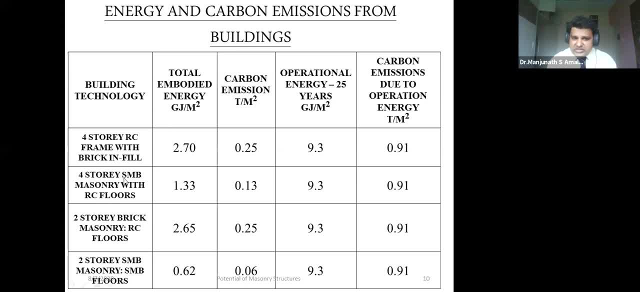 word smb, where smb stands for stabilized mud block masonry. now, if this is an option, which i'm going with, and having normal conventional rc floors, well, you see that there is a significant reduction in embodied energy and also the- uh, you know- co2 emission as compared to the previous one. now, 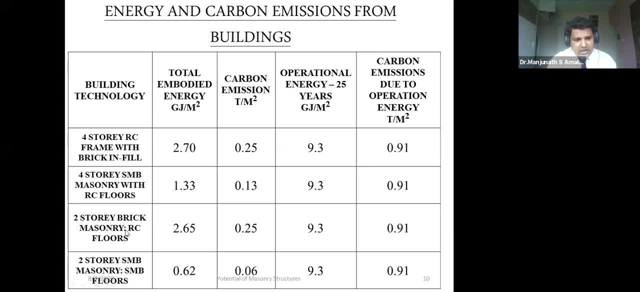 if we have to compare, uh, the two-story building, let's say, uh, you know, with the two-story brick masonry. now, this, these two comparison is only among the masonry. now, let us say i have a two brick, two-story brick masonry, uh, with, uh, conventional rc floors, rc floors. when i say 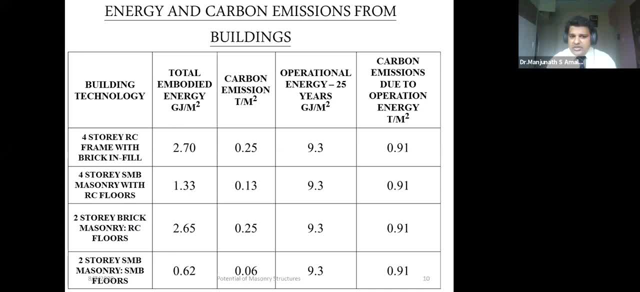 rc slabs is what i meant. uh, you know, it requires something around 2.65 gigajoules per meter square. uh, if i, if i choose, rather than a brick masonry, an alternative to this, if i, let us say, i choose a stabilized mud block masonry and not have rc floors, but then have stabilized 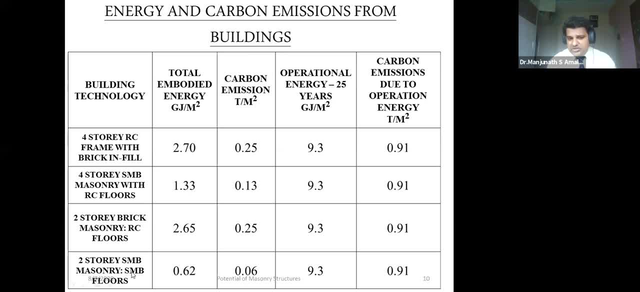 mud block, masonry units itself as uh being used as a floor, then you know there is a significant reduction in the amount of total energy which is, you know it's, which is, which is evident here, which is 0.62 and 0.06 for uh embodied energy, which is 0.65 gigajoules per meter square. 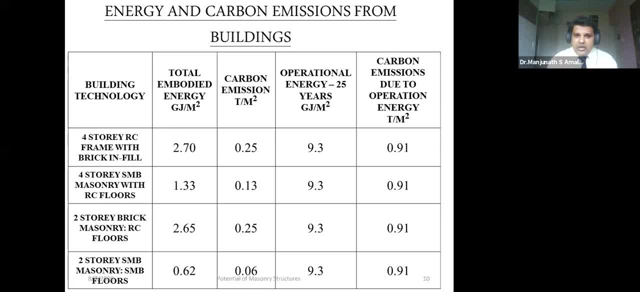 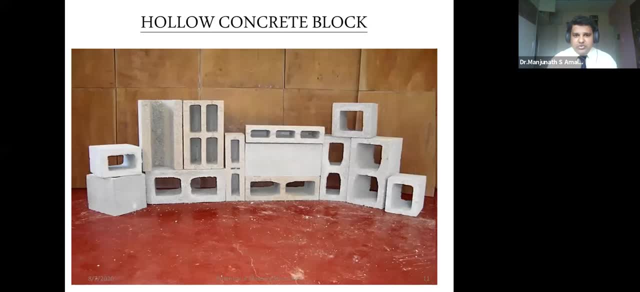 energy and co2 emission respectively. well, going ahead, uh, talking about the masonry units and uh, what are the alternatives we have? well, this is one alternative which is being extensively used. uh, you know, it used to be hollow concrete blocks which are, which were sort, rather the solid concrete blocks which were being done, uh, using a very, uh, crude method earlier. 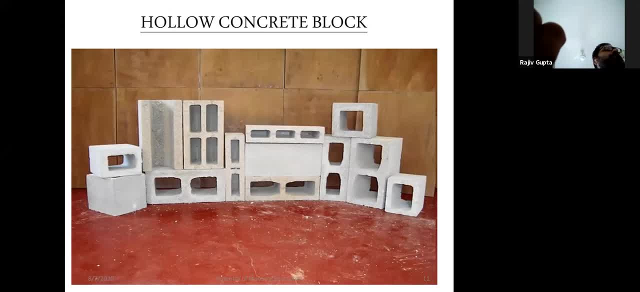 but now there have been a lot of manufacturers who have, you know, kept a better quality control and, uh, who are, you know, in a position to make a good quality hollow concrete blocks. now, what? what you see on the screen is, uh, hollow concrete blocks with various sizes, various shapes and, uh, and sizes. 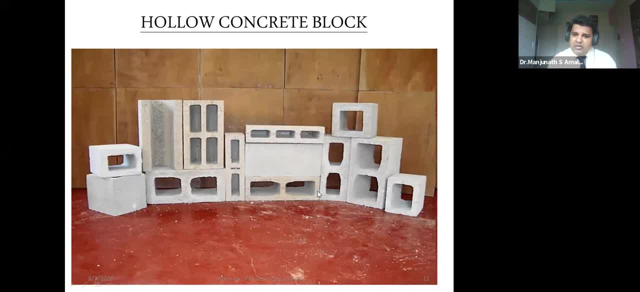 of for various, uh, you know, purposes. uh well, some of the blocks- you can see that the holes are through, uh uh, from the throughout the height of the block. well, there are, you know, which are not having two and two holes. they are hollow but they are not having two and two holes just to facilitate the. 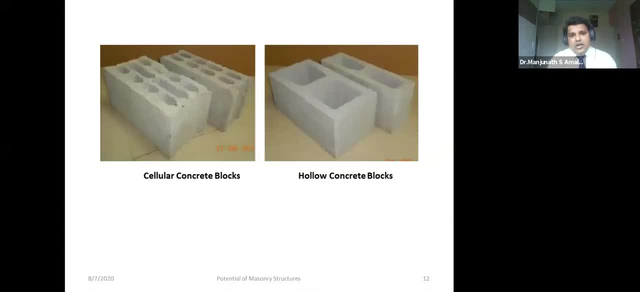 the placement of the masonry units. so that's one of the advantages of the masonry unit is that you can. masonry unit is that you can uh, if the hole is, you know, enough in width to get a ten square meter. uh, double flat instrument or smaller, with only one hole you can attract a ten square meter. 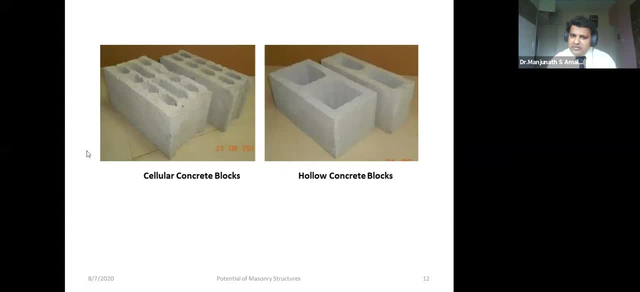 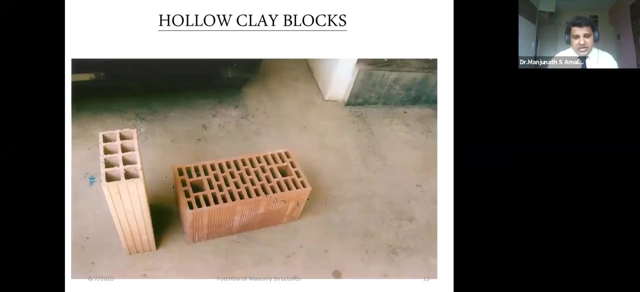 please, but more in number. we usually refer to these blocks as cellular concrete blocks, And the ones which are with the larger holes we can refer it to as the hollow concrete block. Now, the other option is, of course, these clay blocks. 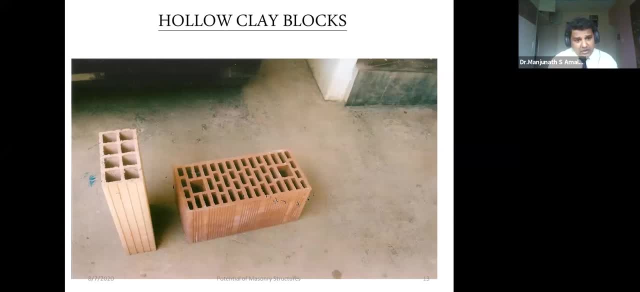 Well, there are a lot of manufacturers who are making a very good quality clay blocks which are being used, although for a mixture, as an infill as well as a structural masonry unit. Well, the advantage is it's very light. 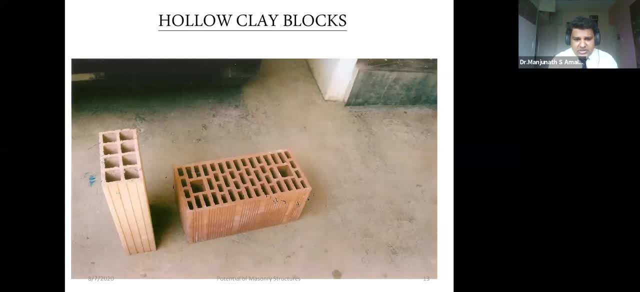 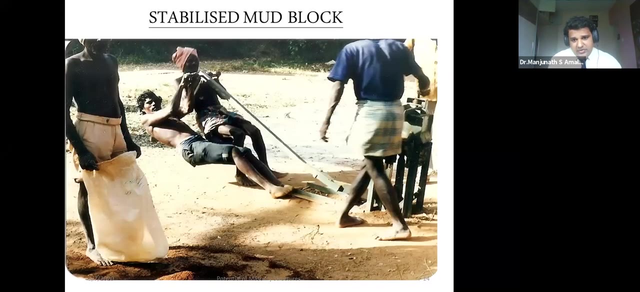 It's very light with the kind of number of holes present, And you see that there are provisions for even placing reinforcement and perhaps grouting it later, depending on what is the purpose of usage. Well, this is the one which is actually the brainchild of Astra Indian Institute of Science. 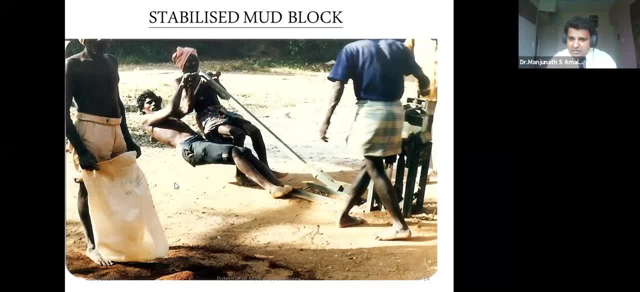 This is the press which is called as the Press which is made used to produce the stabilized mud blocks. It was under the guidance of Dr KS Jagdish, who was the director for Astra Indian Institute of Science. 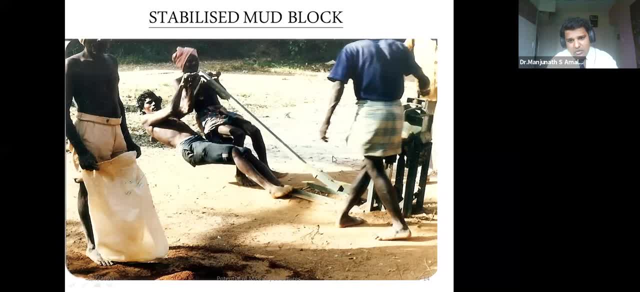 who has actually designed the machine? Well, the blocks are just made by processing sandy soil with a certain percentage of stabilizer. Maybe one can use, But they don't have a lot of strength. Well, the best is to make a concrete structure. 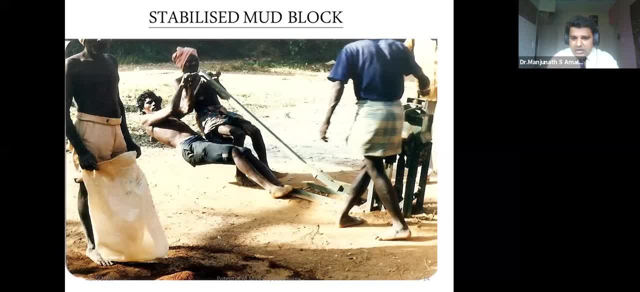 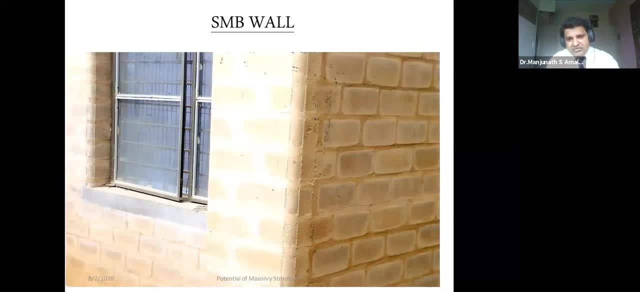 where you can put cement as the stabilizer And then it just has to be pressed at the optimum moisture So one can get blocks which would look something like this, Although I do not have a picture of the block, but then I have a picture of the masonry here which is being 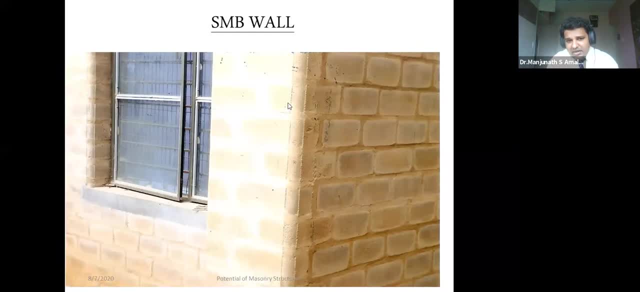 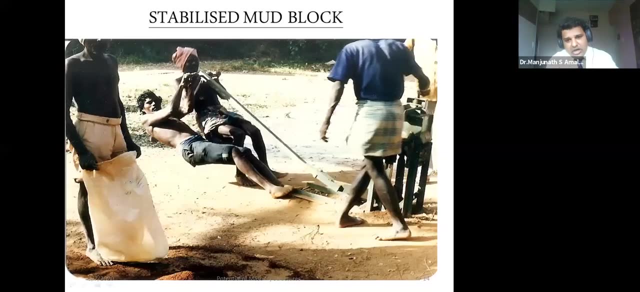 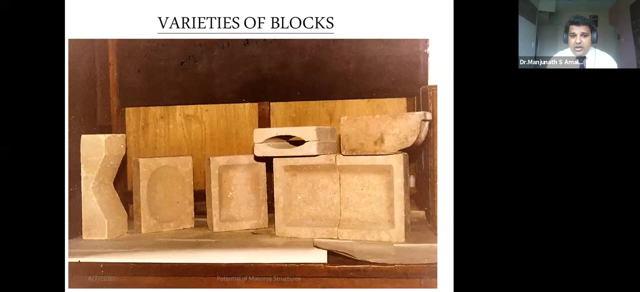 or the wall which is being built using this stabilized mud blocks. One can do it here as well. one can get it done using the same press, what I, you know, I did mention a little while earlier Now, not only you know rectangular blocks, but then one can, you know, produce blocks of various shapes and various sizes for various, you know, purposes. 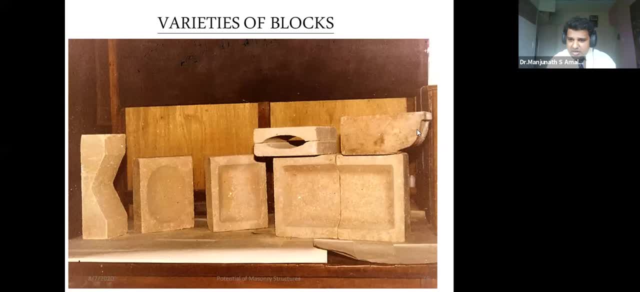 If you want to have it as a carnage here. so one can maybe produce blocks and, depending on various applications, one can produce blocks of various shapes and various sizes. Well, you see here the block which is having a depression here. We will of course discuss these types of blocks a little later, when we look into the applications of these blocks. 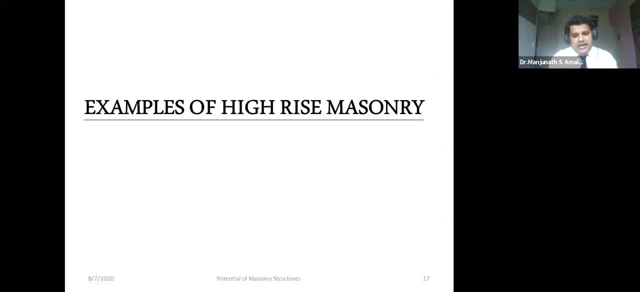 Well, you know, we understand that. you know masonry blocks. structural masonry is one of the oldest building methodologies and by far the most resilient, Right from the the Egyptian pyramids and Roman Pantheon to the Vatican and to the Baltimore. 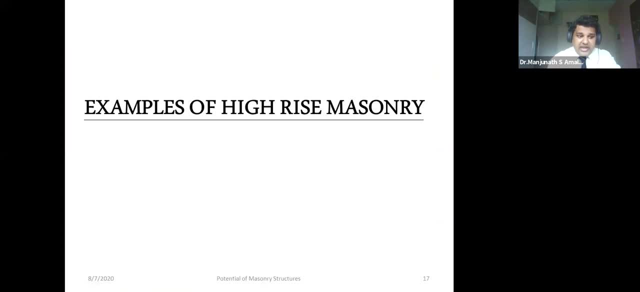 there have been stone and brick masonry that have been used to build. you know, the world's most iconic and enduring structures, You know. just let's say, let us also look into those iconic and, you know, innovative structures a little later. 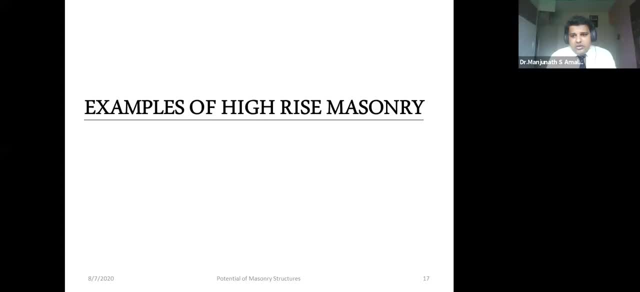 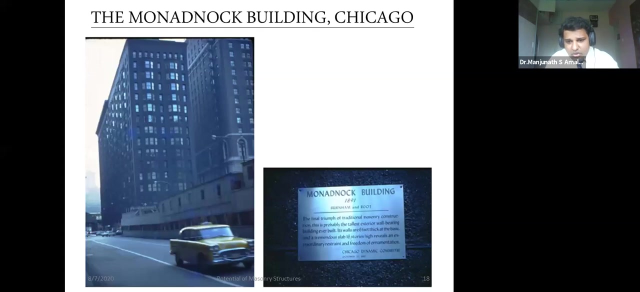 But let us look into some of the examples where high rise masonry have been used. Now let us first start with the abroad, So the, the building which was built in Chicago, the Monad Nock building, you know, which was built way back in 1891.. 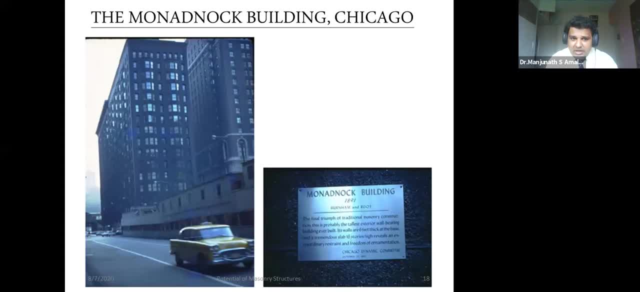 Well it's, it's a 16 story high building. Well, the thickness, you know, was definitely had to be more because it was all masonry, which was which had to support the load coming on from the superstructure. Well, the thickness at the base was, you know, roughly about two meters. 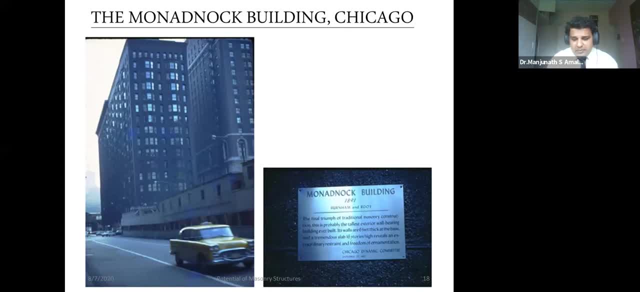 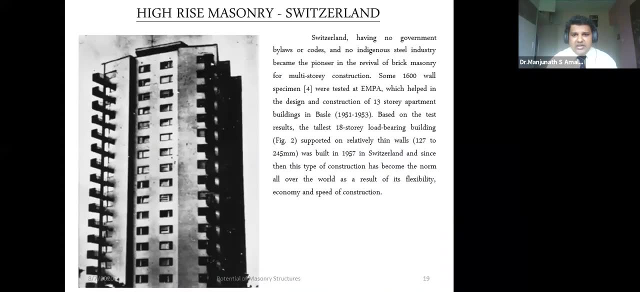 Well, this is. this was built during the The, as a as a high rise, during the early phase of high rise masonry, And subsequently we can see a lot of examples, like the one which you see here, wherein it was built in Switzerland. 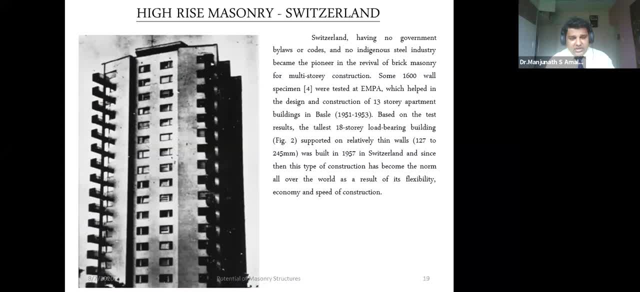 Very, very interesting note that during the 1950s, where, you know, Switzerland or even Denmark did not have a steel industry of their own, Well, had to have built, you know, let us say, 18 to 13 to 18 story buildings using, you know, the masonry. 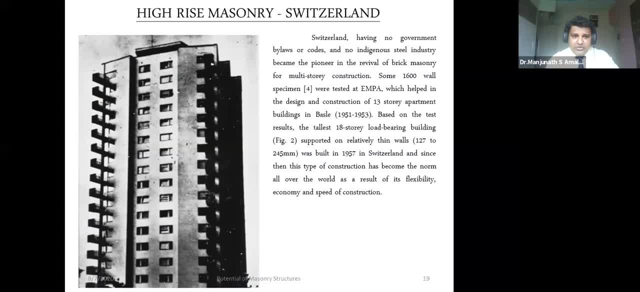 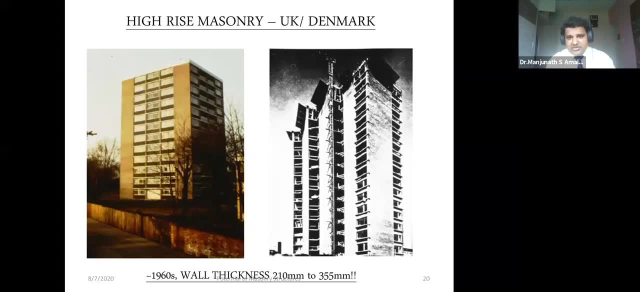 Blocks. Well, what you see here is the one which is built in Switzerland. You can see some more in Europe, That's the one on your left is the one in Britain, UK and Denmark. Well, the wall thickness is considerably low because you know the the, the achievement in the strength of the due to the better blocks manufactured. 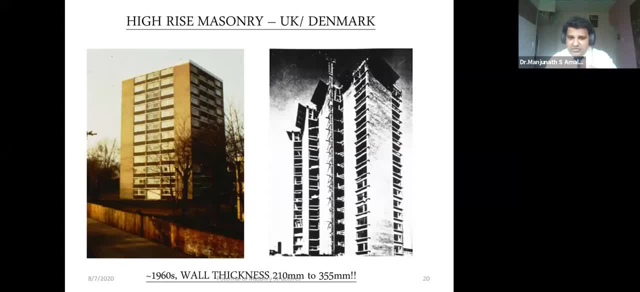 Sure One could, you know, significantly reduce upon the thickness of the Walls. The one, what you see, is built in the 1960s. Well, the thickness is ranging between 210 to 355 mm. Well, this is another, built in US. 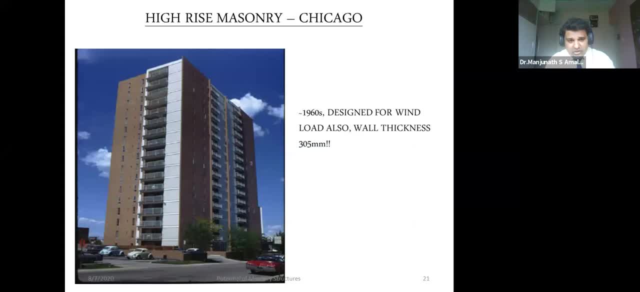 Chicago. Well, this is not only designed for the vertical loads, but it's also designed for wind load, And you know, you can imagine that. you know the thickness is just 305 mm. You can imagine what is what would be the strength of the block in order to achieve, you know, such a slender sections. 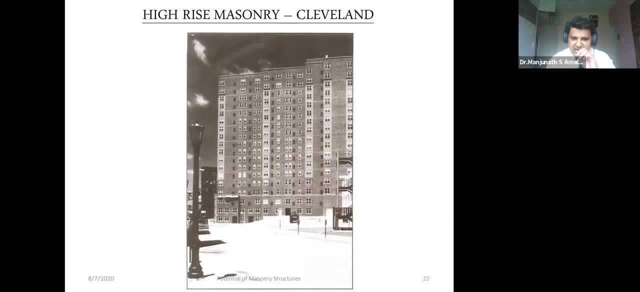 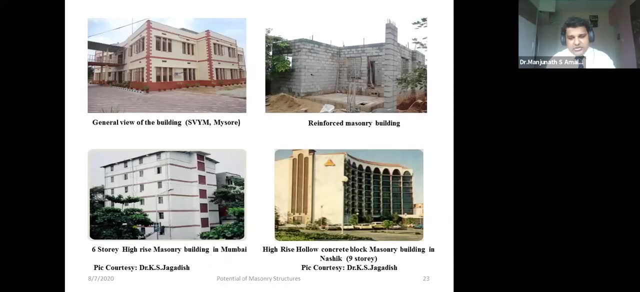 This is another example, from the US as well, Built in Cleveland, on a local front, on an Indian context. Yes, there have been buildings which have been built using, you know, hollow concrete blocks, like the one which you see here. This is a building, nine storey building, which is being built in Nashik, you know, which is a hotel building. 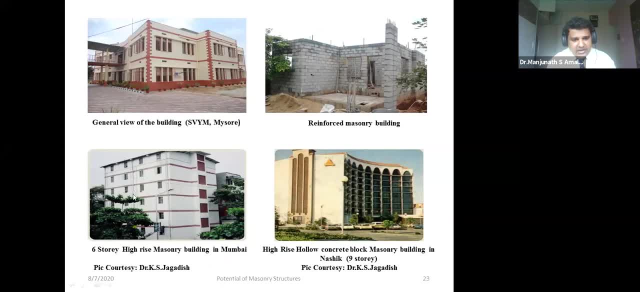 And the one on the left is a six storey high rise building built in Mumbai by the architect, Mr Ganesh Kamath, And the ones you see on a very local front, with this building very close to Bangalore and Mysore, where a two storey- you know hollow concrete block masonry building has been built. 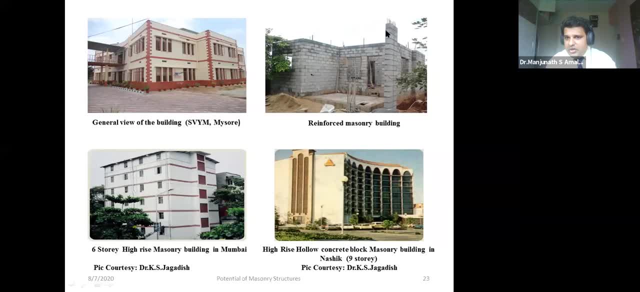 This is a residential building built in Bangalore. You can notice that, you know, because of the advantage of having larger holes in masonry, particularly hollow concrete block masonry, Well, if you want to make it good in lateral loading also, Well, one can go ahead, you know, reinforcing these masonry vertically and some, and depending on the design, you can, you know, place nominal reinforcement as per the requirement. 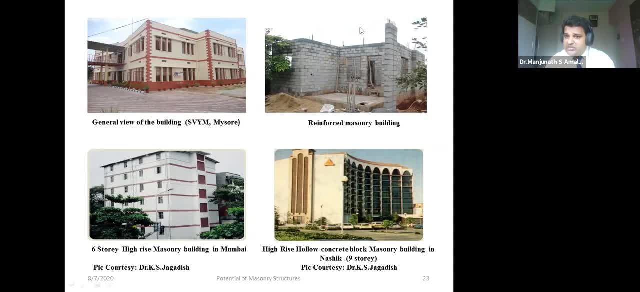 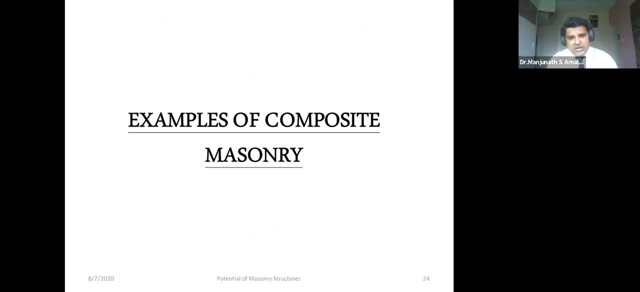 And one can go ahead with the reinforced masonry, which will not only be good in vertical loading, but also it would reasonably withstand lateral loading as well. Now, having looked into some of the examples For high rise, let us look into some where composite masonry units have been used. 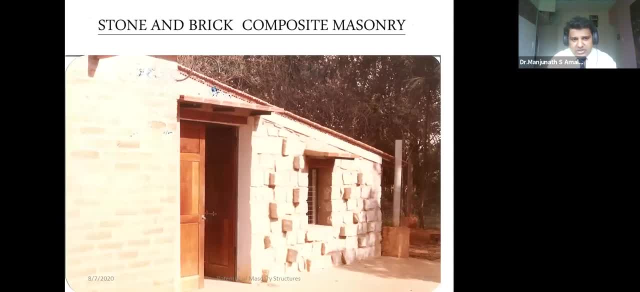 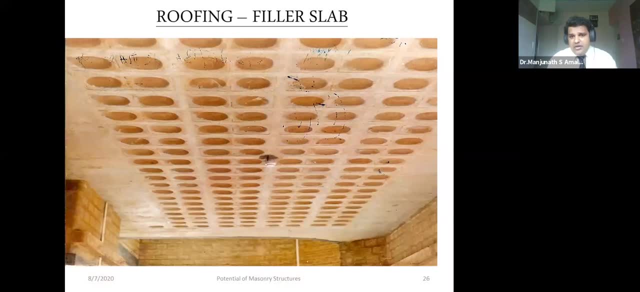 Well, the one which you see here is a composite masonry built using stone and brick, And likewise you have, you know this is very interesting- This is a filler slab. Now we have seen a lot of blocks of the masonry units which you know have been used to construct only the vertical walls. 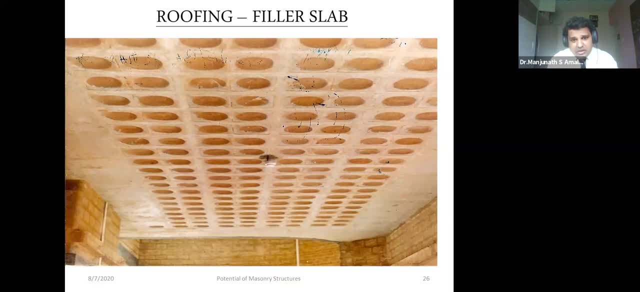 But what you see here Is a roofing which has been constructed using a stabilized mud block. The concept is very clear here. It works on this concept: Like, let us say, we have a rectangular RC slab And when it is being loaded from the top, we obviously have tension at the bottom. 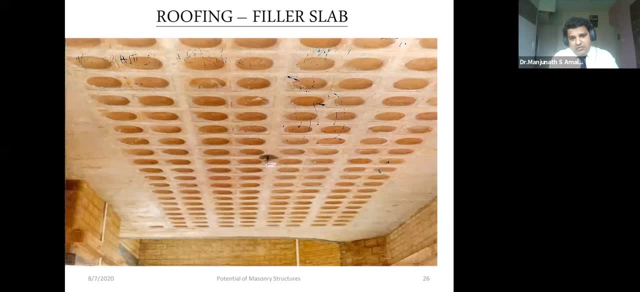 And of course, the compression at the top. Now one thing which we know about concrete is: concrete as it is is not good in, not that good in tension, although it is very good in compression. Well, if that is the, that is the behavior of concrete, then one can afford to remove the concrete. 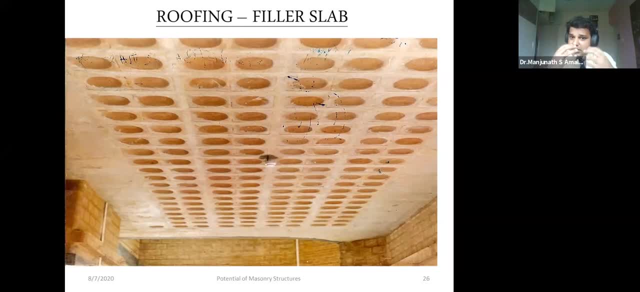 which is in the tension zone of the slab and replace it with another masonry unit. Let us say, in this case we have a stabilized block, which I had mentioned in the beginning. Well, this part of the concrete is replaced with blocks. 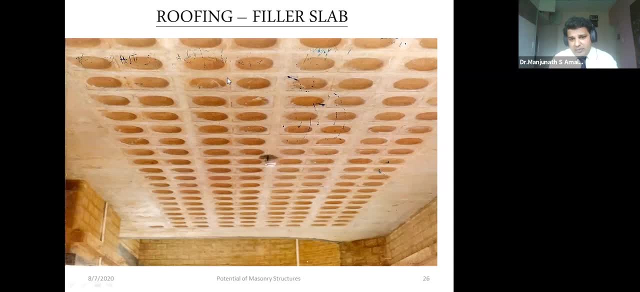 And of course you know, there would be obviously tension at the bottom. So we will leave the tension to be taken by the reinforcement which can be placed, or can be designed to be placed, in between the two rows or columns of these blocks. 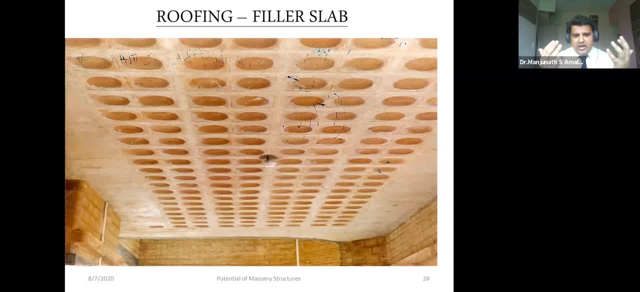 Well, you know what are the advantages? Yes, it would look. you know the temperature, you know the transfer of heat would definitely certainly be better, as we are looking and looking at a material which is an earthy material. 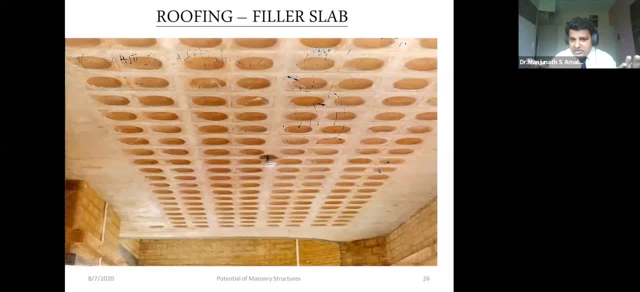 Will there be a less amount of heat transfer? Well, architecturally, aesthetically, it looks much more pleasing. And another thing: maybe if the workmanship is good and one can go ahead without even plastering the roof and maybe, you know, just finishing the slab, and it would just look very aesthetically better as well. 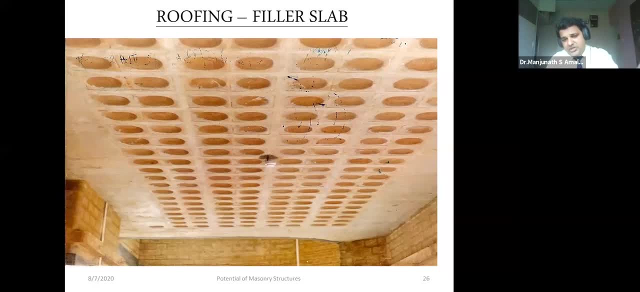 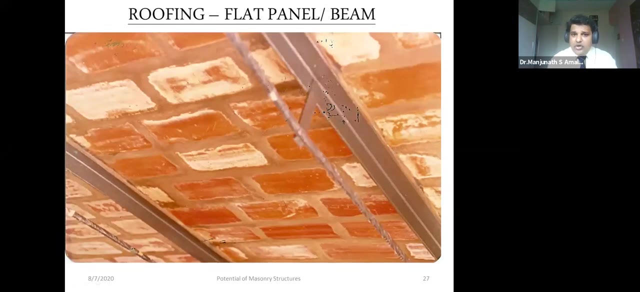 This is, this is the. you know, this is also an option where the masonry unit not only is being used for the, the walls, what you see here, but also, you see, it is being used as a roofing material also. Well, you know, you can also have what you call the flat panel. 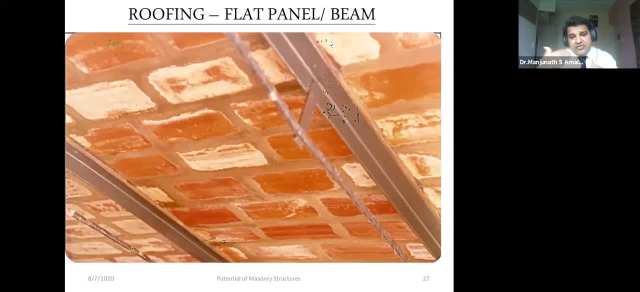 Well, the flat panel, you know, which are maybe prefabricated elsewhere, And then you know, it can be brought to the city, to the site, And then, you know, just have to place these panels as a roofing material, of course, with the beams. 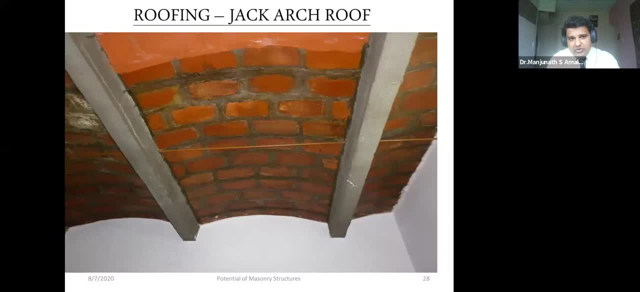 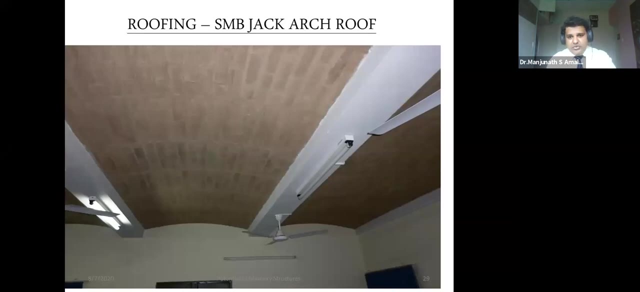 Well, if one wants to use an arch kind of roofing, you have an option of making the panels again, And one can also have a jack arch roof. This is used using masonry. and then some more examples where stabilized mud blocks have been used to have the jack arch roofing. 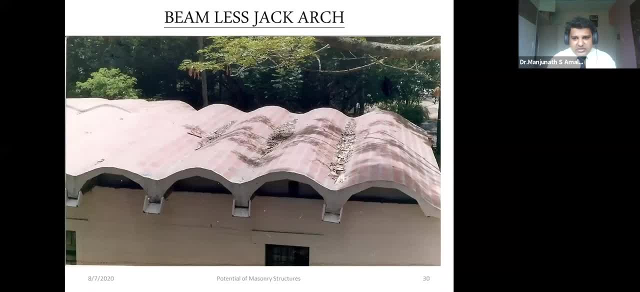 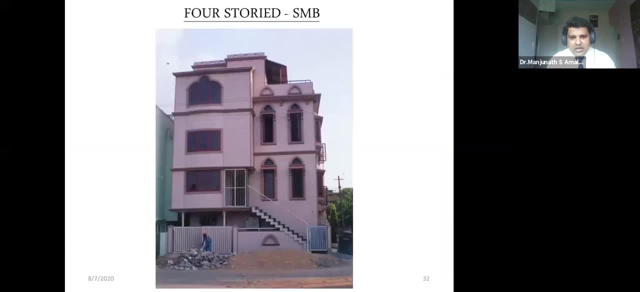 Some more examples Again. this is a beamless jack arch roof slab. And moving forward, well, talking about, you know some of some more examples with SMB. Well, this is another building in Karnataka where you know a four story stabilized mud block masonry has been built. 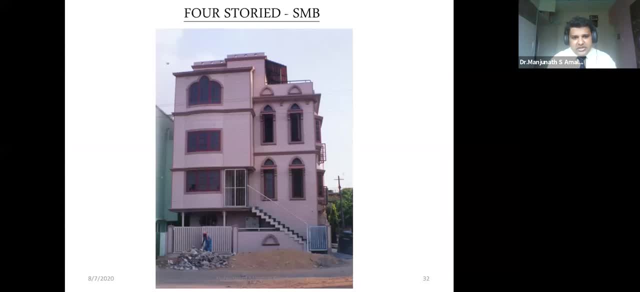 You can see that. you know it is architecturally pleasing. Well, I think you know. you can also notice that you know the plastering is avoided and making it- you know that much more You know- efficient because of the less usage and maybe you know it could be worked out to be more economical as well. 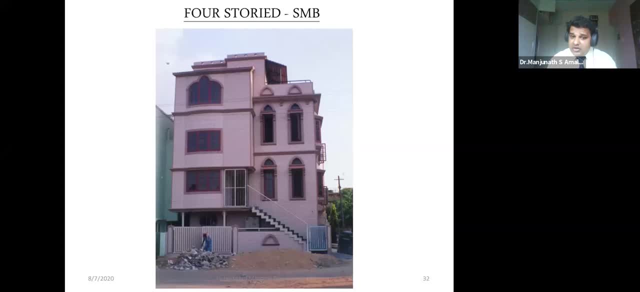 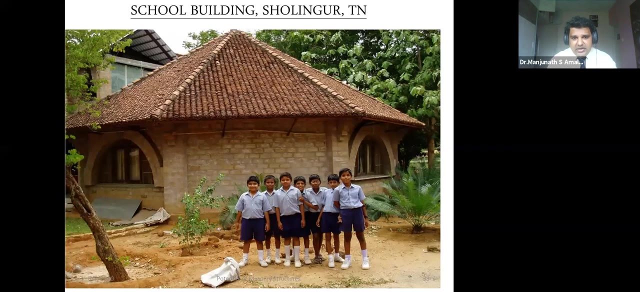 And the good part is that you know it consumes far lesser energy and lesser CO2 emission, as discussed in the previous slide, in the beginning slides. Some more examples. This is a school building, you know, in Tamil Nadu, where the stabilized mud blocks have been used. 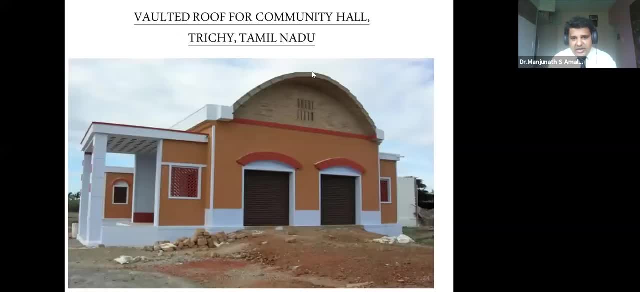 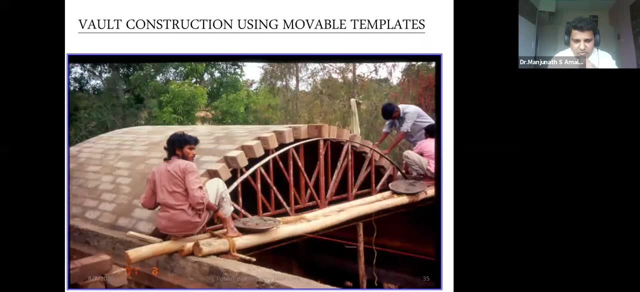 And this is a vault. This is a vault, And you know again, which is being built using the stabilized mud block. Well, if one wants to look at, you know the construction. well, it's quite simple where you have a movable template. 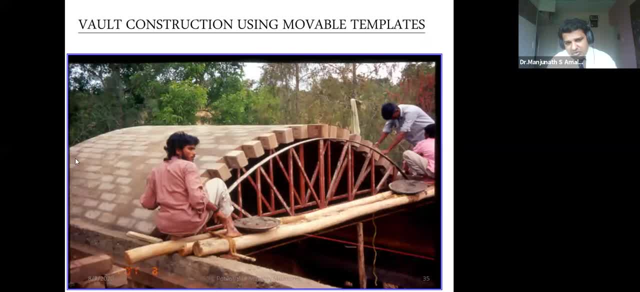 which is being traversed from one part of the slab, one part of the roof, And you just have to place the blocks over the template with proper locking, And then you know the vault, would you know, be finished. This is another example of a vault. 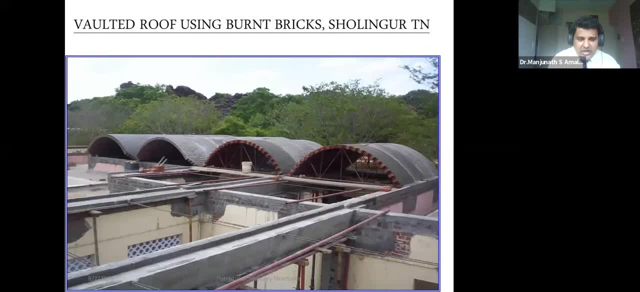 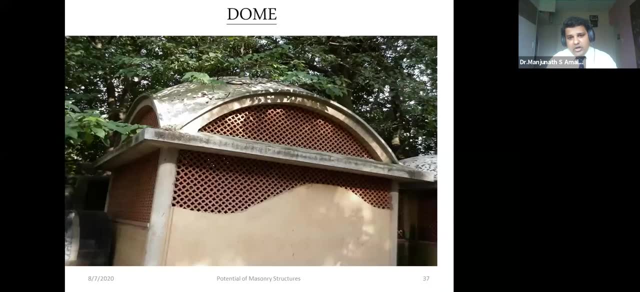 This is another example of a building in Sholingur, Tamil Nadu, where a vaulted roof has been built using the burnt bricks. Well, a dome, you know the masonry is not restricted for vertical members as walls or, you know, horizontal members as filler slabs. 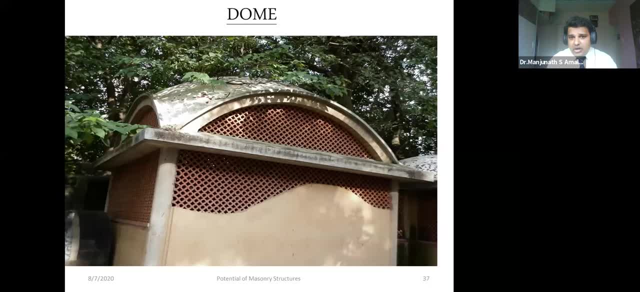 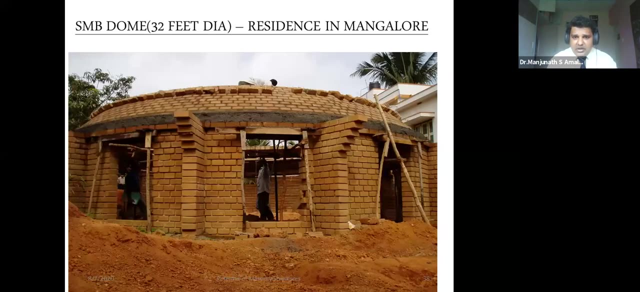 Well, you know you can, maybe you can build, you know, curved roofs as well. Well, one classical example you can think of is a dome. Now, this is another example where a dome is being constructed using the masonry. Well, this is another example where you know for a residence, a stabilized mud block dome of about 7.5 to, let us say, 8-meter dia has been constructed. 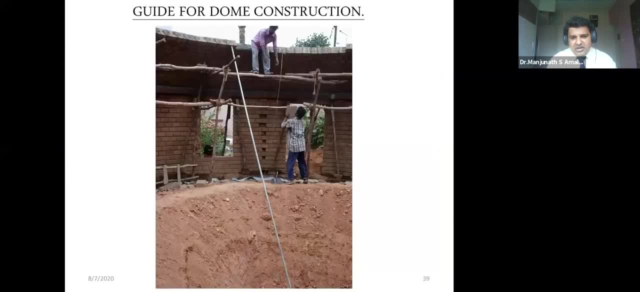 Well, even as we did mention in the beginning, well, you know, even for the construction of dome, we do not, unlike the RC structures- we do not require formwork as well. The concept, the technology does not require formwork. Well, you know, even for the construction of dome, we do not unlike the RC structures, we do not require formwork as well. This is another example where a dome, you know, works culturally. A dome's frames height is nine centimeters. 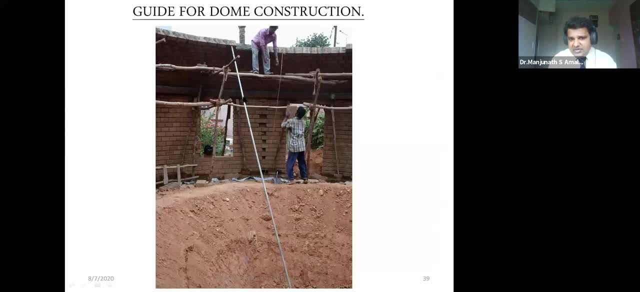 We summarize it as a model tube, Basically this structure, and then we make the slabs, the masonry. Well, this is another example where a dome is a…. This is another example where… Where a dome… lowered or it can be heightened, based on what is the rise of the dome which one wishes to. 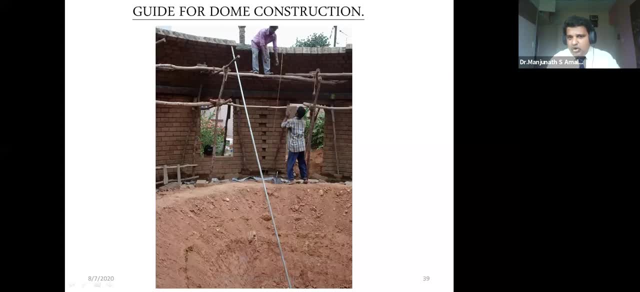 have. If you want to have a shallow dome, well, you know, you just have to, you know, lower your force upon your center point of the dome. Well, this is the finished product, finished building of the same building which I was. 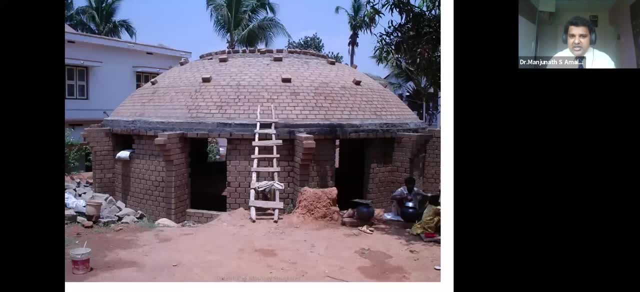 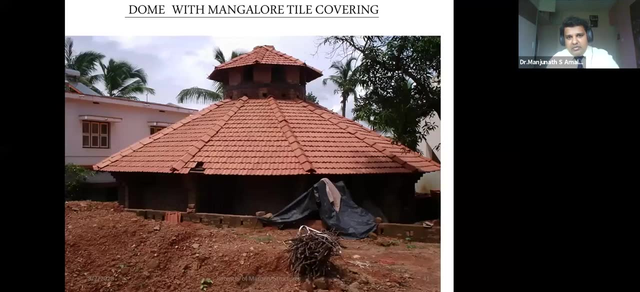 talking about. Well, if you want to cover it, if you want to have it as a curved roofing in the interior, it could be that way: an outer and an exterior. you know, if you want to have it as you know. 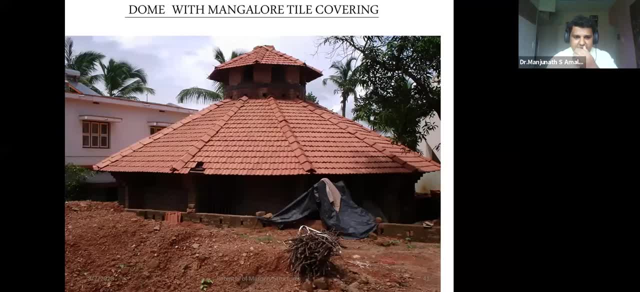 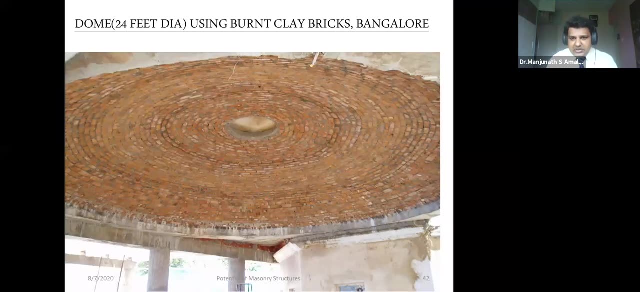 a Mangalore tile covering. one can go about doing it depending on one's requirement. Well, for the same dome, you have a Mangalore tile covering, which is being done. Well, this is another building, you know, a burnt gray bricks, again about seven meters. 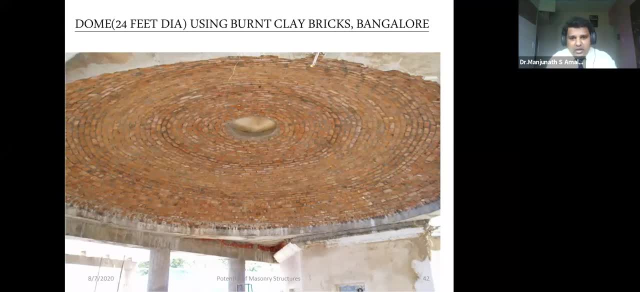 being built in Bangalore. Looking at the construction of dome, I think you know one can look at it in a different way. If you want to look at, you know constructing, let us say, a spherical dome. well, a spherical. 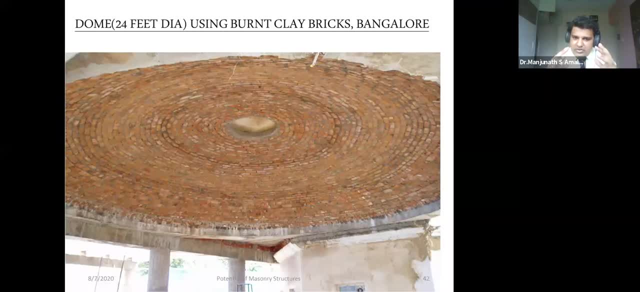 dome can best fit in a plan which is, let us say, square. Now if I want to have a curved roof, but then I do not have a plan which is in square. Now let us say if I have a rectangular plan. 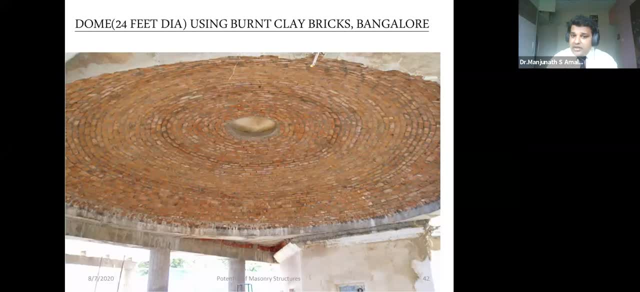 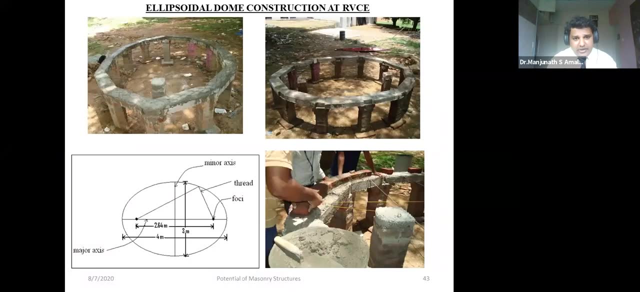 Now again, you want to go about, you know, constructing a dome. Well, for such reasons, One can Basically choose what you call as a dome in ellipsoidal shape or, if I can say, an elliptical dome. 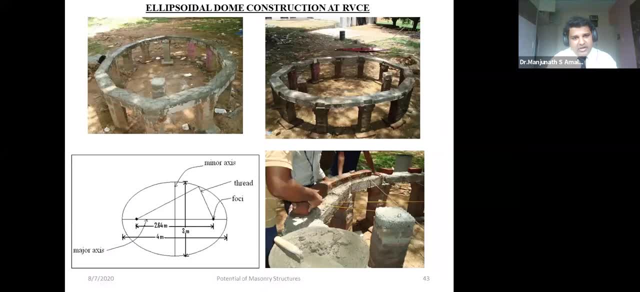 On that note, we had one project- a student who wanted to work on that in Arvi College of Engineering, Bangalore, where you know we went about, you know, attempting to construct a dome in the form of an ellipsoid. 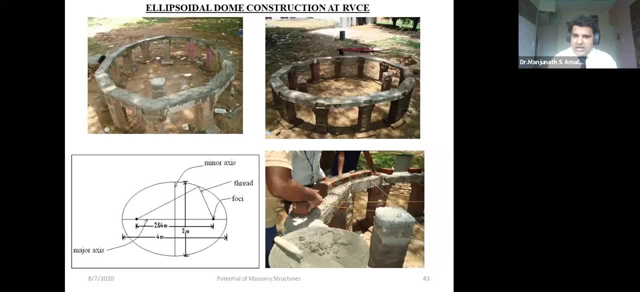 Well, the idea is quite simple. Well, you know, it is basically a prolate spheroid. It is a spheroid, It is a spheroid, It is an elliptical dome, where you know if you are looking at the plan of the plan. 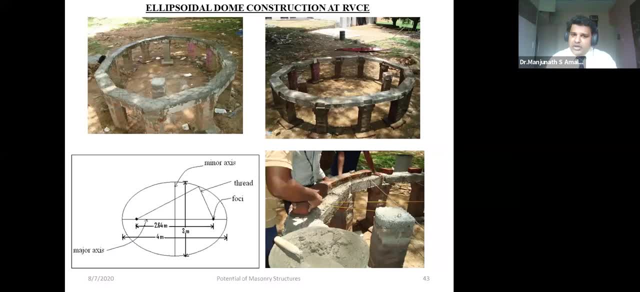 and, let us say, a section along the major axis, it would look elliptical, while if you are taking a section along the, let us say, minor axis, it would shape of a semicircular. Now, and based on the geometry, one can arrive at what you call these two points as the point. 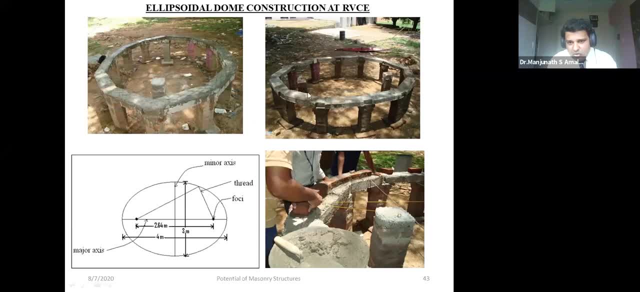 of foci And you have these points On the foci. what we did was we just, you know, erected piers here, depending on what is the span, I think we took four meters as the major span and three meters as the minor axis span. 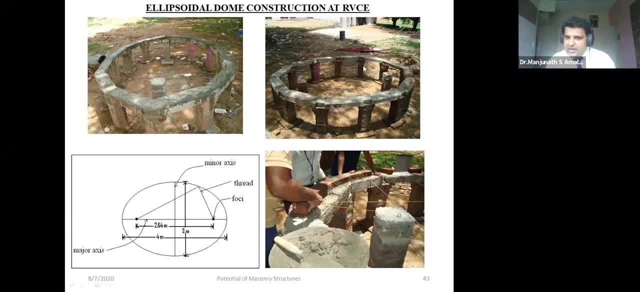 And then the distance between the two piers were all calculated And then we could have this shape as a supporting member And using the foci. what you see here, these are the two piers of foci And, having a constant distance between the two piers, we could have a supporting member. 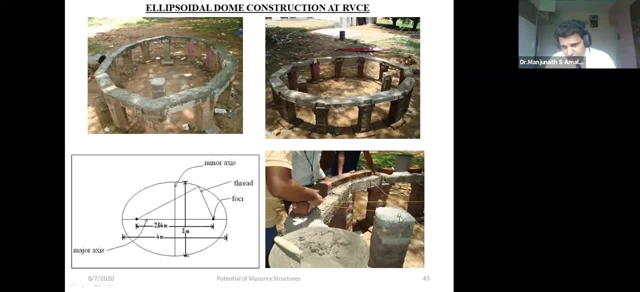 And using the foci, what you see here. these are the two piers of foci And having a constant thread. you know where one end of the thread is connected to one foci point, like what you see here, and another thread, the other end of the thread, connected 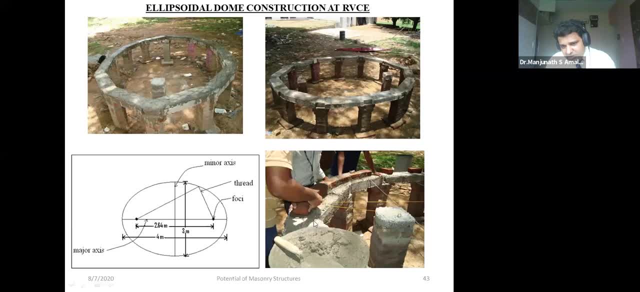 to the other point of the foci and just pulling it out and along this profile, you'll be able to trace the, you'll be able to trace the, what you call the ellipsoid in time. Now, this is what was attempted. 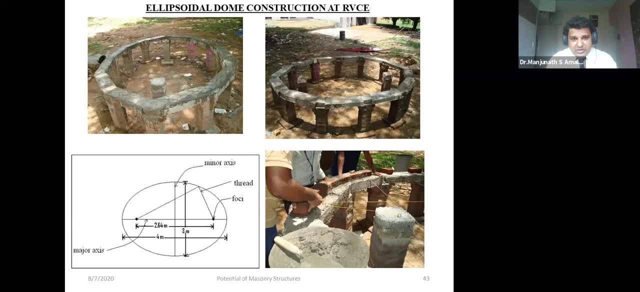 And you know, I'm happy to also say that, you know this is what we've attempted. I'm happy to also say that there is no point in trying to find that this was, you know, purely attempted by one of my student and in fact you know. 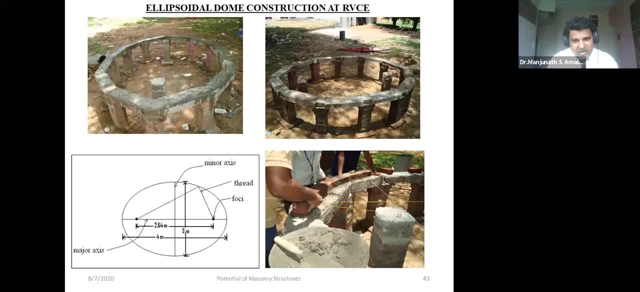 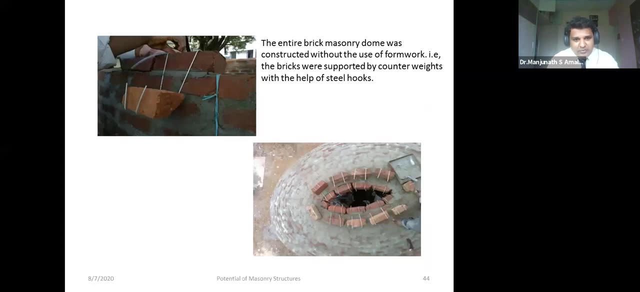 he did the construction also himself, and you know it is always, I know one would say, experiential learning is always, you know, appreciated. so on that note, he, he wanted to do it himself and that is where we, he could, you know, we could complete this doom and what you see here, well, as you are going ahead with, 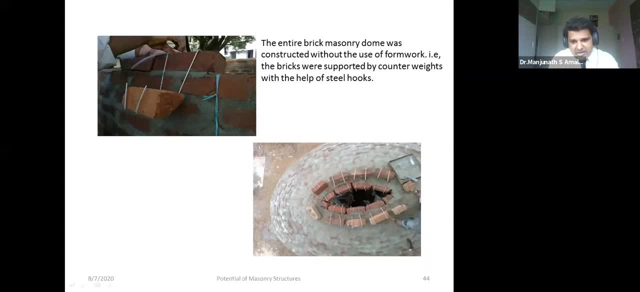 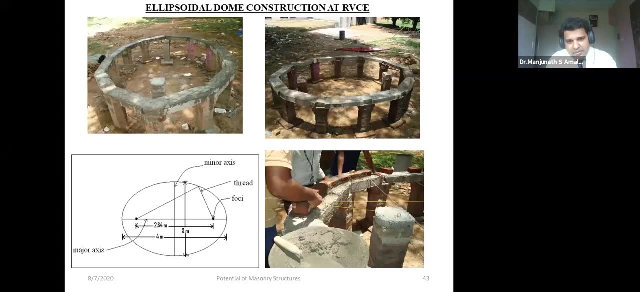 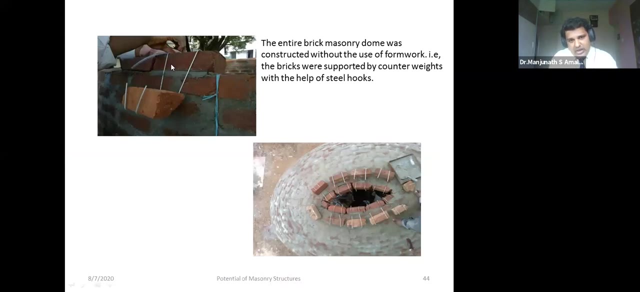 construction of doom, for you know, let us say, subsequent layers. this is the first layer. as you go, you know, above, obviously, you know you will have the curve and you know, as you are going inwards, you know the blocks which you are trying to place here have to be supported. now, you know, in order to 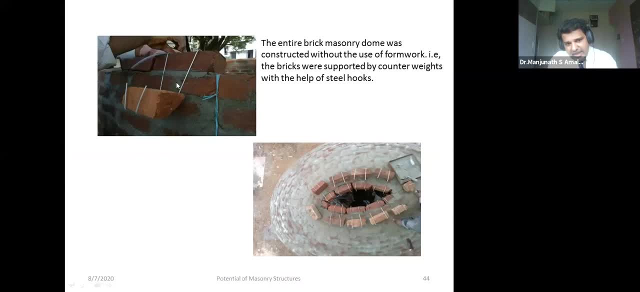 support that we have the steel hooks which are, you know, in s-in shape. now, these s-shaped hooks. you know what it would do is it would counterweight the goal of the construction of doom, and you can see that. you can see that the blocks which are in position with another brick here. so why does this? 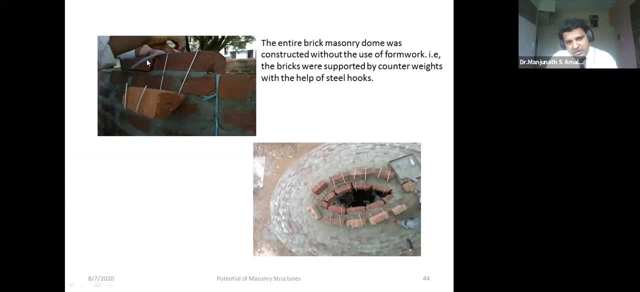 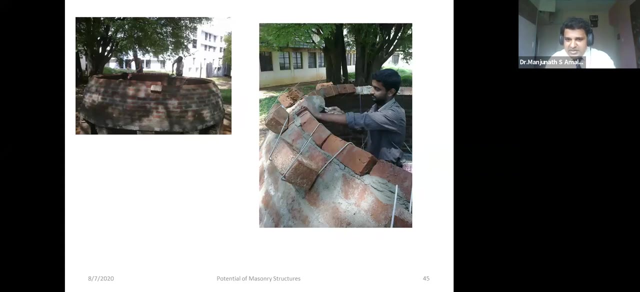 construction goes for one you know, perimeter, well, the blocks would have, you know, sufficiently set well number of layers. we, he went about doing it and well, these are the the various stages of his construction. he's the student who has done this and the counterweights. here you can, you can see the 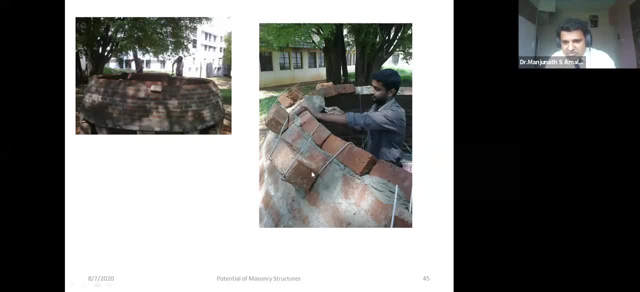 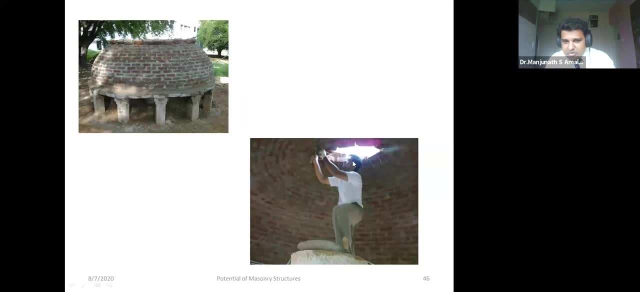 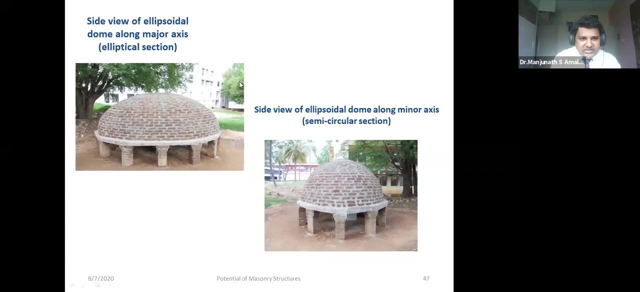 counterweights here which are, you know, trying to contract the weight of the blocks which are just placed on top of each other. and you can see that the blocks are just placed on top of each other, and you can see that the wall, you know, by that I mean the wall- is in position. well, the product, you know. 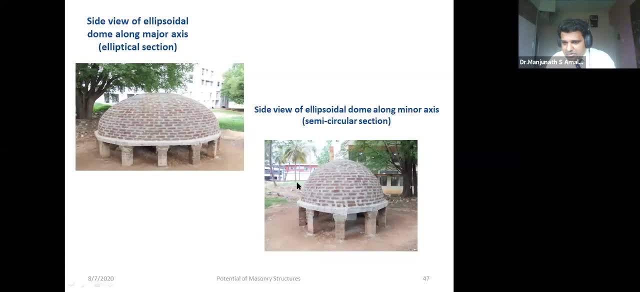 you can imagine. well, this is the interior of the doom and this one could imagine. this is the final product, what we had, as I said. well, along the major axis it is a elliptical in shape. while you are looking to take a section along the minor axis, it would be a shape of a semicircle. now, if you want to, 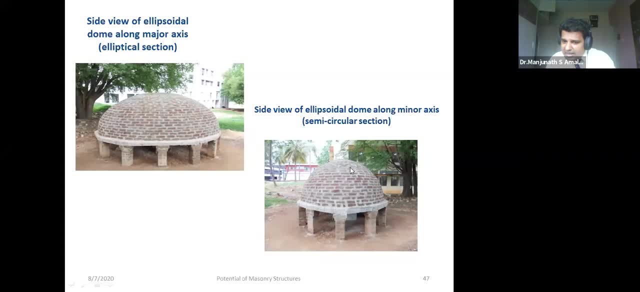 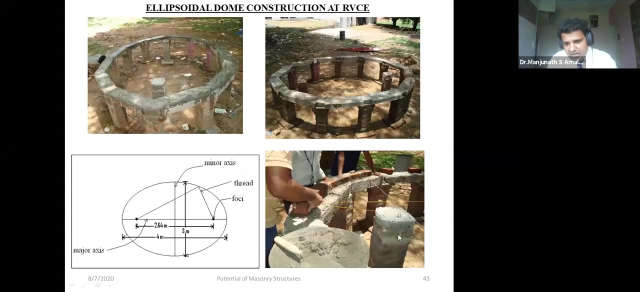 you know, maybe not have it as a dome of such big rise. one can make a shallow domes by just lowering the position of the foci. So if you just play around with the position of foci, what I'm trying to say, one you and of course you know. coming back with the distance, 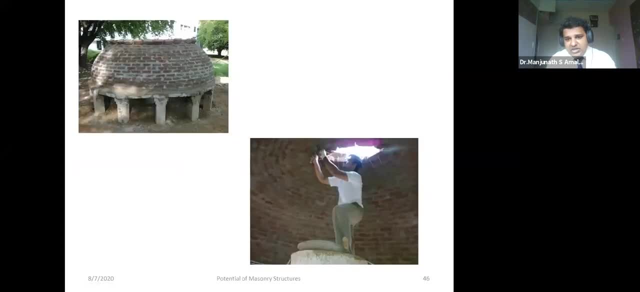 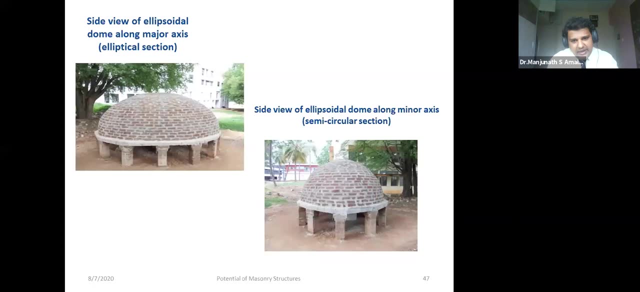 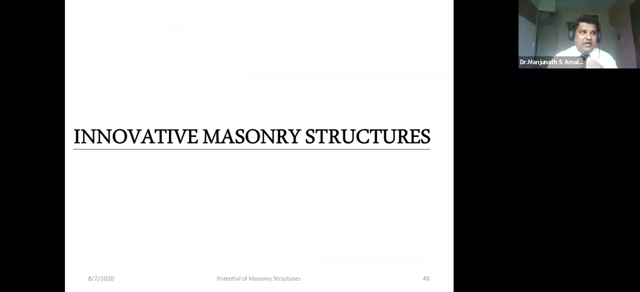 of the foci, one can, you know, construct a domes of shallow depth as well. Now, talking about the innovation, well, you know, I think you know it is not complete unless we talk about the way the famous architects who were behind you know constructing some of 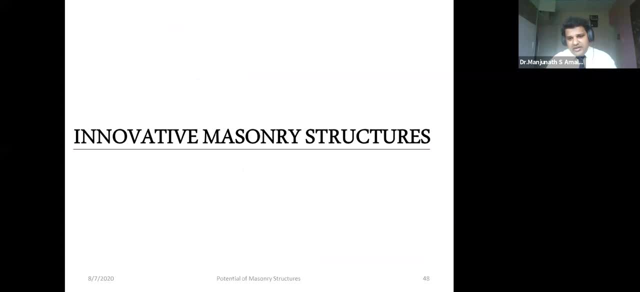 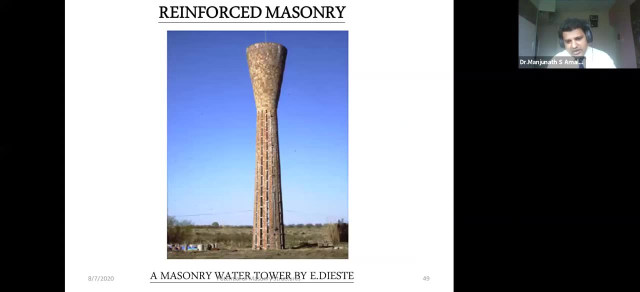 the, you know, famous structures, if I can say that. well, one cannot forget an architect, Leonardo Dias, who was an Uruguayan architect. well, during his tenure, that's during some time in the mid 20th century, he has come up with wonderful structures, you know, very innovative. 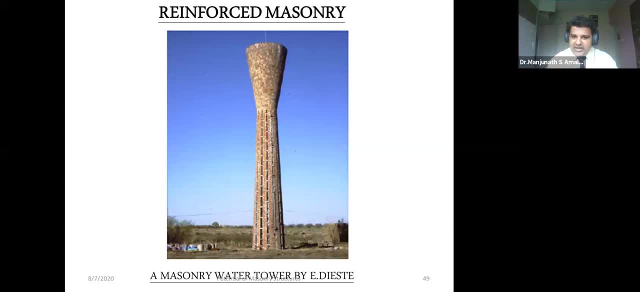 where one which you see here is actually a masonry water tank. of course it is reinforced. Well, we have seen reinforced concrete structures and its structure, but you know, masonry is also not far behind when you are looking at. you know, you know, you know, masonry is also not far behind. 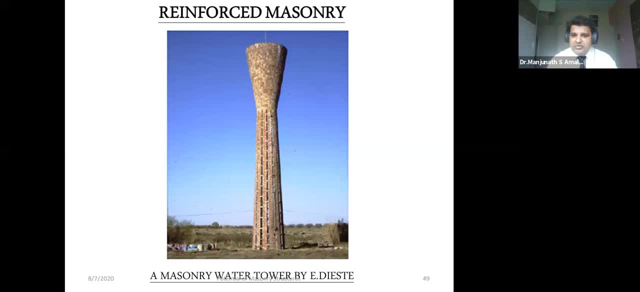 when you are looking at you know masonry is also not far behind. when you are looking at, you know proper design and proper placement of reinforcement one can achieve wonderful structures like what you see. here is a masonry water tank which was built in the mid 20th. 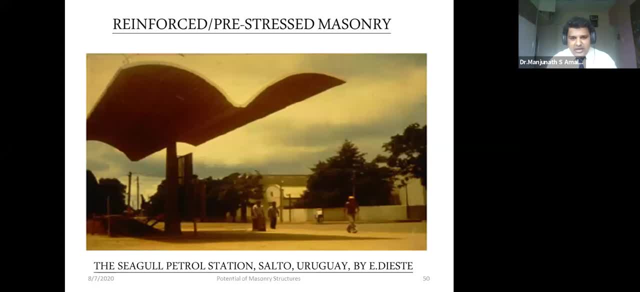 century, During the same time, the same. you know designer, you know you could. you could see this. you know cantilevered petrol station. you know what you can say: a cover where you can imagine what is the kind of cantilever it has. Well, you can say that. 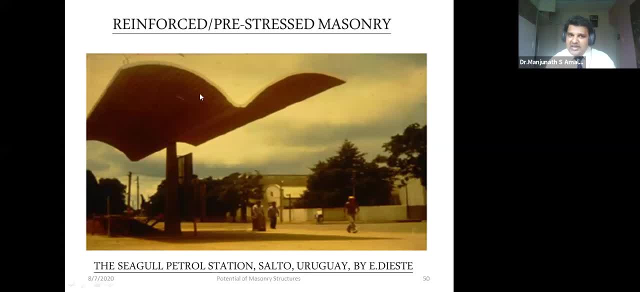 you know, the technology used was. it was again a combination of reinforced and pre-stressed. we have seen, you know, pre-stressed concepts being, you know, used very extensively nowadays for concrete structures. but, you know, masonry also can be pre-stressed and such structures are. 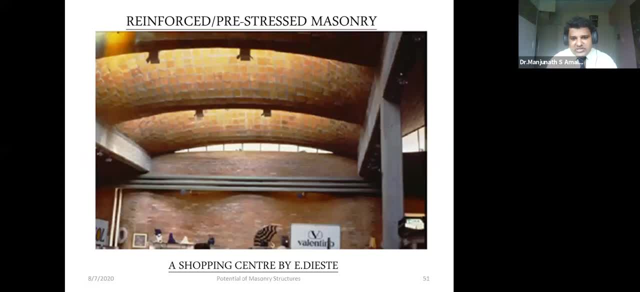 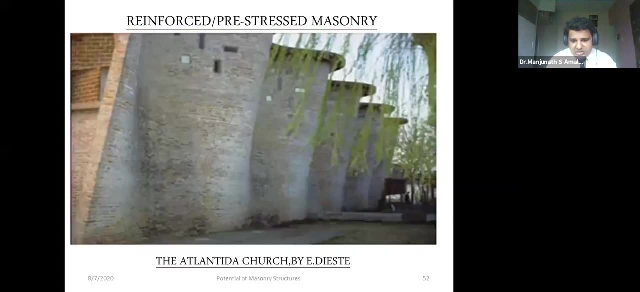 quite possible. These are some more examples of the same designer. Well, this is a shopping center at Uruguay. This is a church you know. again in in in Uruguay. Well, you know, if you just key in the name of this designer, I'm sure you can see a lot of examples which are of great interest. 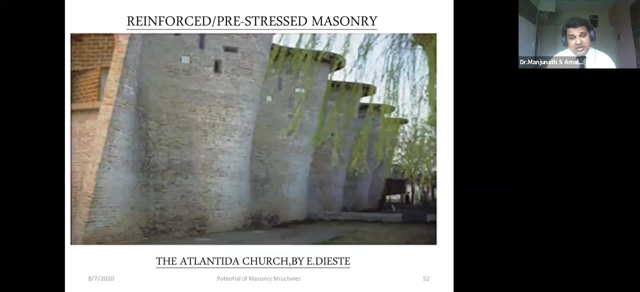 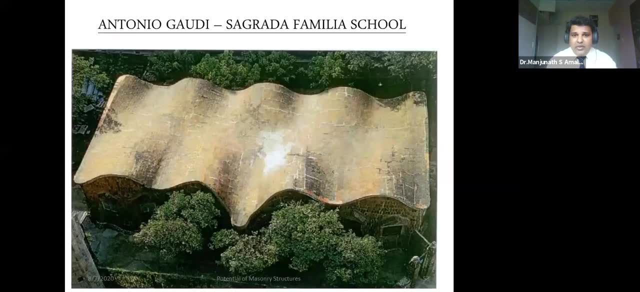 you know from, for a structural engineer, and one can appreciate such structures being, you know being constructed, you know, with masonry. Well, how can one also forget, you know forget, Antoni Gaudi? Well, you know some of the structures which was constructed. 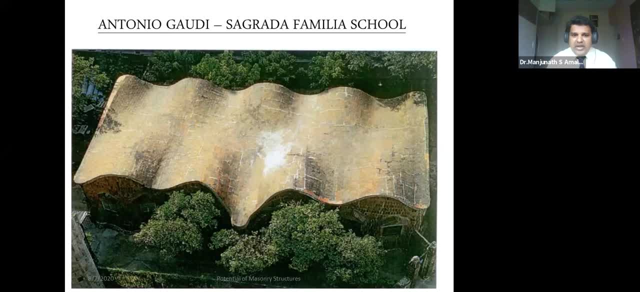 are, you can say, a late 19th century. We have such fascinating structures which which have been designed by this famous, you know, architect. He was a Spanish architect during the same that period. Well, this is what you have, you know: a school building. 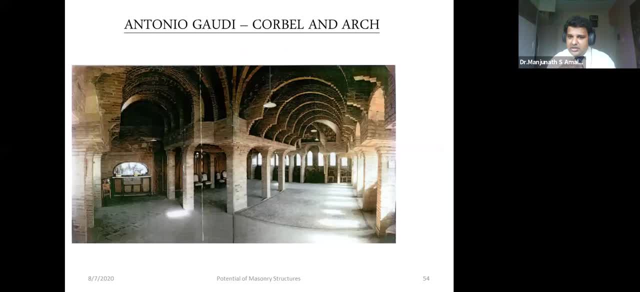 and you know it's not restricted to being only used as vertical, horizontal. Well, you can construct, you know. you know carpels say arches. you know using the using, you know masonry. 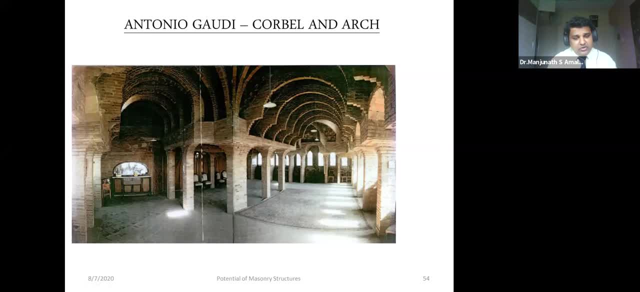 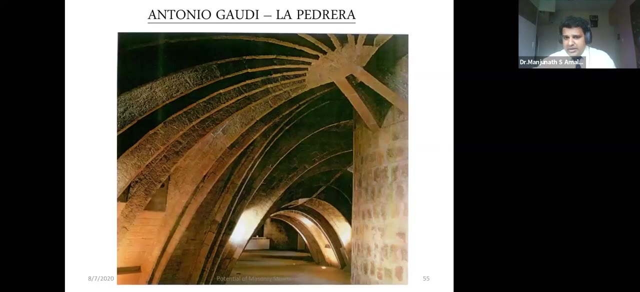 Well, all these pictures talk, talk to itself, talk by itself, the potential of masonry structures. And remember, these were built, you know, maybe more than a century old, maybe 1 150 years old, and this is a building in um, in barcelona, which is, uh, called as the lapid. 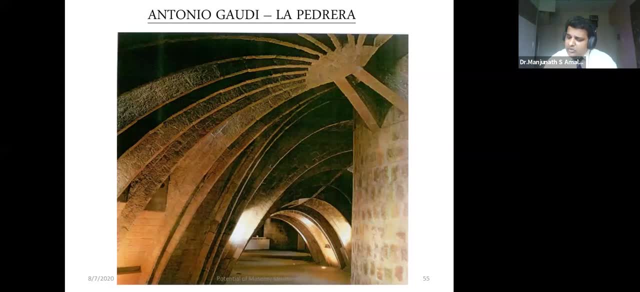 it's also commonly called as, uh, you know, casamilla, and well, this, this, this was purely built using limestone blocks, maybe during 1906 to 1912, and it sometimes also referred to as stone query. and now, now, this has all become heritage, heritage structures. you know where it has become a? 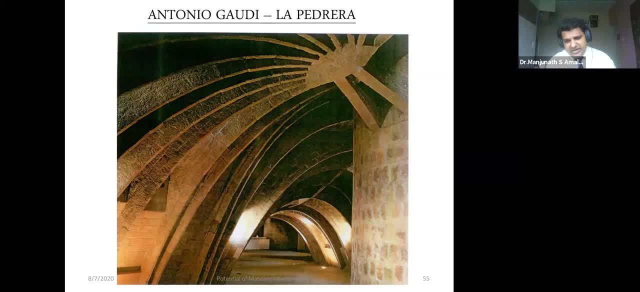 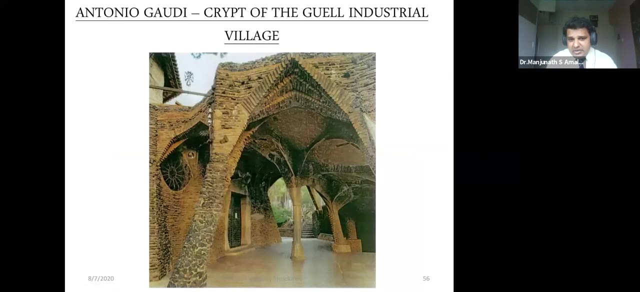 tourist place which also hosts a lot of, you know, commercial, social and cultural activities. you can see that you know it is neither it is. it is, you know, a curved kind of a you know construction which has been made. well, this is a very classical example. this, this was. 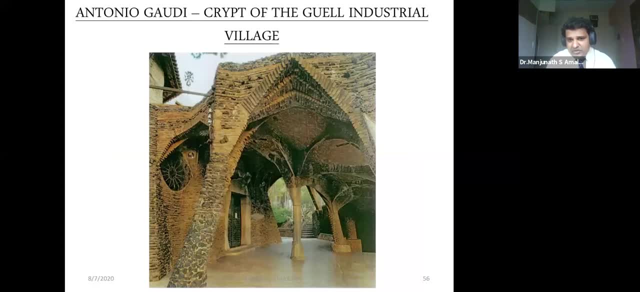 this project was the last uncompleted work of antonio gadi. well, however, this part of the uh, you know the crypt, uh, uh was actually could have, could they could complete it. you can see that there are, these are all inclined in plan. uh, you can, you can, one can imagine, uh, the kind of 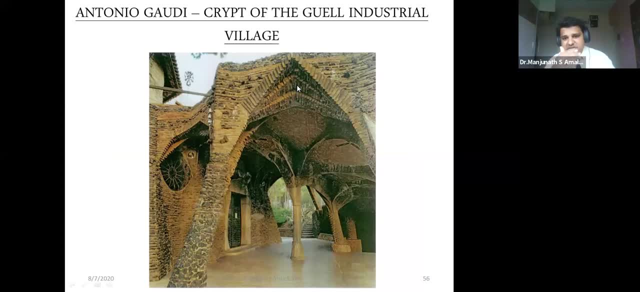 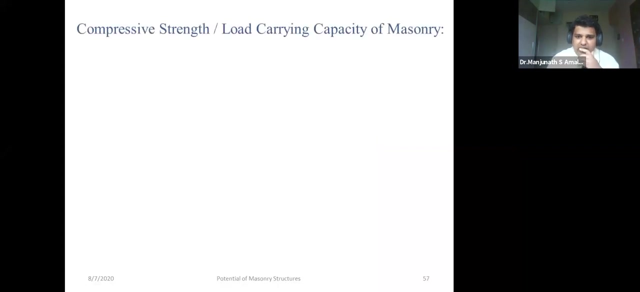 technology, the kind of uh design which is being behind to get such fascinating structures, although the original uh the building was to be a church, but later it was converted to be a crypt- in in this place, where, which is about uh 23 kilometers down south of uh barcelona. well, these are some of the structures, i'm sure. 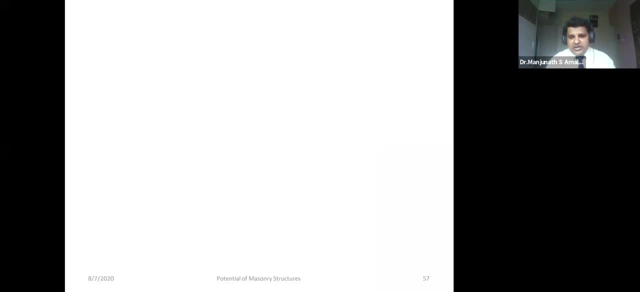 you know, if you just keen, uh, these are like, likewise, many such uh, architects or designers who have, uh, you know, very innovative structures which have been built using the concepts of masonry structure. that this, now, this comes, these points, i think you know we could, uh, you know. 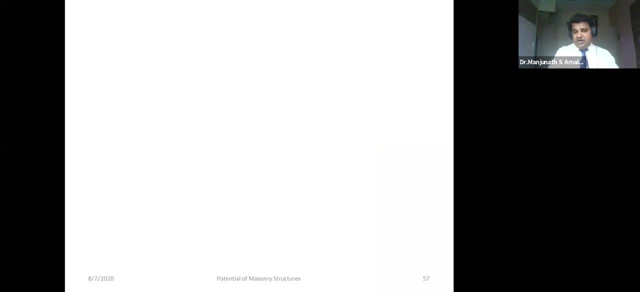 appreciate, or we could see that you know, what is the potential of masonry structures. you know uh well, in terms of structural as well as in terms of architectural. now, uh, you know, uh, i would a little extend on my presentation, uh, in order to look at, uh, how do we go about assessing this? uh, basically, strength, uh, you know. 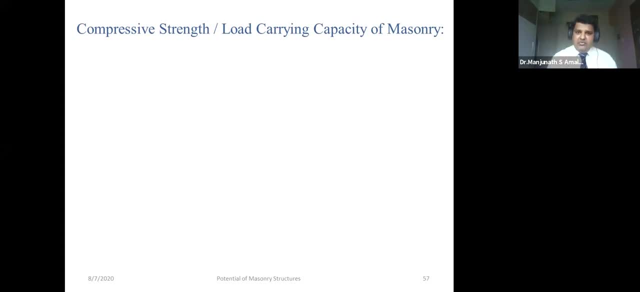 what are the, what are the ways in which i have, i can find out the uh, strength, uh, and adding to that, i will try to you know, uh, you know, maybe, in a nutshell, try to also explain very briefly what are the guidelines as per 1905 and, uh, how do we go about with the design of a masonry structure? now, if i have to, 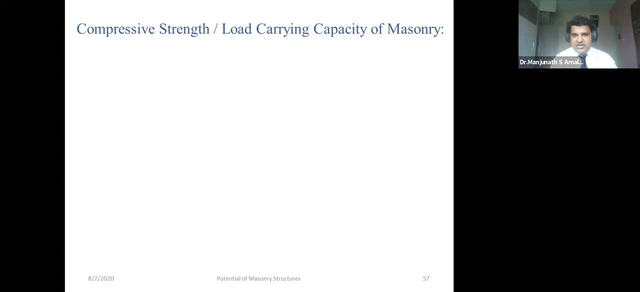 let us say, assess the load carrying capacity of the masonry structures. well, uh, you know there are three possible ways. uh, well, it is. first, it would be to test the masonry costumes. when i say masonry costumes, it would be testing the masonry units and, of course, the one which is binding them. that is the matter. secondly, now you one could you know? 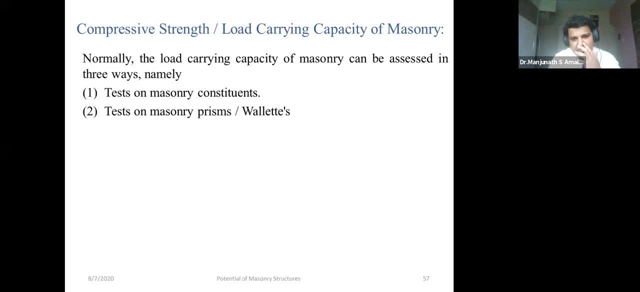 test the masonry prisms or wallets. what are prisons and wallets? we will discuss a little later. and the third option, which, which is the most preferred one, if one can afford it, if one has the facility, well, uh, the best way to do it, or test our masonry capacity, is to do a full scale. 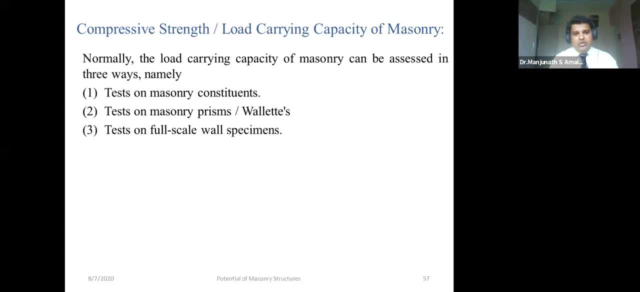 wall specimen. now, when i say full scale wall specimen, what i mean is a story height wall which can be tested, store a height. let us say, if i'm looking at a conventional residential building, i would look at a height of, let us say, three meter. well, if i can have, if i, if i can, you know, have the 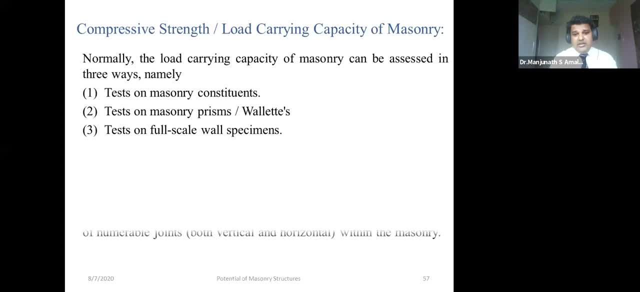 facility to test a full scale walls. well, that that would be the best option, because it will give you a more realistic- uh what i can say, uh, understanding of the performance of masonry, because it takes a lot of factors into consideration, consideration which we will discuss, and not only that, very 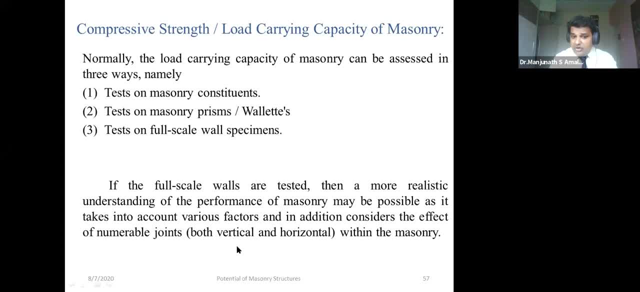 importantly, it takes the uh, uh, the uh, the effect of uh joints, because you know uh any, any structure, you know especially masonry structures. it is the joints which you know, which uh, which also decide upon the load carrying capacity: uh joints and the number of joints, uh, which decides upon the load carrying. 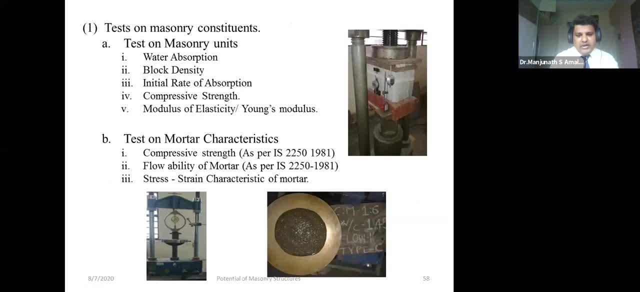 capacity of the masonry. now, how do we go about it? let us go in one by one. now, if you have to test the masonry constituents, yes, of course you know i'll have to test the masonry units. well, what are the tests? one: one have to do the 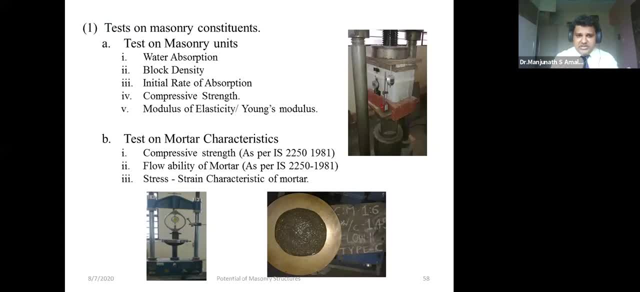 uh, the uh. what do you? what do you say? uh, the physical tests and, of course, the structural uh properties. now, what are the uh tests one can do? for physical, of course, you know, one has to know what is the water absorption of the block, what is the density of the block, what is the rate? 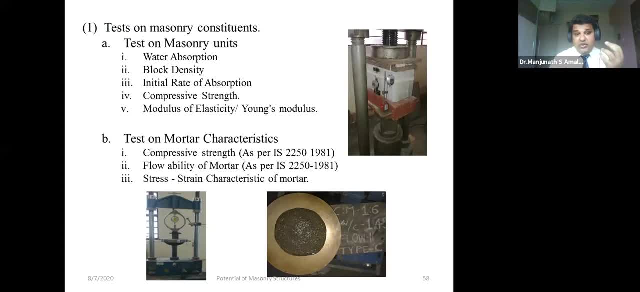 initial rate of absorption, uh, well, and also structurally, one has to know what is the strength of the block. okay and uh, and apart from that, we go about looking at the characteristics of masonry units. Secondly, we'll also have to test upon the motor characteristics. 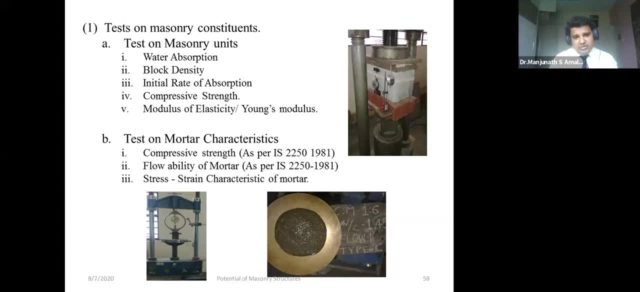 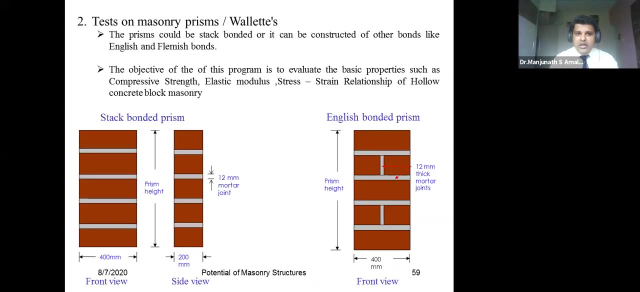 Now, because this is the one which tries to block units. now again: compressive strength, flowability, stress-strain characteristics. these are some of the tests which one has to perform when we talk about the motor. The second option, of course, is to test the prisms. 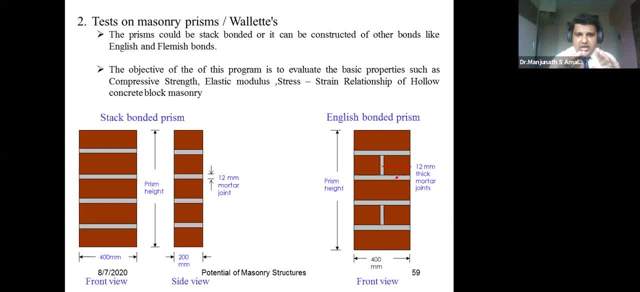 Now, what are prisms? To understand prisms, prisms are basically, I can say, short walls. short walls of certain H by T ratio, where the H by T does not exceed, let us say, 6.. Well, these are the elements which 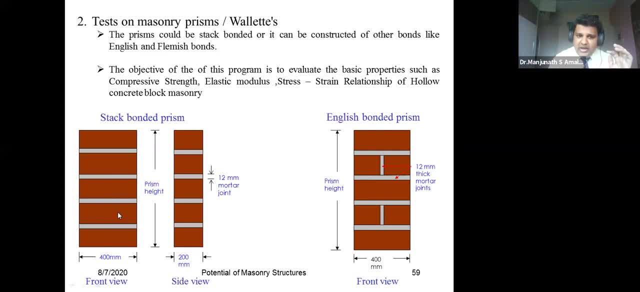 have been constructed, keeping the blocks one over the other like a stacked bonded prism, with, of course, the joints And then the other option. if you also want to take the vertical joint also into account, well then you can also have it as an English-bonded prism. 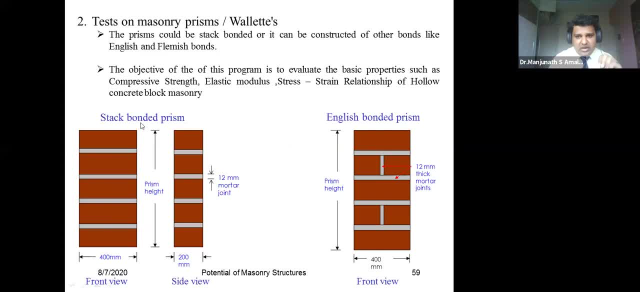 And the objective is to again test for its basic properties: compressive strength and, of course, the stress-strain characteristic of the blocks. Although this could be the general kind of test for any unit, I would try to do it. 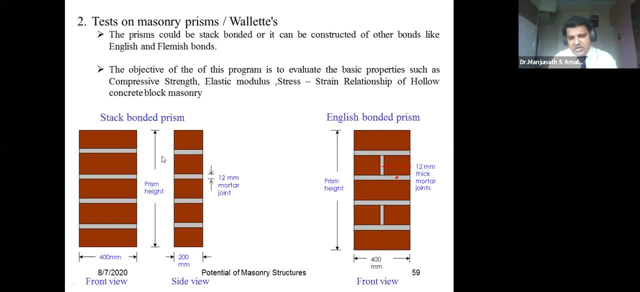 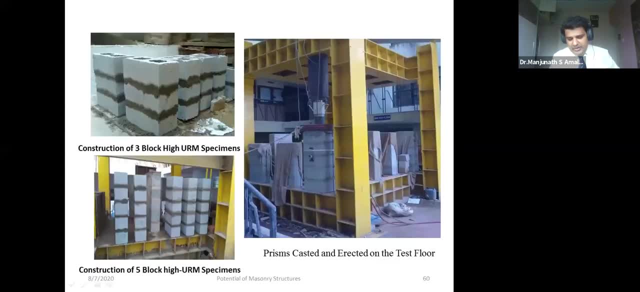 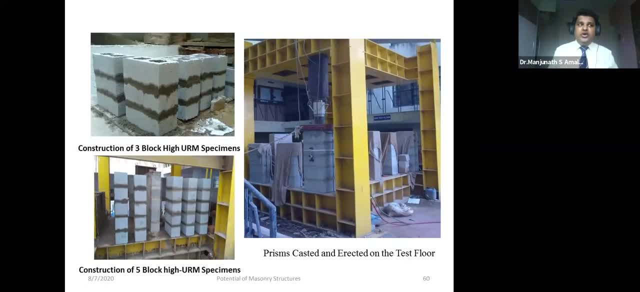 As I told, the prism is restricted. If you have to call it as a prism, well you know you can go up to H by T of, let us say, 6, slenderness ratio. Well, typically you can have it as 3-block. 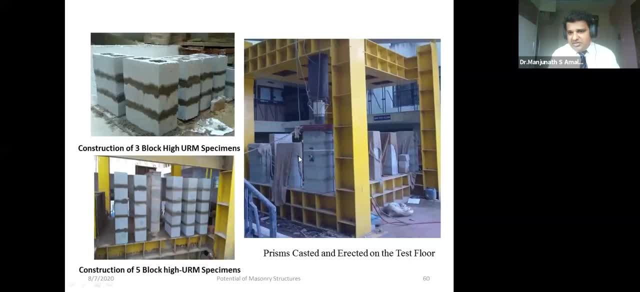 You can have it as 5-block prism, And well, we were fortunate to have at RV College of Engineering. We call this as a test floor. Well, this is a facility which maybe can be used for testing any structural element: a beta slab column, anything. 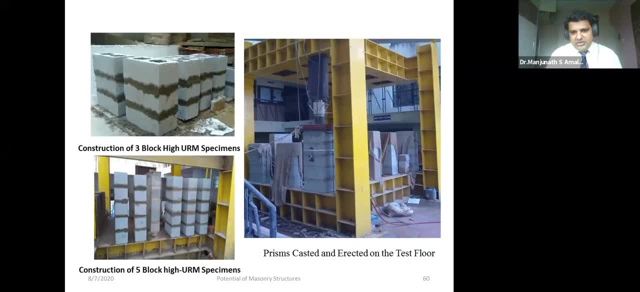 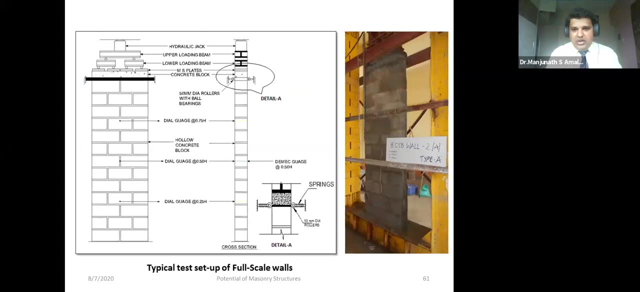 The capacity was something like 2,000 kilonewtons, 200 tons. Well, we could use this facility to test the prisms for its compressive strength and other properties. Well, the other. we were fortunate to have a hundred project from VTU. 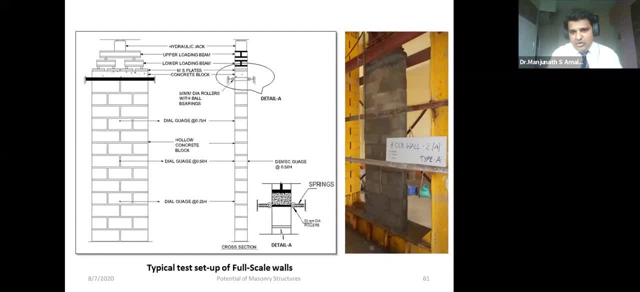 where we could erect a closed frame, a closed frame exclusively for testing the tall walls. Well, this is a wall which we have tested, which is a wall of height three meters, And well, it requires a certain amount of arrangement which has to be done. 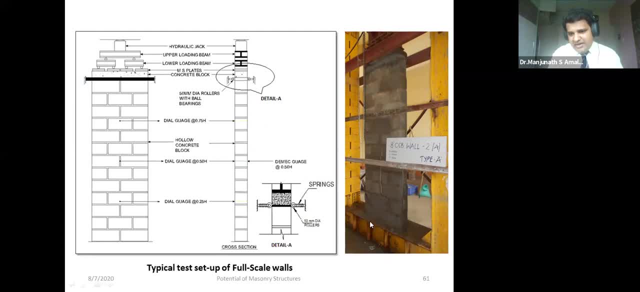 Well, in order to look at the boundary conditions, it's assumed to be laterally, and rotational restraint at the bottom. Well, in order to have it only laterally restrained at the top, well, we have an arrangement with a spring and a roller. 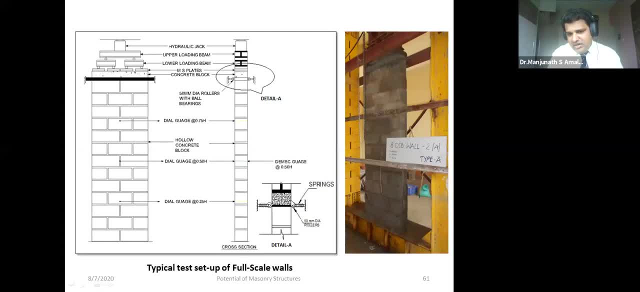 which will make sure that you have a lateral restraint, whereas there's no rotational restraint at the top. And in order to make sure that the loading is uniform, what we did was we had a staircase system of loading, where the load through a closed frame. 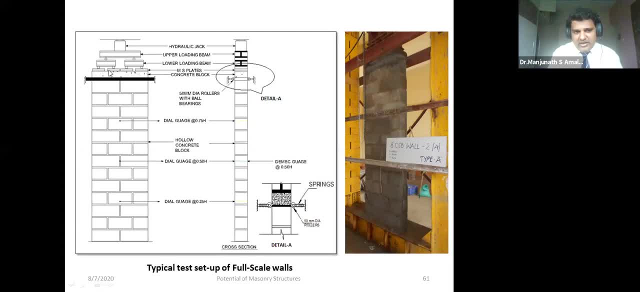 was transferred to two different tires of loading, And so this is a load that was transferred to the main assembly unit as a uniformly distributed load. Well, because of one tough time perhaps, I'm afraid we will not be able to share the results of this. 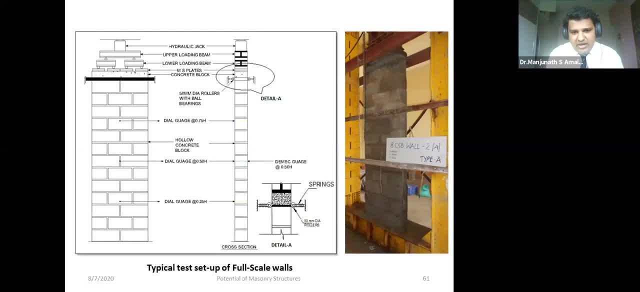 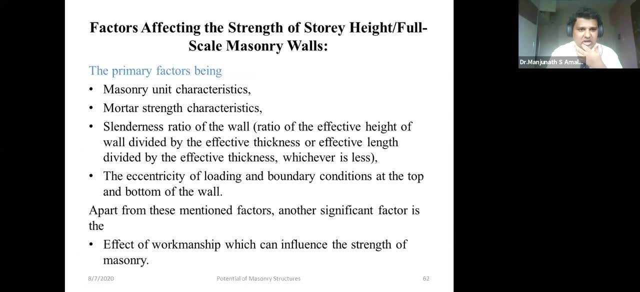 but certainly about the prisms, we would like to definitely look into some of the values. And now, these are some of the factors which I did mention. if you are trying to test the full scale walls, well, of course, the masonry units. 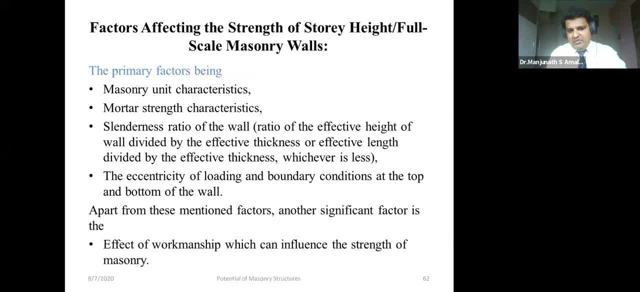 the water strength characteristics. Well, of course, you know the masonry units. the water strength characteristics are the primary factors, for sure, And apart from that, the slenderness and also the eccentricity of loading play a very important role. 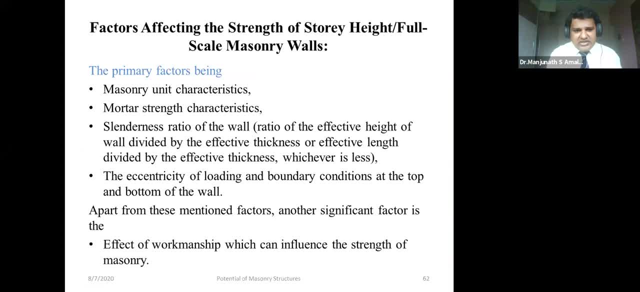 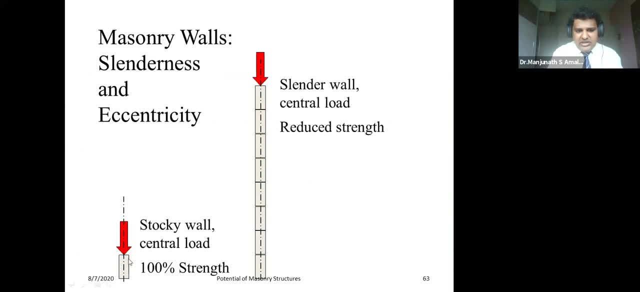 Now, what is eccentricity and slenderness? Now let us understand it with this sketch here. Now let us say, if I have a single block which I'm trying to test it for a concentric- when I say concentric, you know it's a central load- 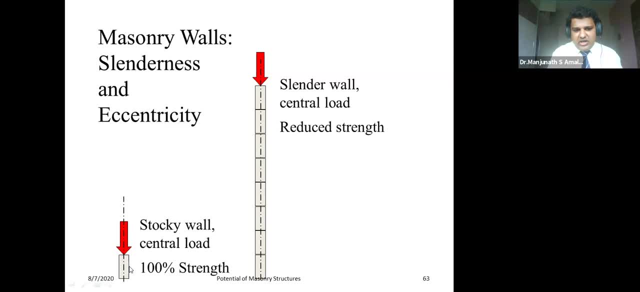 then obviously I would get 100% strength of that particular unit. But if I just place these units one above the other, making it a little more, you know what you can say: increasing its slenderness, in other words, increasing the hex by D ratio. 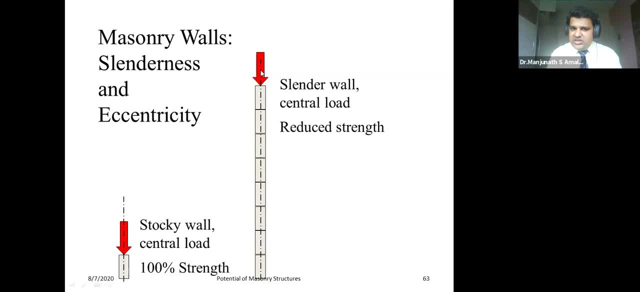 And again, let us say I'm trying to apply a concentric load. Well, you would definitely, because you know, because as the height increases- it's a general phenomenon, one would you know definitely expect a reduced strength. 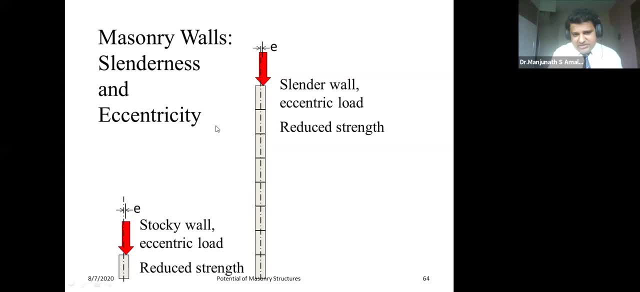 Similarly, if I'm talking about eccentrics- eccentric- what does eccentricity mean? What does eccentricity mean? Well, the loads are not acting at its CG. It is being placed at a certain distance away, which can be expected, you know, in a structure. 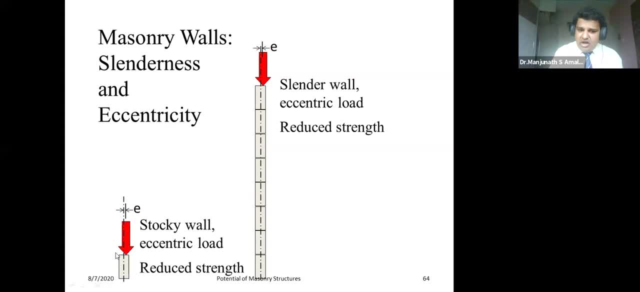 any structure for that matter. Now, if that is the case, even though it's a small unit, but if the loads are not concentric but eccentric, then again you know, there is a reduction in the strength. And if you have the same load, same load. 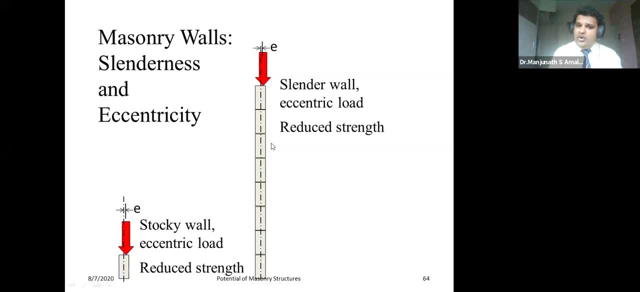 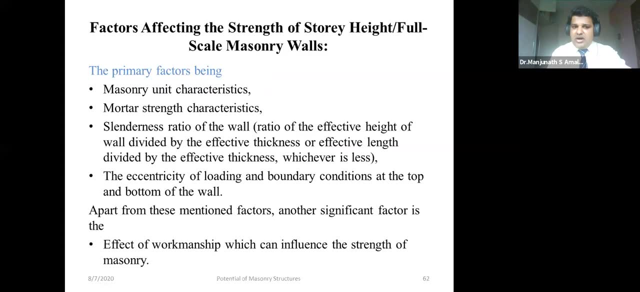 which is being applied- eccentric load- and along with that, you have a taller wall. obviously, there's a further reduction in the strength of, or the capacity of the wall. Well, this is what sums up these two points, That is, that it affects the slenderness ratio. 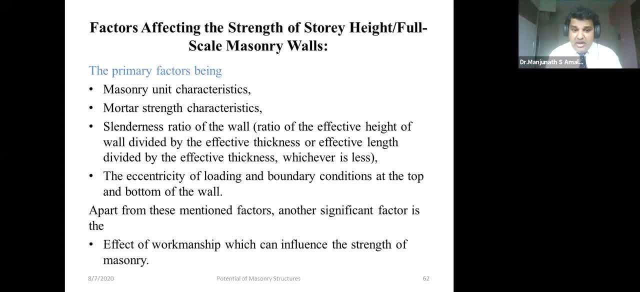 as well as the eccentricity of loading and, of course, the boundary conditions. Now, apart from that, very important in masonry is the effect of workmanship. If the workmanship is not proper, then definitely one can expect, you know. 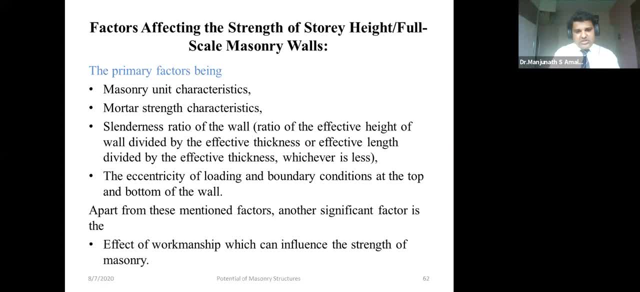 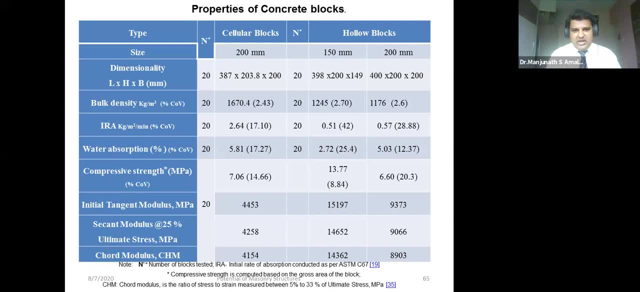 the strength to be hampered or there would be an influence in the strength of the masonry. Now, as I did mention, I thought I said you know I would be sharing a certain results of what we did For concrete blocks, you know. 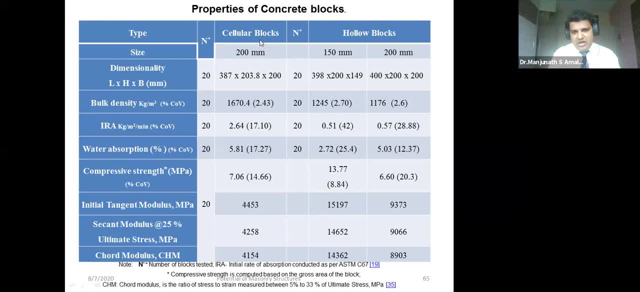 I have just specified to the concrete blocks. Well, these are the cellular blocks and these are the hollow concrete blocks. Now, if you remember, in the beginning I tried to distinguish what I mean by cellular and what do I mean by hollow. 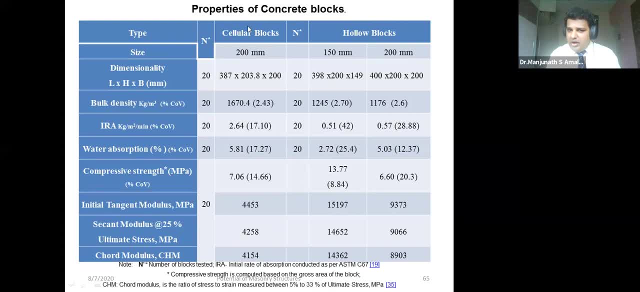 Just to repeat the fact: if I have a concrete block with smaller, or rather smaller diameter of hole, but more in number, then I would call it as cellular block. Well, if I have larger holes, and then that is your conventional hollow concrete block. 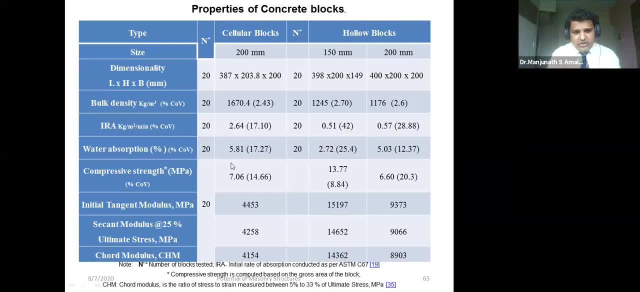 Well, the first initial rows talks about its, you know, physical properties. what's its dimension, what's its density, what is its initial rate of absorption and absorption itself. And, of course, you know, the more important parameter here is the structural properties. 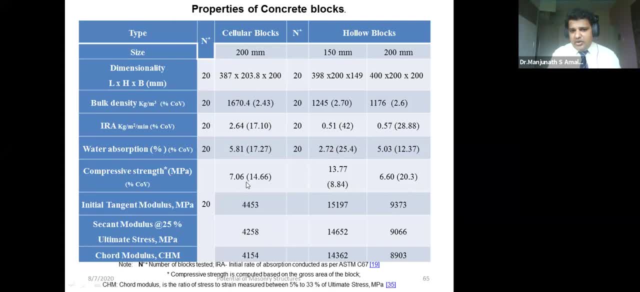 where now you see that it is around 7.06 MPa for a cellular block And we have looked upon, you know, two different sizes, which is 150 and 200 mm size blocks, which are giving 13.77 and 6.6 MPa. 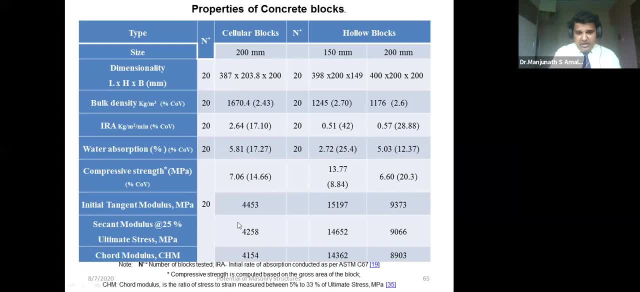 as the strengths respectively. And of course, you know, one would also want to know what are its elastic properties, and that is where we also try to test for its. you know for its. you know elastic properties, And that is where we also try to test for its, you know. 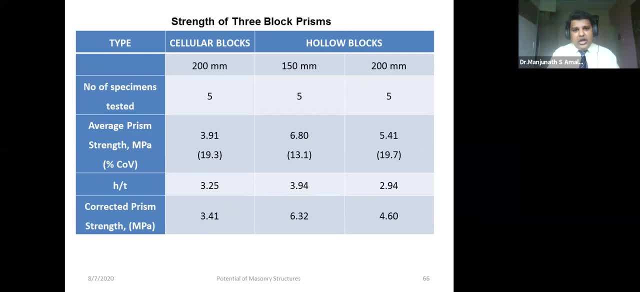 elastic properties, And that is where we also try to test for its- you know, tensile and young smartness assessment, And that is where we also try to test for its- you know, tensile and young smartness assessment. 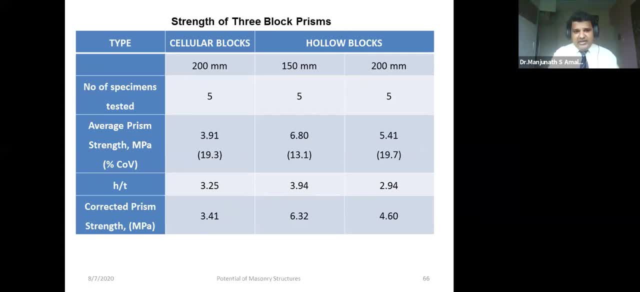 We also had to test for prisms. I will tell you why this test is required a little later. but yes, we, as we said, you know, we wanted to also look into the- you know- strength of three blocks prisms. 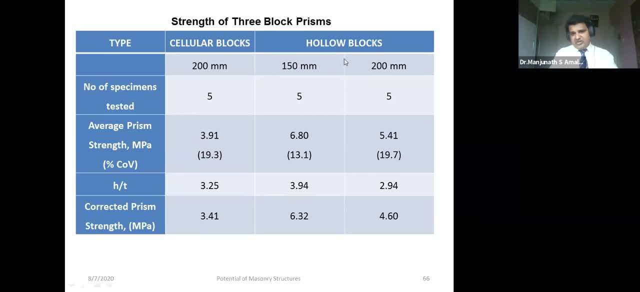 Well, again, the same blocks were used for same sizes. Well, again, the same blocks were used for same sizes. You could see that. you know, the strength was 3.91.. There is definitely a reduction because you know. 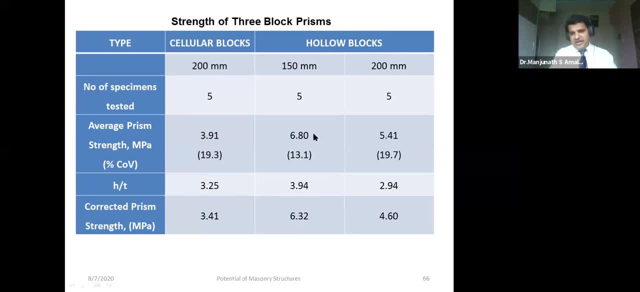 as you increase the height, obviously you can expect a reduction in the strength. that is what I said. And 5.41 is the prism strength, average prism strength for about five blocks. And you also see, in the last row here there's something called as corrected prism strength. 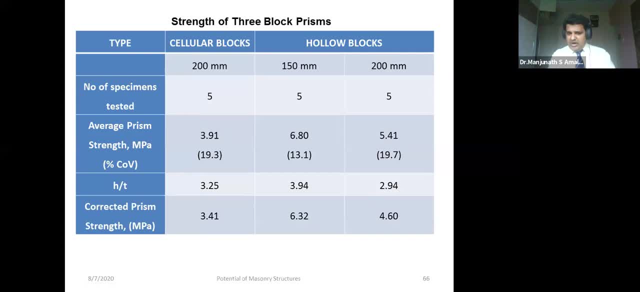 Now, what is this corrected prism strength. Well, this is a provision or this is a recommendation from the code where it says: all the prisms have to be normalized. the strengths have to be normalized for a slenderness ratio of two. 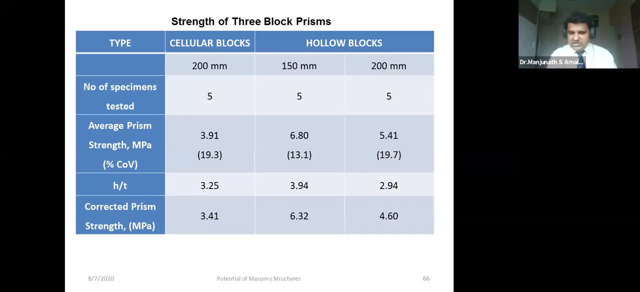 for the normalization of prism strength. On that note, we will also discuss how much is the prism strength and what is the correction factor one has to apply for a hollow block, And although now I would just leave it at here like, the corrected prism strength is 4.6,. 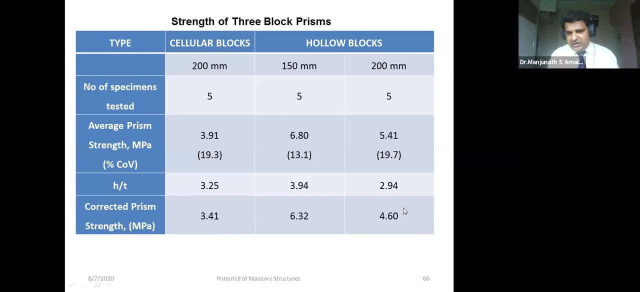 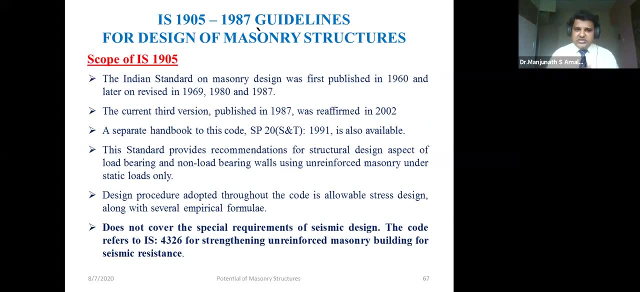 I will definitely come back to this value. how did I get this factor a little later, my friends, Now going forward very, very, very briefly. well, what is the code? Well, it is Indian standards 1905.. 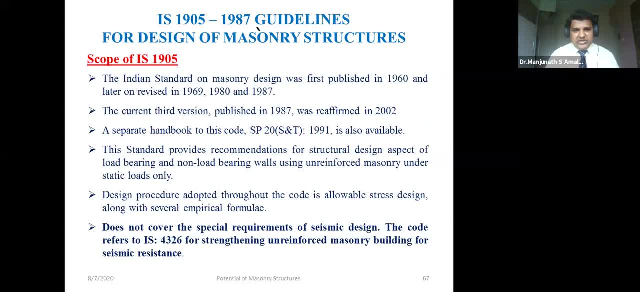 Well, this is the code which one has to look for if one has to design a masonry, an unreinforced masonry structure. Well, it was first published in 1960.. Well, it has further. it was revised three times. 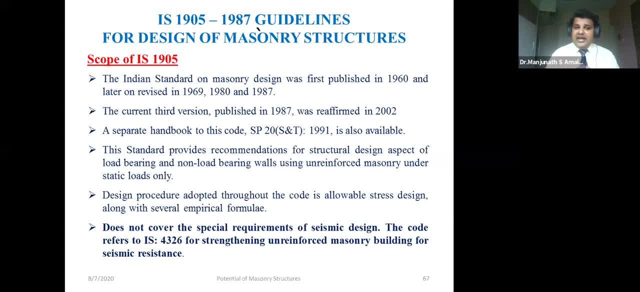 and was reaffirmed in 2002.. Well, like a separate handbook for code for RC, we have a separate handbook for masonry structures as well, in SP 20.. And well, you know, this is a code which provides recommendations for load bearing. 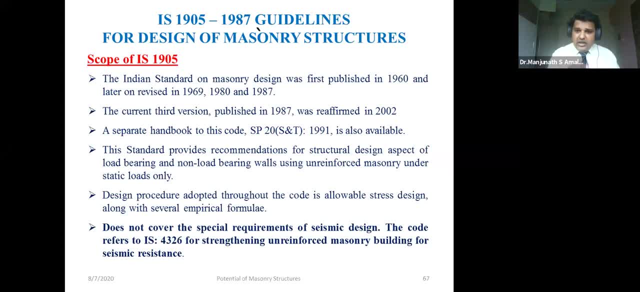 and non-load bearing walls for unreinforced masonry structures and for static loads only. Well, the philosophy of design as per the code is very simple. You know, the philosophy which is followed is allowable stress method, or what you can say as the working stress method. 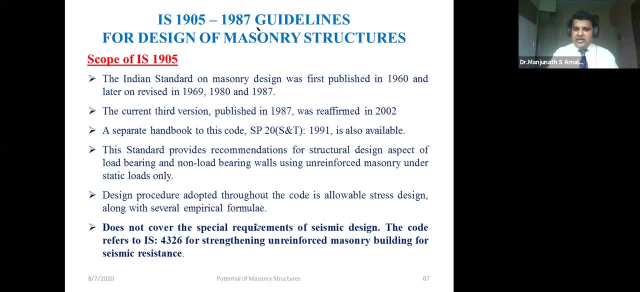 Well, if you want to design it for seismic loading, well there is a reference to IS 4-3-2-6.. If one wants to do a seismic design, one can refer one IS 4-3-2-6. 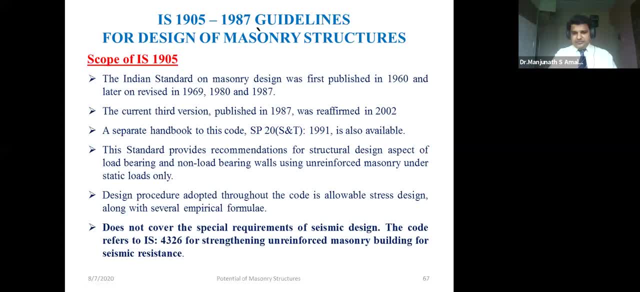 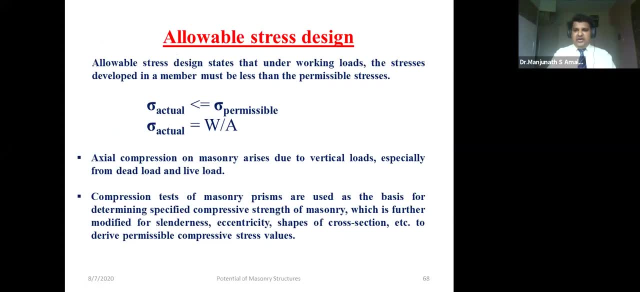 for something unreinforced masonry for the seismic resistance. Now, as we all know that, what is the fundamental principle behind the work allowable stress method is that you will have to find out the actual stress. Now, what are actual stresses? Stress by definition is load over. 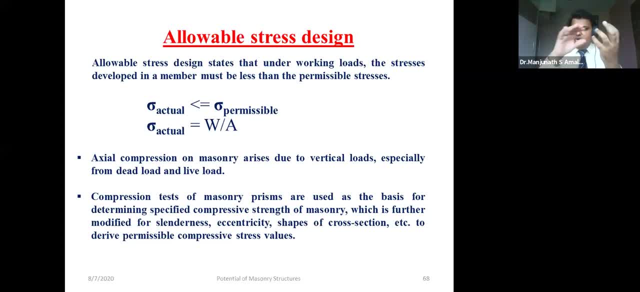 Now, if I have to find out what is the actual stress, I would want to know what is the load coming onto the wall, And then, of course, dividing it with the area will give me the actual stress. Well, this actual stress has to be compared. 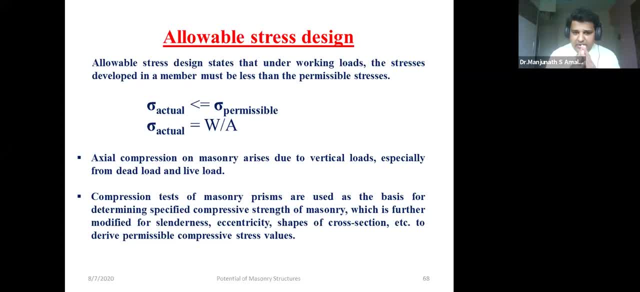 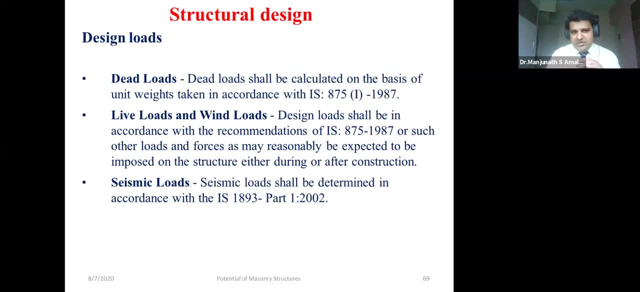 with something called as permissible stress. Now, how do I find out? the permissible stress is the next question, Now the core also, of course, you know, before we go on to the permissible stress. well, the loading, the dead load, the live load, 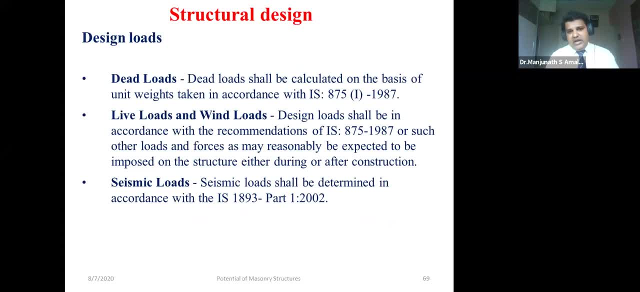 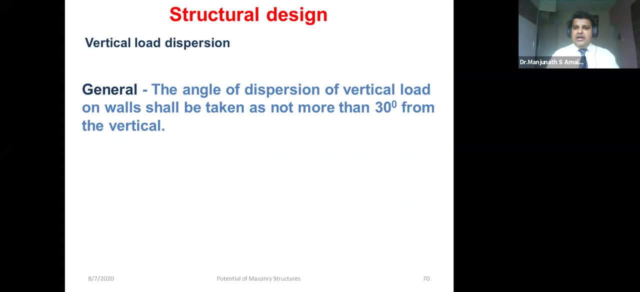 is all as per the, because I've already mentioned, you know, I'm looking at an RC slab here, So the loading is, as for RC structures, where you will, you know, refer IS 875 for its various categories of loads. Now and also before we go on to the permissible stress, 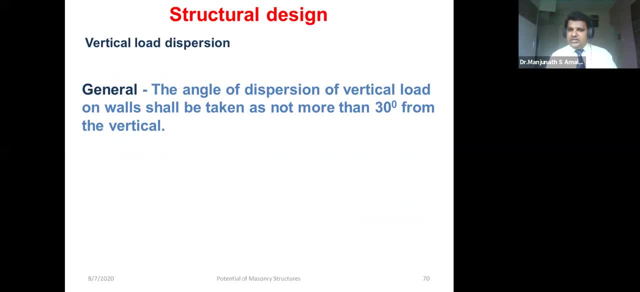 one has to understand. if I'm looking at, you know, the load dispersion for a wall, I would be looking at a dispersion angle of not more than 30 degrees. Where do we come across of this? I will talk about it a little later. 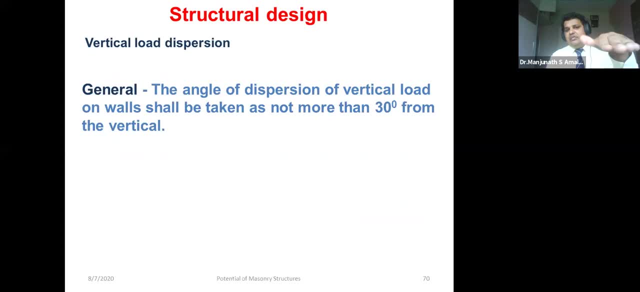 But for now I would like to mention that you know you would be coming up with the dispersion angles. whenever you have an opening in a wall, Like I say you have a window or a door, then one has to look upon what would be the angle. 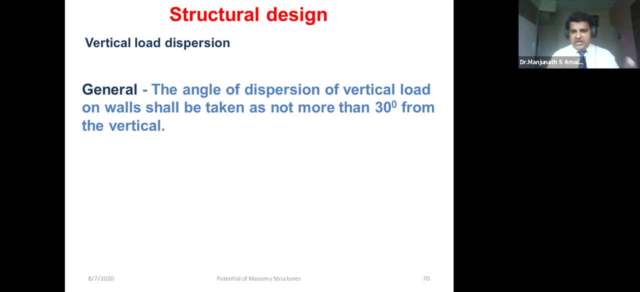 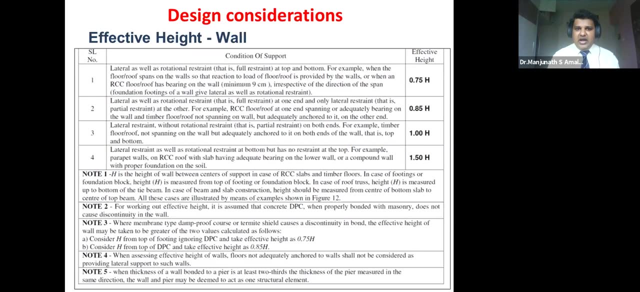 of dispersion of vertical loads on walls when such a scenario occurs. Well, looking at design one, like an RC design, one has to look into the effective height of the wall. I will not go into the details of it but, as we all know, like in RC or the simple column, 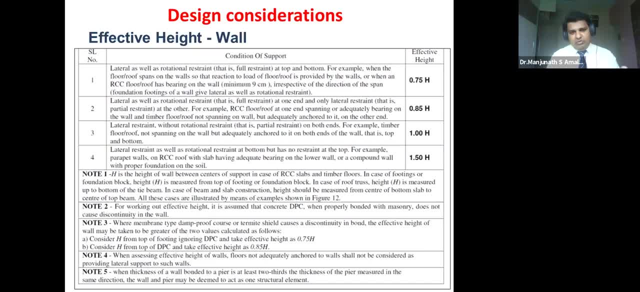 you know analysis, you know it all depends on what are the support conditions. Likewise, you know, based on what is the support conditions, one can arrive at whatever is the recommended effective height of the building. Now, well, this is the screenshot. 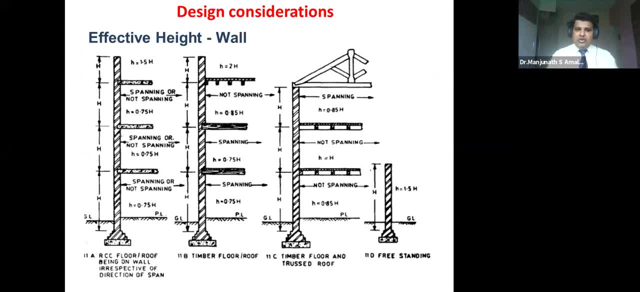 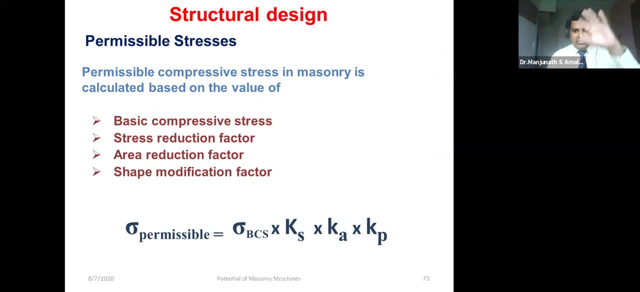 which I've just taken it from the code which gives you the guidelines: what has to be the effective height? Now, coming back to our permissible stress, because this is the one which we have to compare with our actual stresses. Now, the code says that you know. 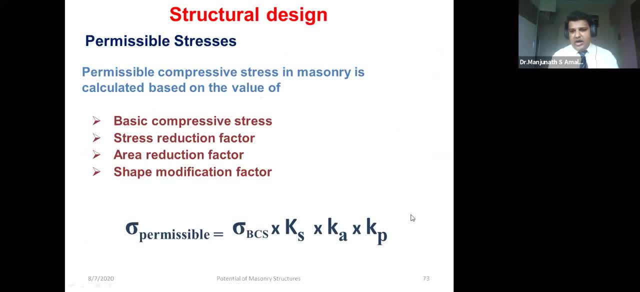 it can be calculated by these parameters. Now, what are these parameters? The first is, you know, the basic compressive stress. Now, what is basic compressive stress? We will talk about it. Well, this basic compressive stress has to be multiplied. 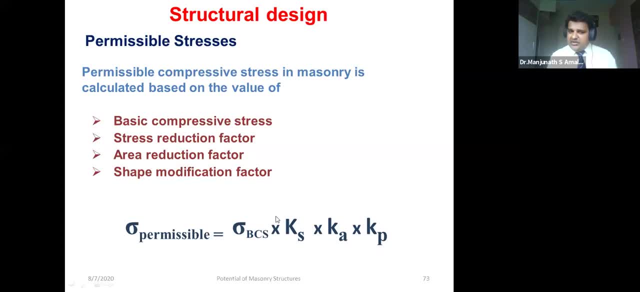 with certain reduction factors. Now, what are these factors? One is called as the stress reduction factor, depending on, depending on the stenderness, Other one being the area reduction factor, based on the shape of the block. And the other one the last one, 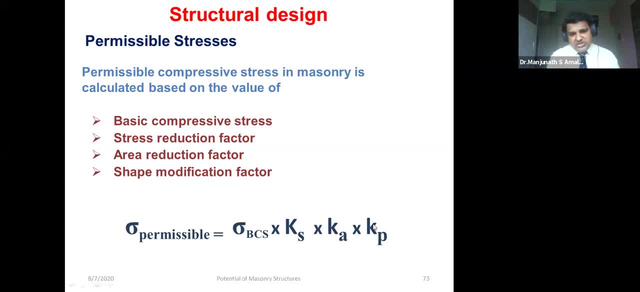 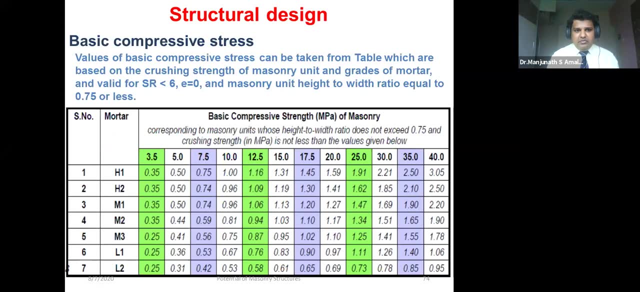 which is called as the shape modification factor, depends on what is the shape of the block. Now, very briefly, we will just go into it one by one. Let us look at basic compressive stress. Now, where do I find basic compressive stress? 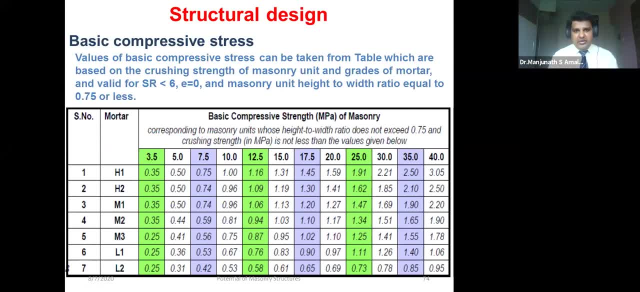 Now there is a chart or a table given in the code where it talks about, you know, the stress. it talks about basic compressive stress, you know, for those blocks where the height to width ratio does not exceed 0.75.. 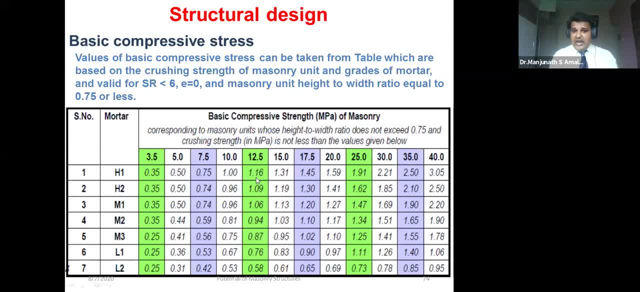 Now, this table- definitely for that reason- can be used only if your block has a height to width ratio when it is being laid. the height of the block to the width of the block when it is being laid it should not exceed 0.75.. 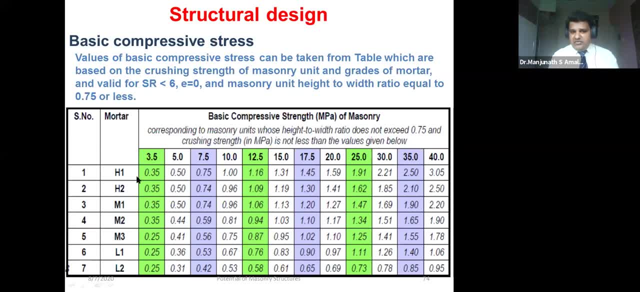 If that is the condition- knowing what is the matter we are trying to use and knowing what is the block strength- here one can arrive what would be the basic compressive stress. Well, this is one option to find out the basic compressive stress. 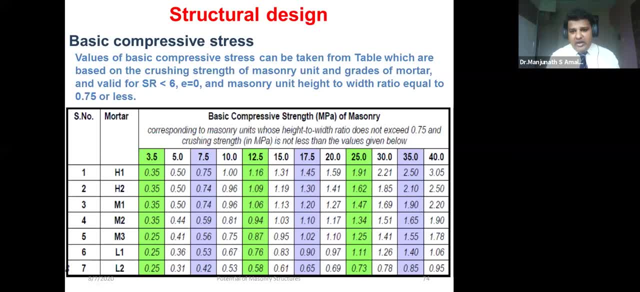 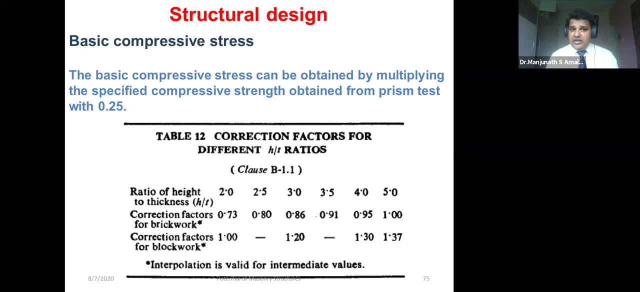 Looking at what is the other option. the code also says: now, what happens if H by T of the unit exceeds 0.75?? Now, in that case, well, the code says: if you have to find out the basic compressive stress, 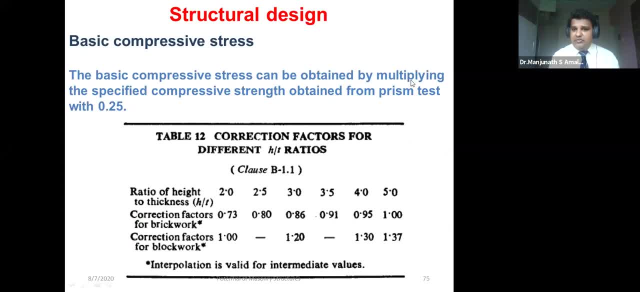 all you have to do is multiply this value of you know value of the presumed strength, which you obtain experimentally, with 0.25.. In other words, all you have to do is divide the presumed strength by four in order to get the basic compressive stress. okay. 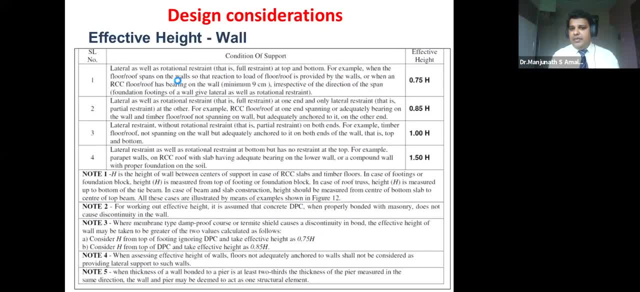 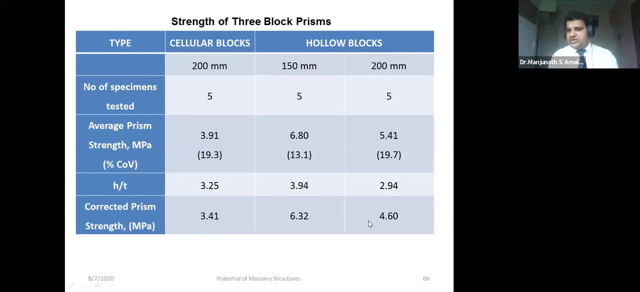 So, like if I just quickly go back here now, this was the strength which I was talking about. if you remember, I told you that this is the presumed strength, which is 4.6, and I called it as corrected presumed strength. 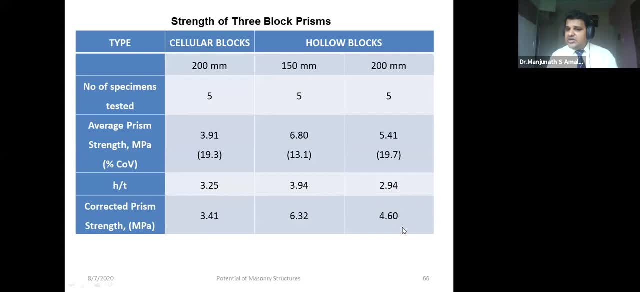 Now all I have to do if I have to get basic compressive stress is just divide 4.6 divided by four, or multiply this with 0.25, which will give me the basic compressive stress. Now, that would be the value. 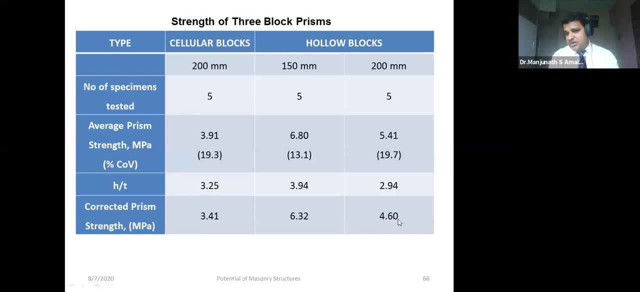 Now, how did I get 4.6 is another thing which we have to understand, because we got this 4.6, and we got this 4.6.. Based on the experimental value of 5.41.. Now, going back to the same slide here, 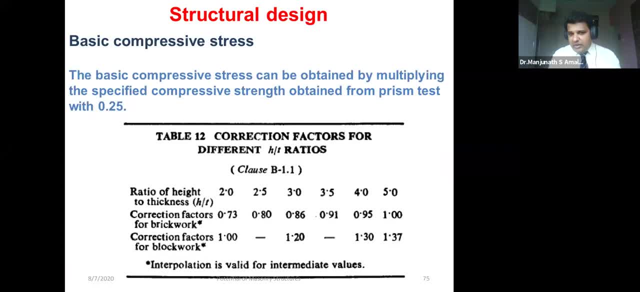 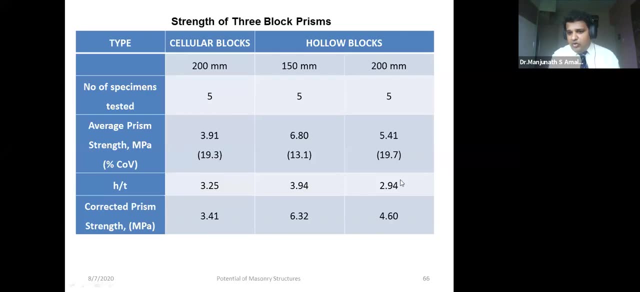 if you look here, there is another table which talks about the correction factor for the prisms. As I told you, it is normalized for H by T of two. In that note, going back again very quickly, 2.94 is my H by T. 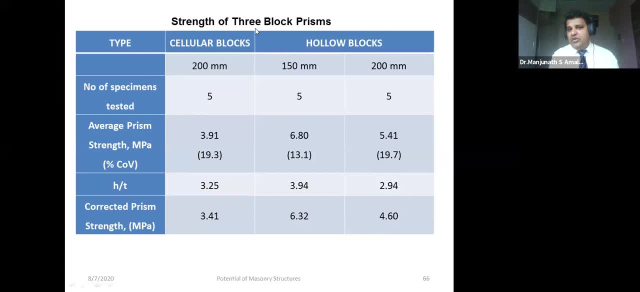 H by T. how did I get 2.94? Because it was a three block prism, So one above the other. So it is, let us say, if it is a 200 mm block. you know, let us say 200 three times with two water joints. 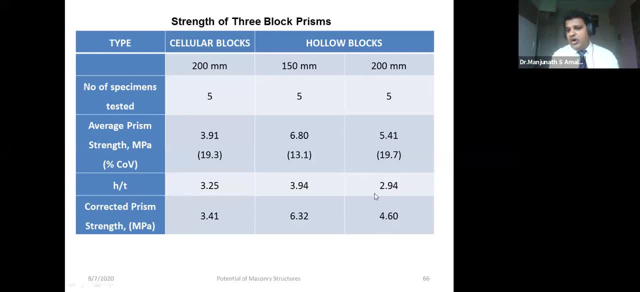 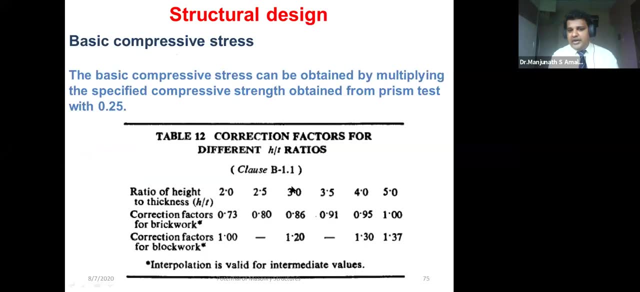 will give me a certain value of H. If I divide it with 200 mm thickness, will give me this value of 2.94.. And all I have to do is go back to that table and look at this. what is the value for? 2 point less? 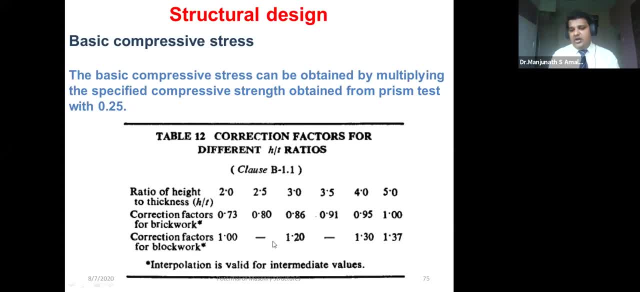 let us say 94.. I always- it permits interpolation- I can always find out the correction factor and then go about there and use it for the correction factors to be applied as applicable Now. well, we finished with the first part. 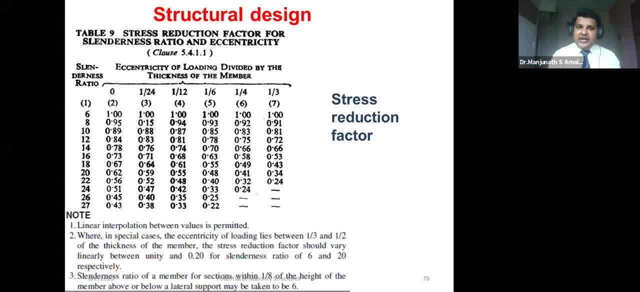 which is to find out the basic compressive stress. Now, what about the factors? The factors, as, again, there are tables mentioned in the code, but, as I said, KS is something on stress reduction factor. Now, what does it depend? 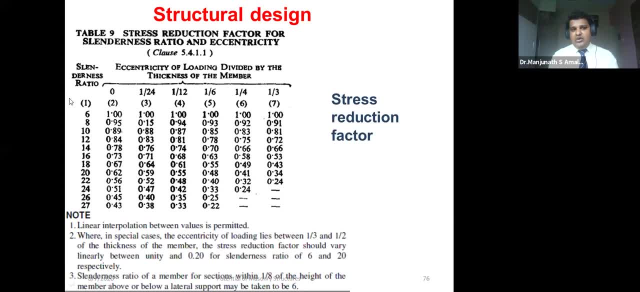 It depends on the slenderness ratio and eccentricity. Now, slenderness ratio, how do I get? I just take the height of the wall, divide it by the thickness. I would get the slenderness ratio. Let us say, if I'm not looking at any eccentricity, 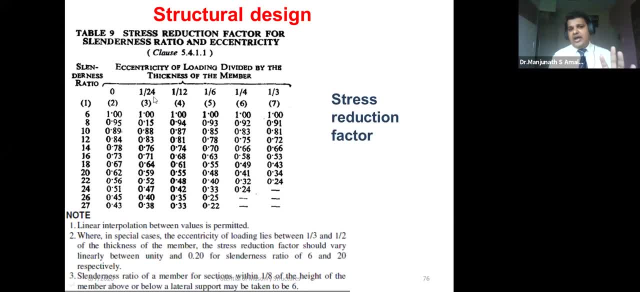 only concentric. let us say, I take the eccentricity as zero or as applicable. then one can get what is the slenderness, what is the stress reduction factor from this particular table nine, my friends? And then the area reduction factor. 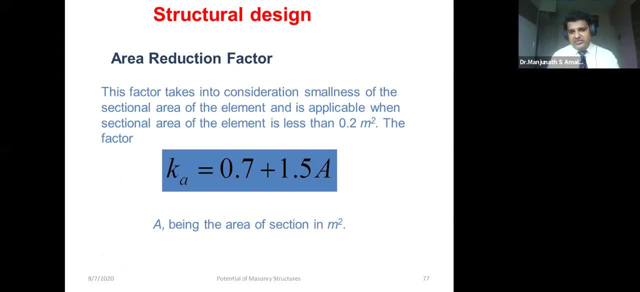 If this particular factor takes into the smallness of the section of the block- and it's applicable where the section is less than 0.2 meter square- the area of the section is less than 0.2 meter square, well, which can be calculated using this particular equation. 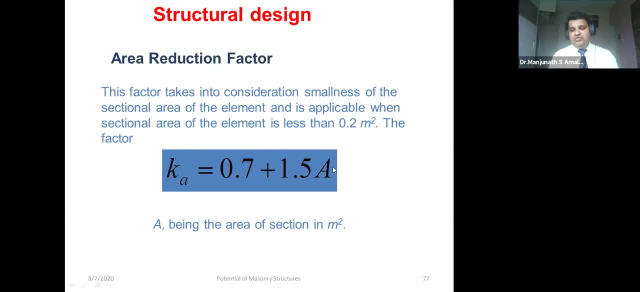 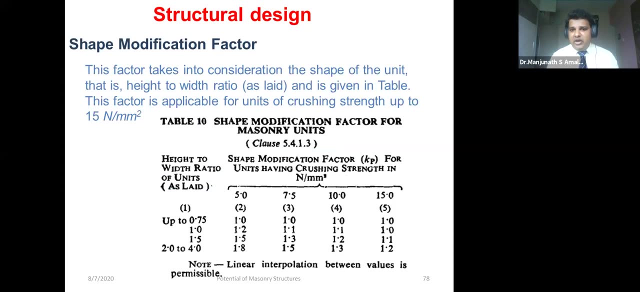 All you have to do is find out what is the area of the block. multiply it 1.5, then 0.71 can arrive at K. Finally, we also have to look at the shape modification. It takes into the shape. 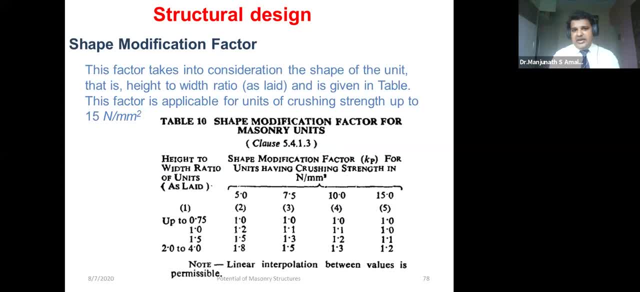 into account, as the very name indicates. and then you have to look at what is the H by T ratio. So the table gives you the H by T ratio, along for the strengths of the blocks which you are, which you have found out, the compressive strength. 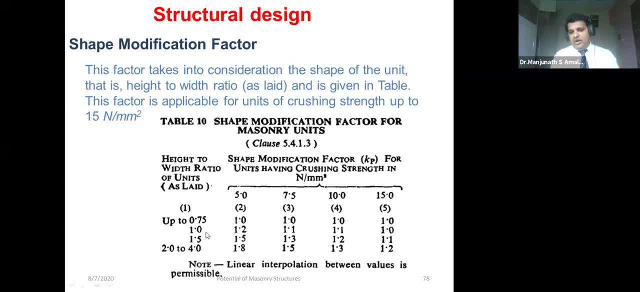 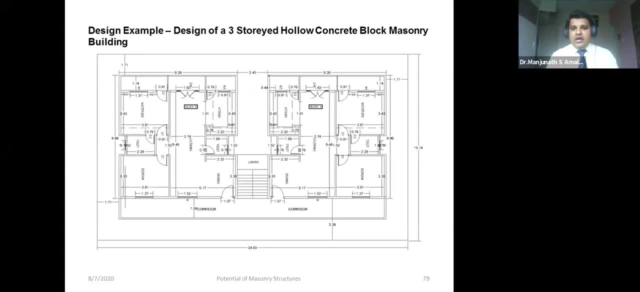 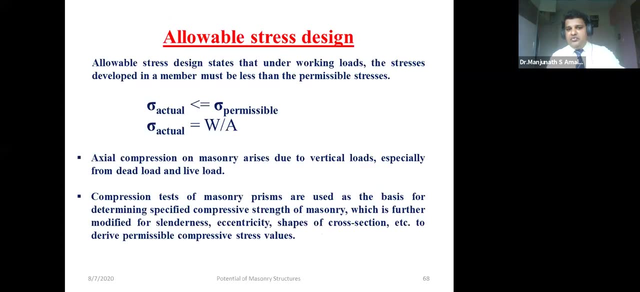 of the blocks earlier. knowing what is the compressive strength, what is the ratio, one can find out the shape modification factor, Kp, as well. my friends, Now we have this fundamental equation, we know how to find our Sigma actual. 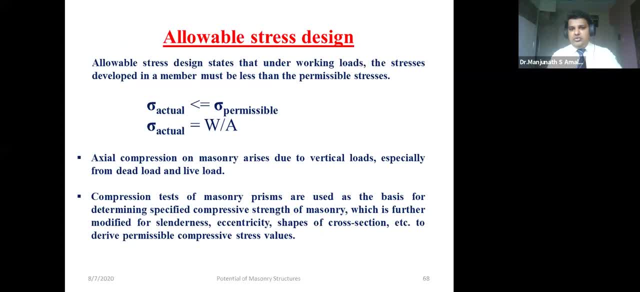 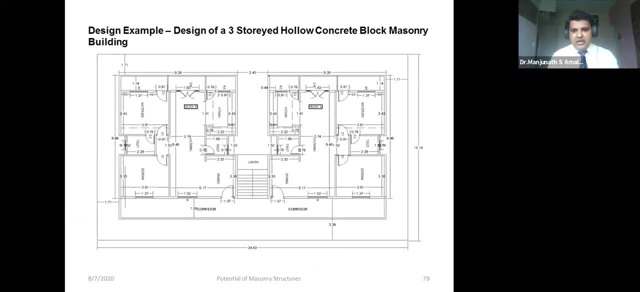 We know how to find our Sigma permissible. Now, just to you know, wind up here. let me take a small example of, let us say, a multi-story building. Now I have here a multi-story building. I've just taken a random plan. 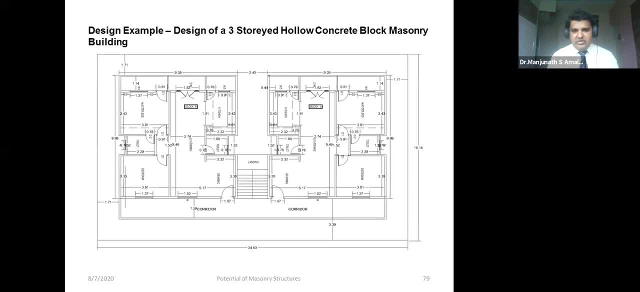 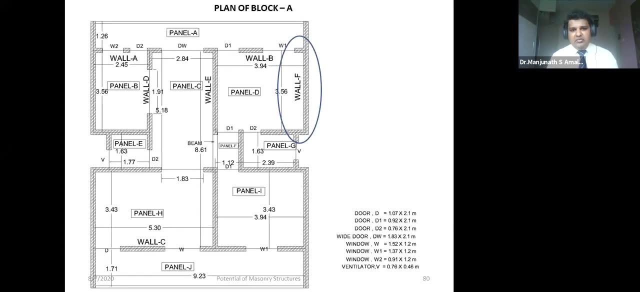 Well, this particular plan, we have, you know, a luckily a symmetrical plan here and which is divided into block A and block B. let us say, And this, let me concentrate on one of the block, as it is symmetrical- 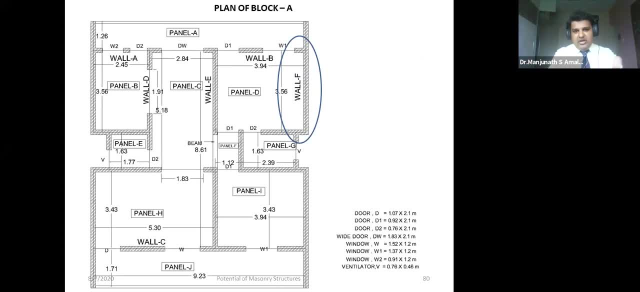 And it is being divided as panels and walls. I've given the naming for each of the walls as wall A, B, C And for our design, let me choose this one Because of want of time. I don't want to go into the other walls. 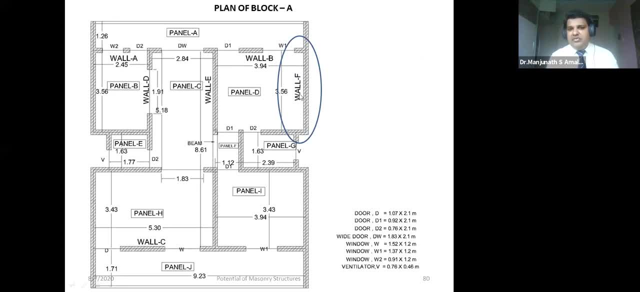 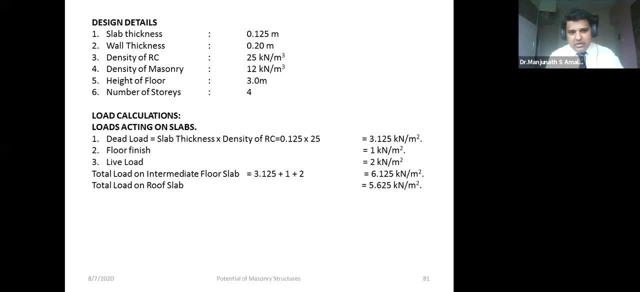 But I'm just taking one solid wall here which I would very quickly try to look at the design of it. Sir, do we still have time? Hello, Yes, sir, Yes, sir, Yeah, I'll take a maximum of 10 minutes more. 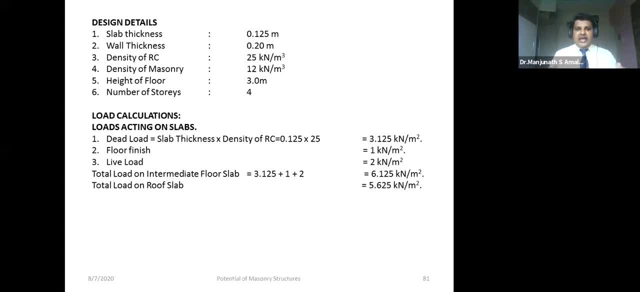 Yes sir, Yes sir, Continue, Continue, Yeah. So what is the calculation involved? Well, the design. it's like any conventional Because, as I mentioned earlier, we are looking at a conventional RC slab which has to be supported by our masonry. 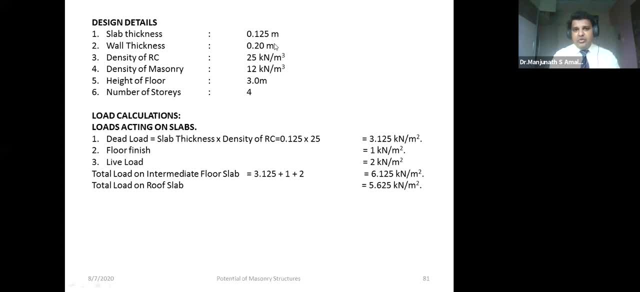 Now, let us assume a slab thickness of 0.12.. 5 meter. The thickness of the wall has 0.2.. Well, the density of RC, as we know, is 25.. And then the density of masonry. 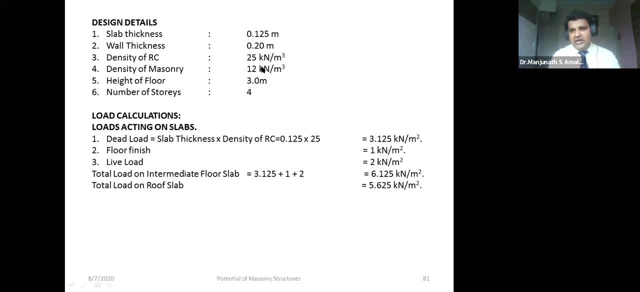 Now, where did I get? What is the masonry I'm trying to use? Well, I'm trying to use the density of hollow concrete block masonry, which is the one which I mentioned in the table, where the density was around 12 newton per meter cube. 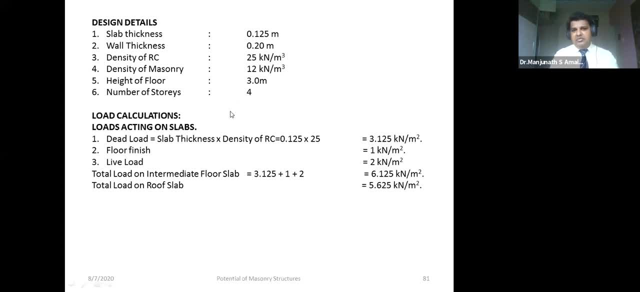 Well, of course, the height of the floor is 3 meters And let me look at what is the feasibility of the one which I tested, if it is OK, for, let us say, a G plus 3 or a four storey building. 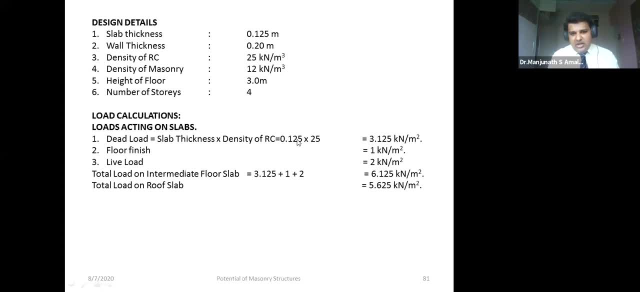 The calculations of slabs goes as usual, where you will have to find out the dead load, the thickness into the density, the floor finish, depending on what is the kind of building, the live load based on what is the usage of the building. 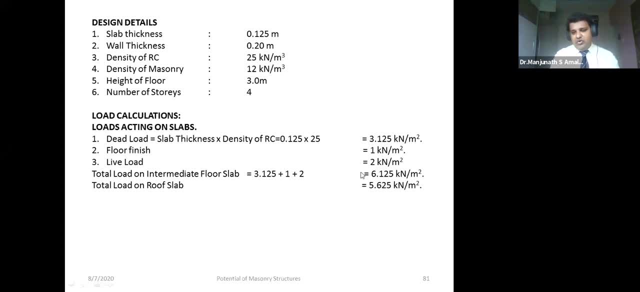 One can arrive at what would be the total floor slab load, which is 6.125 kilonewton per meter square. Now if I have to look at for a roof slab, obviously I'm going to maybe reduce upon the live load. 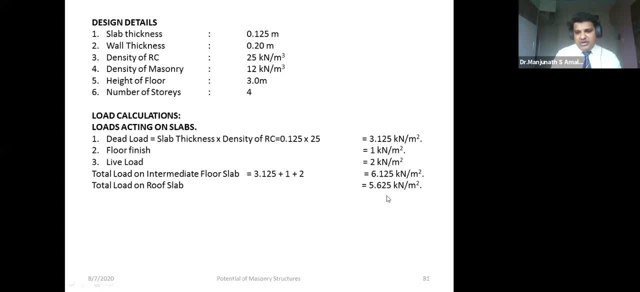 And then maybe by another 0.5 kilonewton per meter square, let us say, I would end up getting a roof load of 5.625.. Now if I'm looking for one floor, one plus one, let us say: 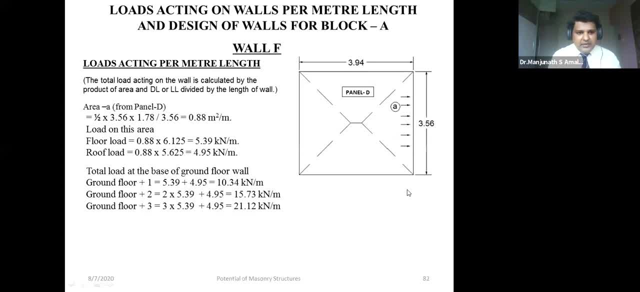 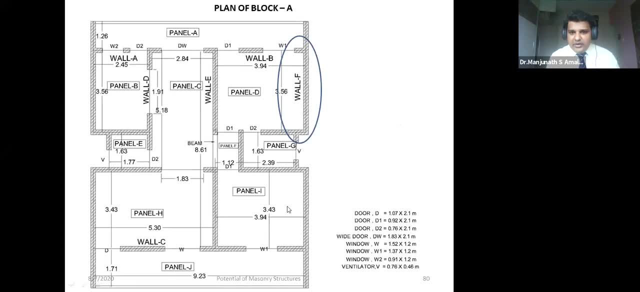 it will be a combination of these two, like what I have here Now. going back to my plan. going back to my plan Now, this is the wall which I have identified. Now, The panel which the wall has to support is panel D. 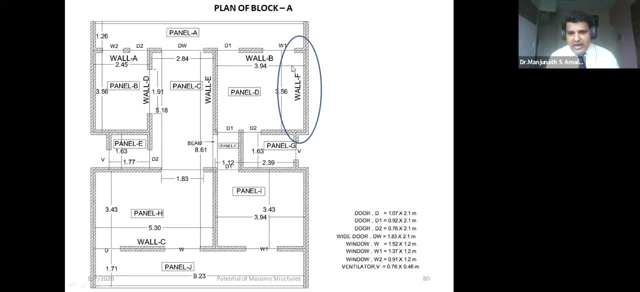 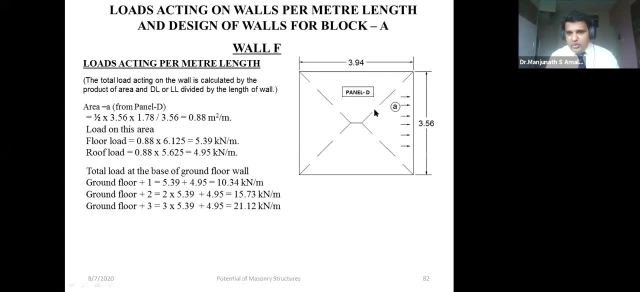 The dimensions of the roof is 3.94 and 3.56.. So this is the panel. So I go back here. It looks like it is a two way slab, which it is. Now I'm trying to support a wall on this face of the slab. 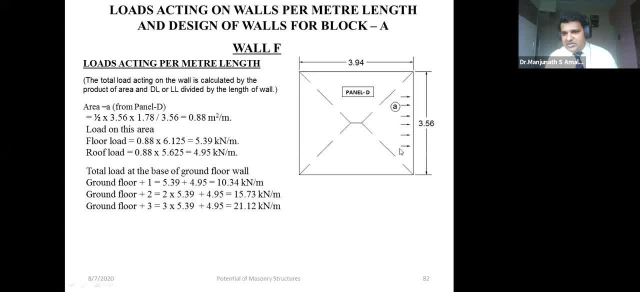 Now all I have to do is try to find out what is this area of the slab which this wall has to support, Going with the fundamental understanding of our roof, This is the triangular portion which has to be supported, So I would go with finding out what is the area of this triangle. 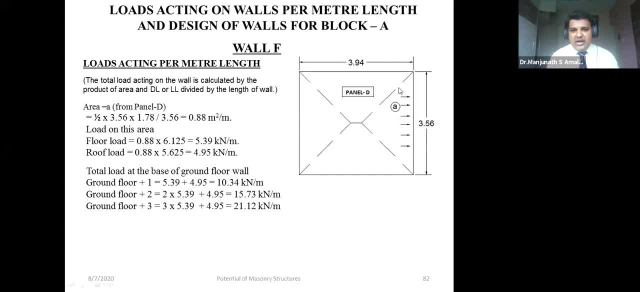 I would find out the area of this triangle with this yield line specifying me the angle. Now all I have to do is find the area and divide it with the length of the wall, so that per meter length of the area. So that is the area of the wall. 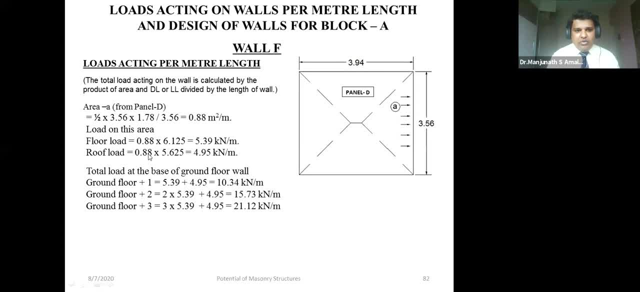 So Okay, So this is the area per meter. Having known what is the area, we have previously calculated what is the load. Now, all you have to do is now multiply the area in meter square per meter into the load, which is in kilonewton per meter square. 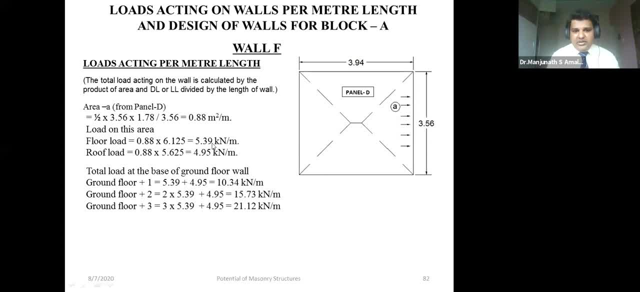 Meter square, meter square gets canceled. So I have the floor load as 5.39 kilonewton per meter And from the roof I have it as 4.95 kilonewton per meter. Now this is a per meter uniformly distributed load which the wall has. 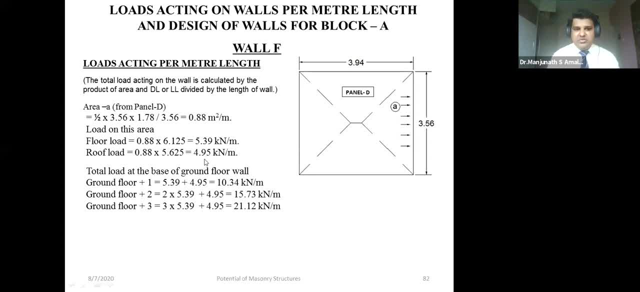 So this is the floor load, So this is the floor load Which the wall has to resist, my friends. Now, if I let us say I take a ground floor plus one, I just have to add these two, as I told earlier, which comes up to this figure. 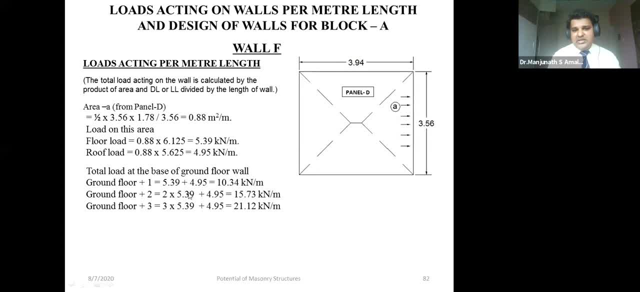 Now let us say I want G plus two. well, you just have to take twice the intermediate plus one roof. Likewise, my intention was to have a G plus three, So I have it as 21.12, that is three times intermediate floor, one time roof load giving. 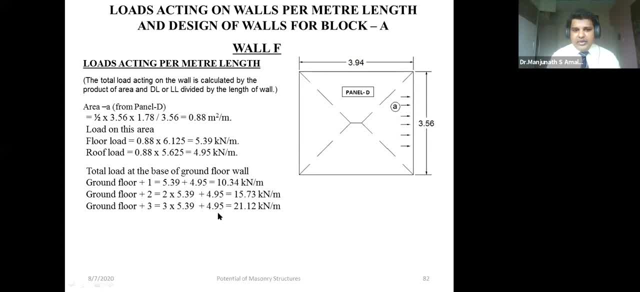 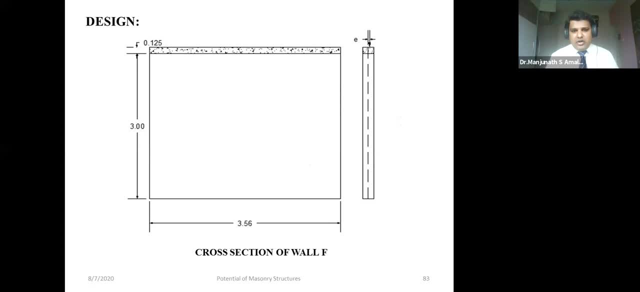 me this value of 21.12.. Going ahead now, this section. I told you I have selected a solid wall, although not all wall. we will not be fortunate to have all walls as solid walls. We will definitely have some openings, windows or doors. because of want of time, I could. 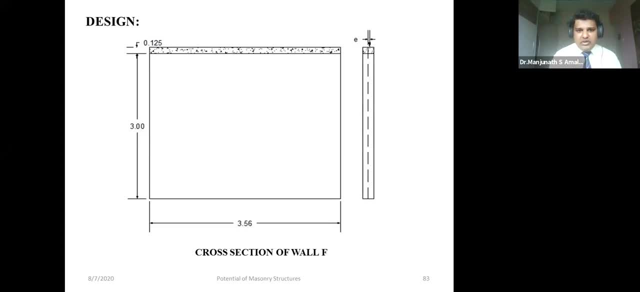 maybe not, you know, touch upon that. it would require a little more time. So I have just simply taken a solid wall for for, for our understanding, let us say this is the solid wall. Okay, This is the section of the wall. 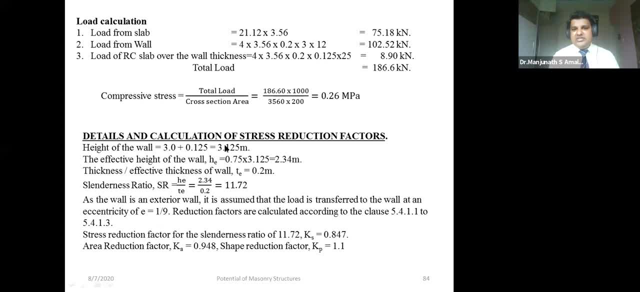 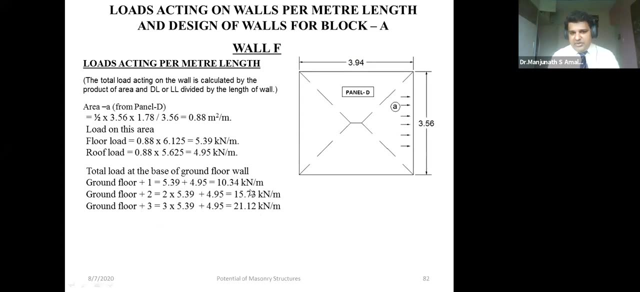 Now let me first find out what are to find out. what is the actual stress? actual stress. Let me convert all the UDLs into the point flow. Now we saw the slab load which we calculated here: 21.12, which is for G plus three into. 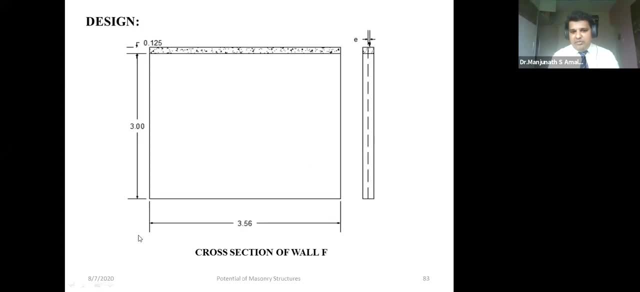 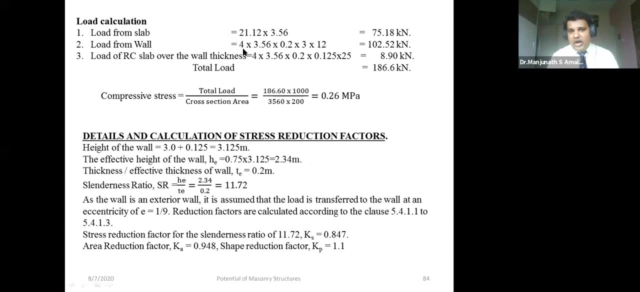 the length of the wall, which is our 3.56.. Now I have converted the UDL to a point. Similarly, I have the wall. one wall have to be resting the other, So there are four such walls. So four walls into the length of the wall, into its thickness, into the height of each. 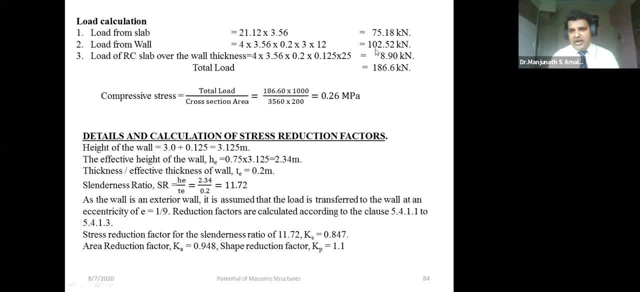 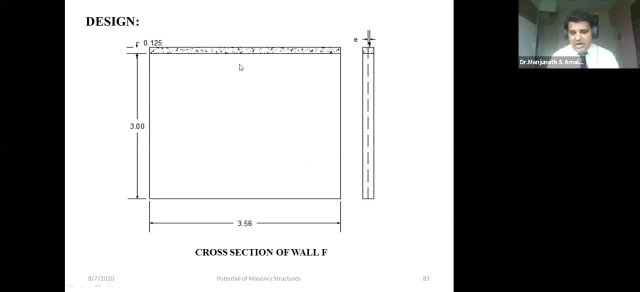 storey into its density, which is 12,, giving this value of 1.02.. Then, of course, you know you have a certain amount of slab resting on the wall which has not been accounted, Let us say, although it's a very small value of it. 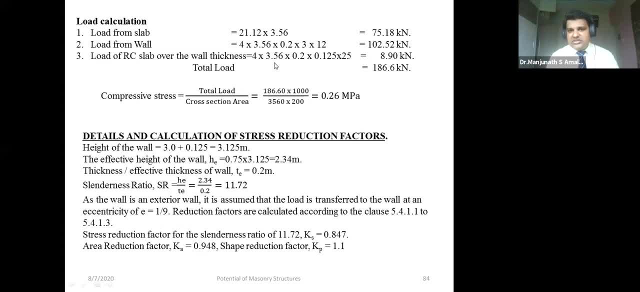 Let me also take that also into account. Again, there are four such slabs: 3.56,. thickness is 0.2.. The slab thickness was 0.125, 0.25, the density of concrete giving up on a lower value. 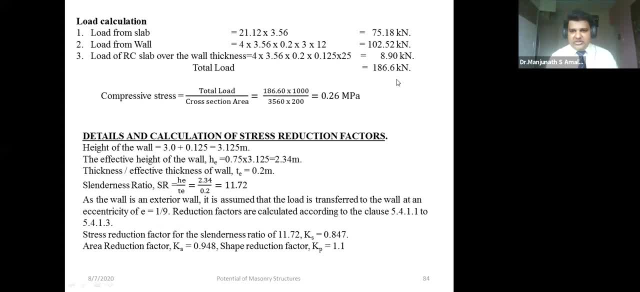 Nevertheless, it's been incorporated. So the total load is 186.6.. Now the stress. we know: load divided by area. We have the load in kilonewton and the area. Now what is the area? Very simple, It is 3.56, the length of the wall into its thickness. 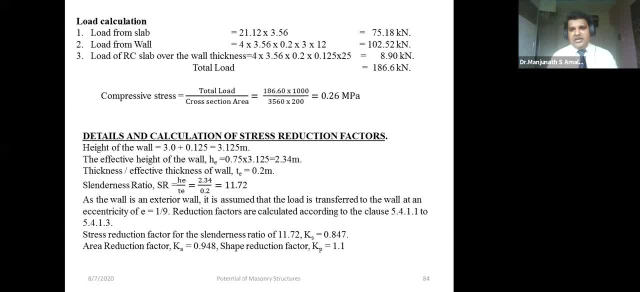 As we, as, as we have assumed, point Okay, Point to thick wall. Well, the thickness is 200 mm and you have the load in Newton now and the area in mm square, giving a value of 0.26 Newton per mm square. my friends, 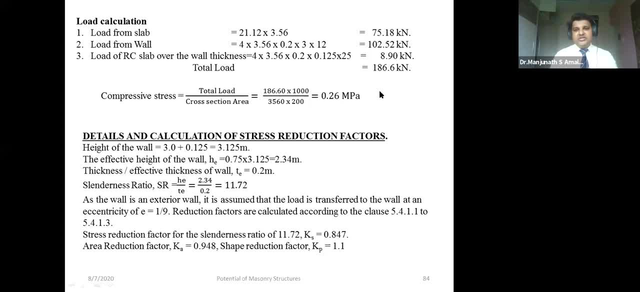 Now I have with me the actual stress ready. All I have to do is now compare it with my permissible stress. Now, permissible stress, as we said, I will have to take the basic compressive stress and then we'll have to take the area reduction factors. 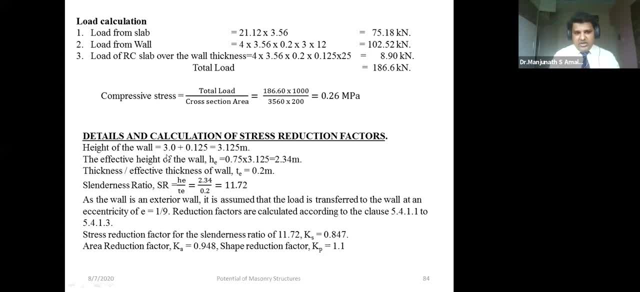 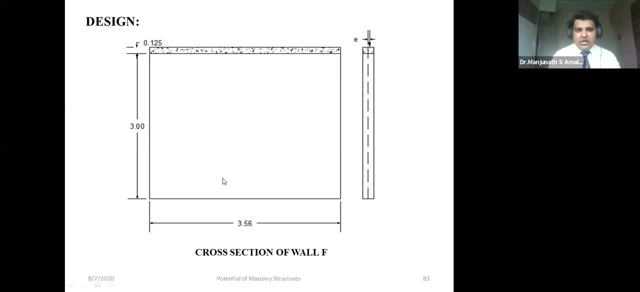 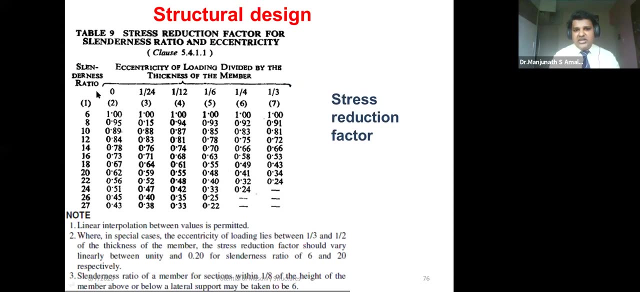 All right, Not only area, but then all the three factors. first, one by one, let us first find out the shape reduction factor. shape reduction factor- Well, this is the one it. it requires you to know that. what is the stenderness ratio? 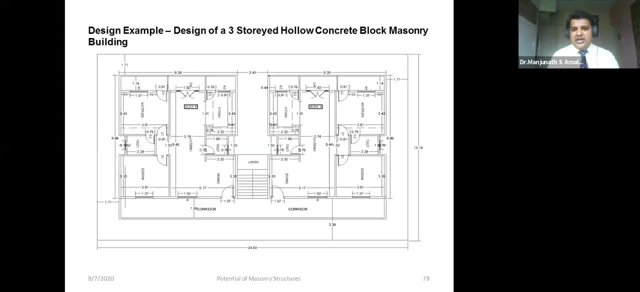 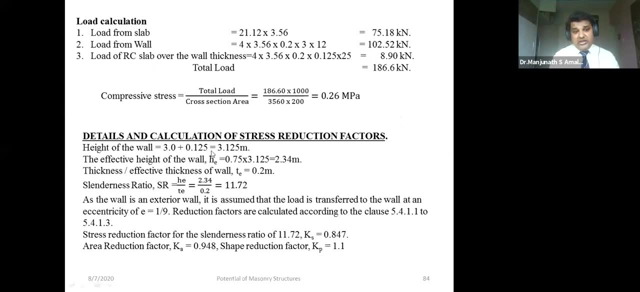 So we will simply go and find out what is the stenderness ratio. Well, the stenderness ratio we know, by definition. it is nothing but the height of the wall to its thickness. Now, height, I cannot take the actual height. 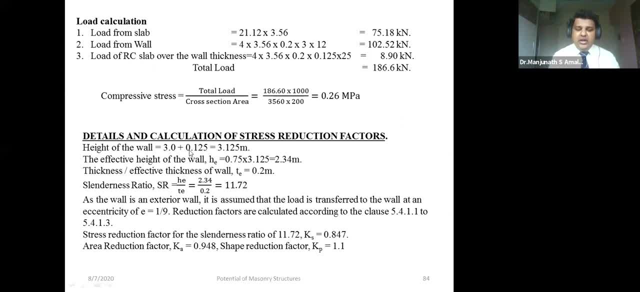 But I'll have to take the actual height. But I'll have to take the effective height based on the support conditions. Now, three meters clear height plus your slab thickness, 3.025, based on whatever support condition I have taken here- 0.75, H times H as effective height, then you get 2.34 meters. 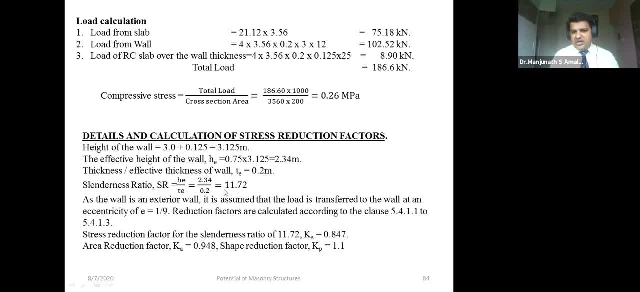 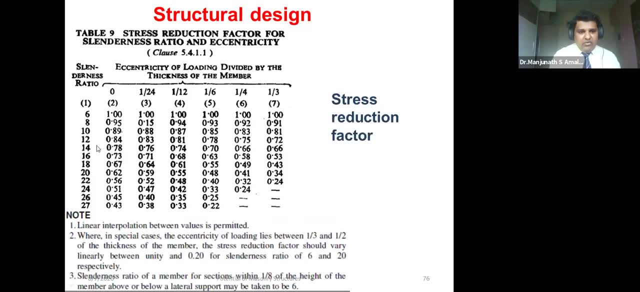 which is divided by the thickness, giving me the stenderness ratio of 11.72,. my friends, All I have to do now is go to this table and find out For a value of 11.72,. I have the choice of interpolation and I can maybe take it as. 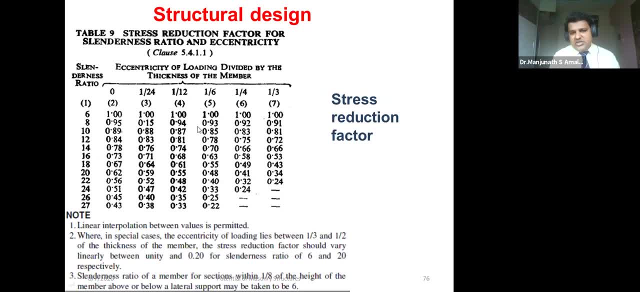 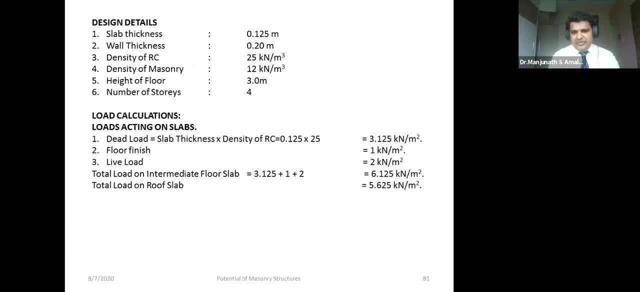 zero eccentricity, or usually, when it is an exterior wall, they prefer it to be taken as one ninth of an eccentricity. So therefore, based on that case, the case you know, one can arrive at what would be the value of the stenderness ratio. 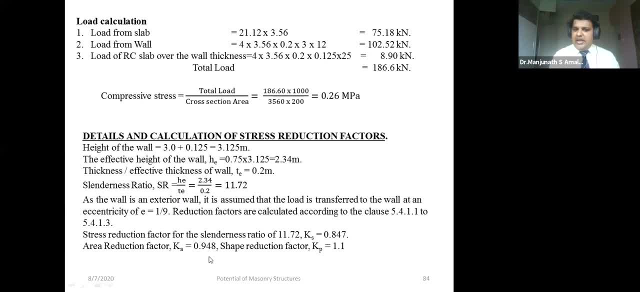 It is 0.847.. Also, Ka Ka, I told you it is 0.7 plus 1.5 times H, The area. you know what is the area of the block. you multiply with 1.5 times plus add. 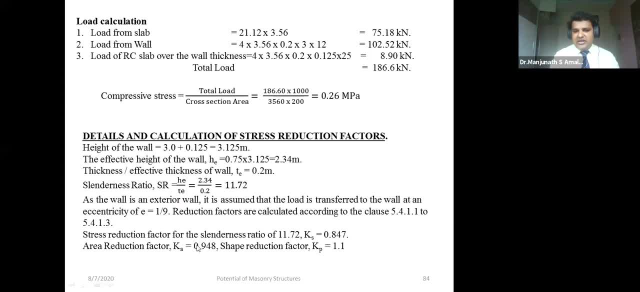 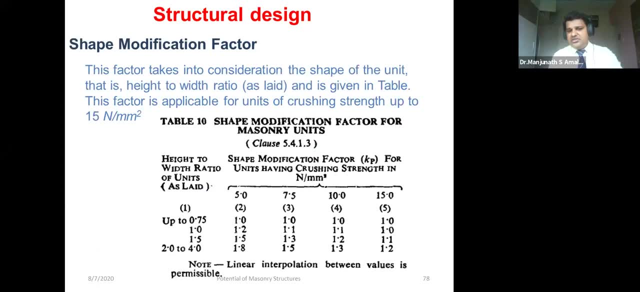 another factor of 0.7, you will get the area reduction factor, which is here, my friends, And then finally, the shape modification factor. Now this one, and based on what is the strength? where do I get the strength? I will again go back to my experimental data and check what is the strength of the block. 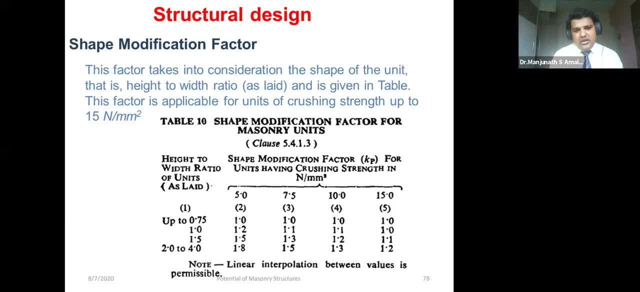 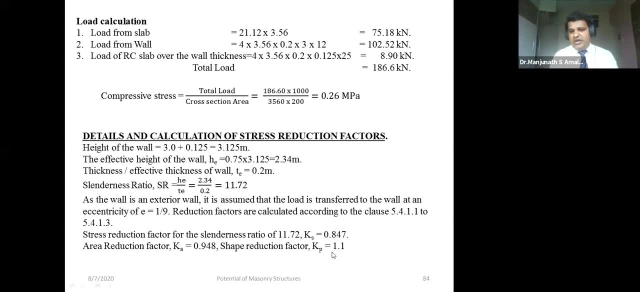 which I had got, And then looking at what is the H by T as late for the unit, I can, I know, arrive at what would be the shape reduction factor, as I have got here as 1.1,. my friends, Now it's time to get in all of them together. 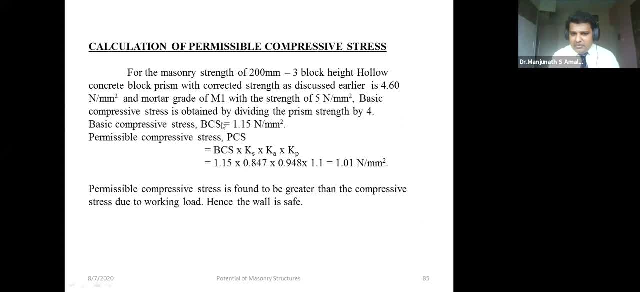 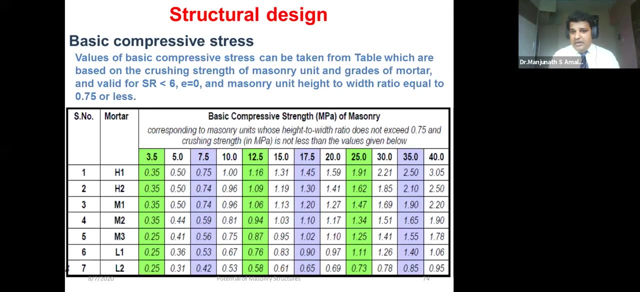 I, as I told in the beginning, just a little while earlier, my friends, I have to multiply these factors with something called as basic compressive stress. Now, basic compressive stress, how do I get? I could have used this particular table, but 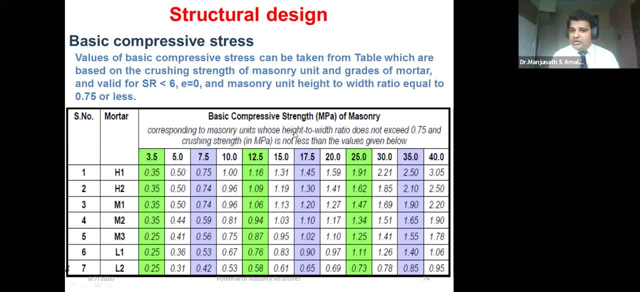 then This particular table is for the units whose height to width ratio should not be exceeding 0.75.. Now, unfortunately, our block is not having, or rather it's having, a ratio of more than 0.75.. So I cannot go with this table. 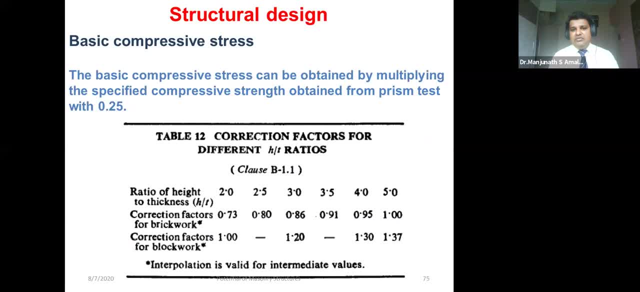 This usually fits in for a brick masonry. Well, I'll have to go with the second option which I have find out: the present strength divided with four to get the required basic compressive strength. So that's precisely what we will do. 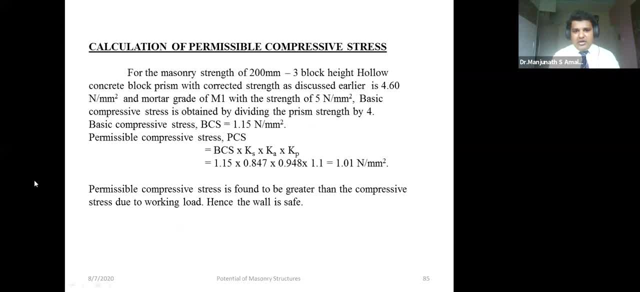 Okay, So what I'm going to do? go back here, look at what was my compressive strength. If you remember, if you recall, it was 4.6,. my friends, 4.6 divided by four is 1.15.. 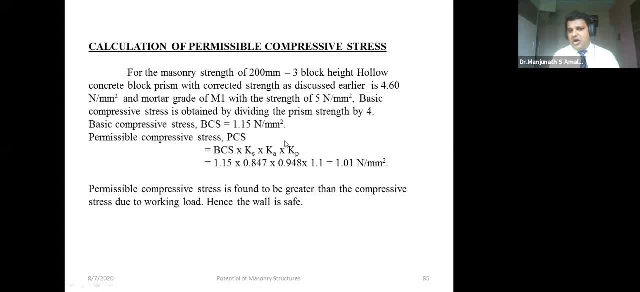 Now this 1.15 is just multiplied with all the other three factors and you get up a permissible stress of 1.01.. Now you can expect, because it's a solid wall, one can expect a larger permissible stress for sure, Because there are no openings. 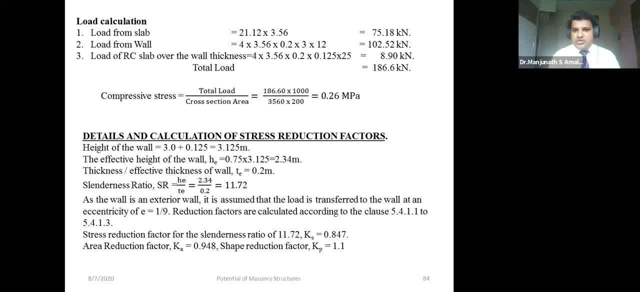 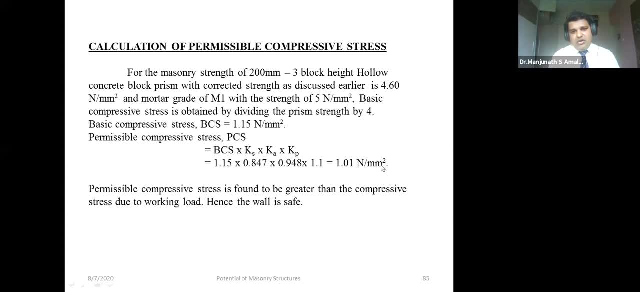 So, you know, I just compare with these two values: actual stress 0.26, permissible stress 1.01.. Well, the actual stress is less than the permissible stress. So then, therefore, my wall is safe. Well, this is a I tried to, you know, get it as a simpler as possible. 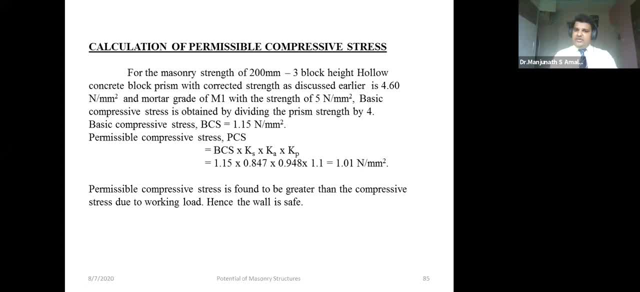 And the wall which was chosen also was a solid wall. So therefore, my friends, you know we ended up having this wall to be, you know, extra safe, if I can say so. Well, if you have other walls, so then let us say. if I go back to the plan, let us say: 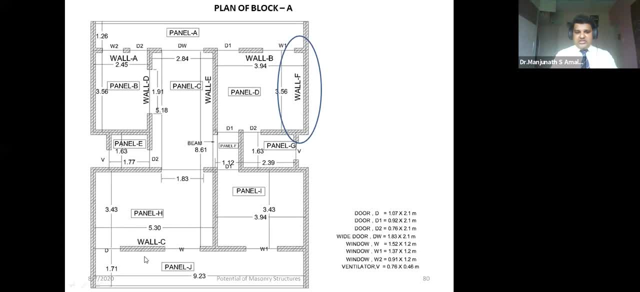 I have few walls here, wall D or wall C. Well, you see, my friends, for such walls there are openings for doors and windows, but if that is the situation, then then you cannot take the entire length of the wall, Okay. 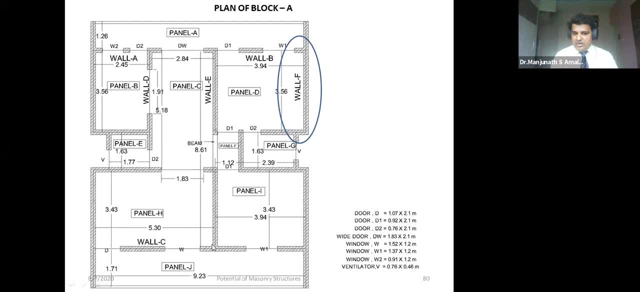 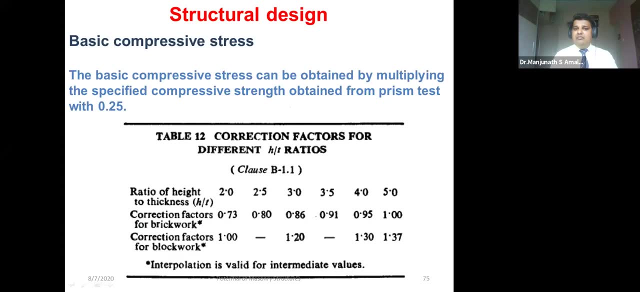 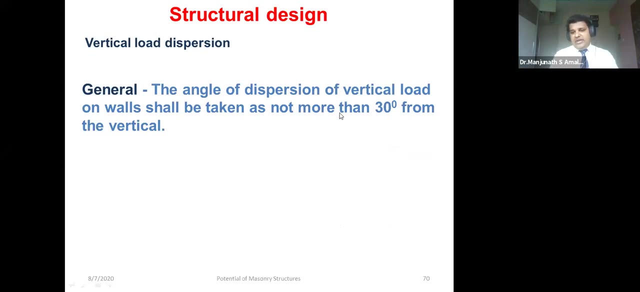 So you have to take the entire length of the wall as the one which is resisting the load. It has to be calculated for another length which depends on what I mentioned here with respect to the dispersion of vertical load and the angle. So that's for another day, maybe because of lack of time. I think you know, you know. 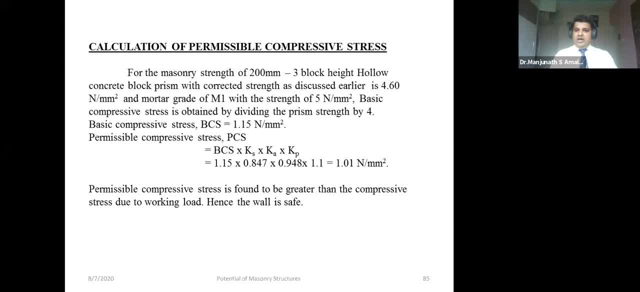 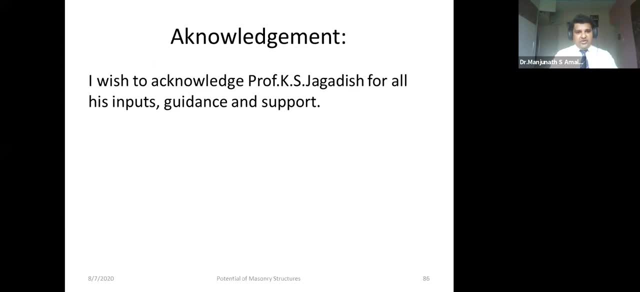 I would. I would end up my presentation with this wall and this is how we go about with the design. But well, at the, at the end, you know, I would fail in my duties if I acknowledge my, my academic mentor, Dr KS Jagdish, who has been my, you know, academic mentor, would. 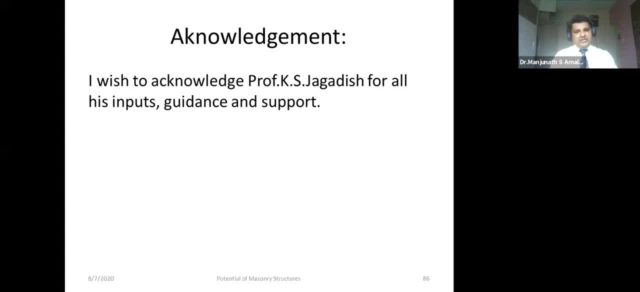 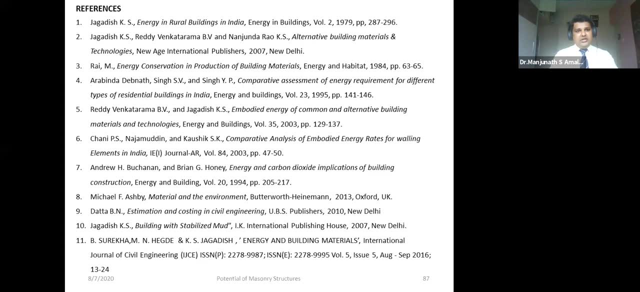 always be thankful for all his inputs, guidance and support throughout my academic- you know- career. And with this- this is the references you know- one can go about looking at most of the things with respect to the design Okay, energy from these references. well, thank you all. I hope I have met your. 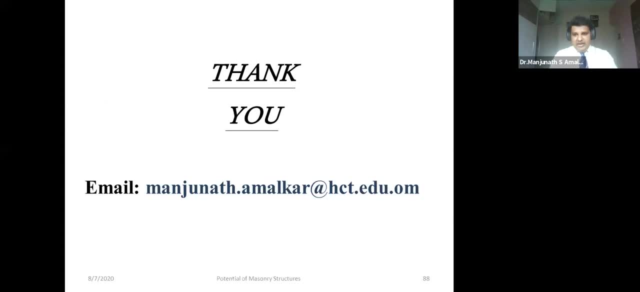 expectations, my friends. well, if you have any more doubts on this, well, you know, you can always, you know, email me your questions. I will be more than happy to answer your questions. well, I believe it, at this page, with my email ID here. so, if you have any doubts, okay, sir, sir, yes sir, thank you very much knowledge, I hope. 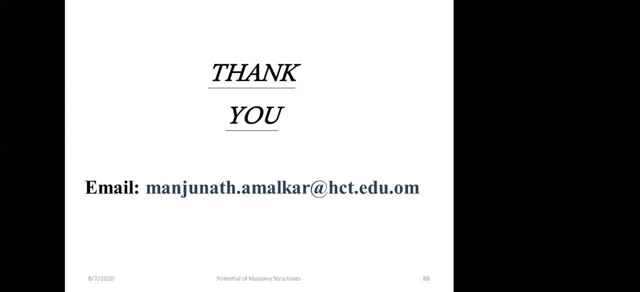 participants have gained a lot from your presentation. now over to Arun Kumar, sir. thank you, sir. so thank you for briefing out on today's topic and for sharing your knowledge. it was very clear and precise, thank you. it was more informative and once again, I would like to thank you for taking time out of your 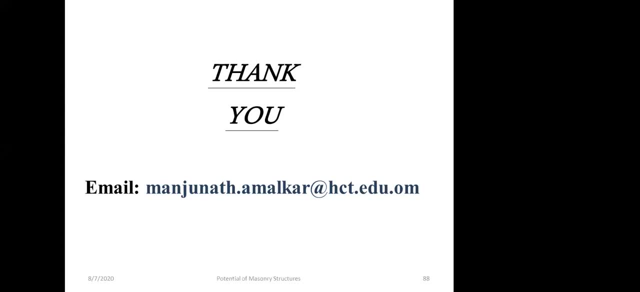 busy schedule, sir, and we are explained with an example design, so it was more informative once again. and now it's time to conclude today's webinar, and I kindly recommend you to subscribe to our channel and hit the bell icon so you don't miss out on any of the upcoming webinars, and I would like to request our 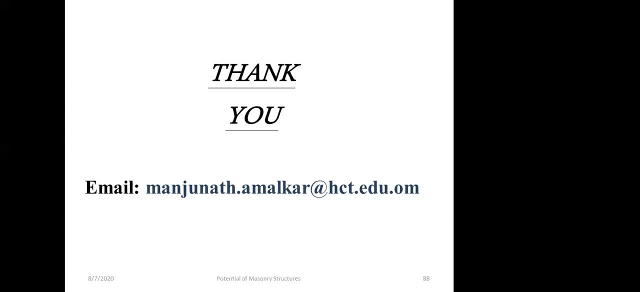 colleague, mr Kiran, sir, to propose the vote of thanks. so once again, once before. so before that, before, what a vote of thanks. any questions pertaining to the topic discussed in today's session I have been asked to drop in chat box and few questions have been asked in the chat. in the chat box I would like to call upon 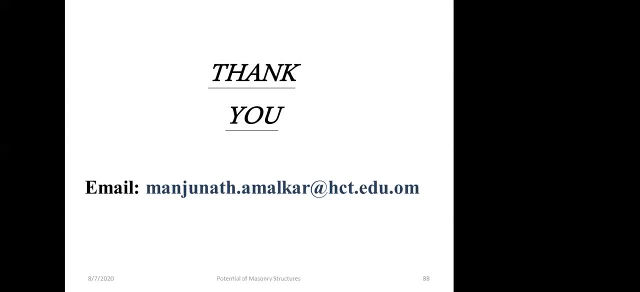 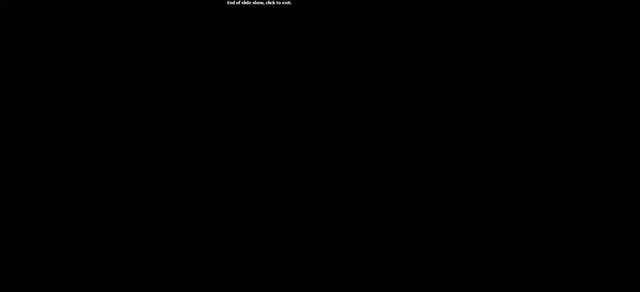 Ajaswari, ma'am, assistant professor, Department of Civil Engineering, to ask the questions in the chat box over to you, ma'am, there are a couple of doubts from the participants. sir, I'll read out those questions to you one by one. yeah, please. first question is from Amit Pratap Singh. 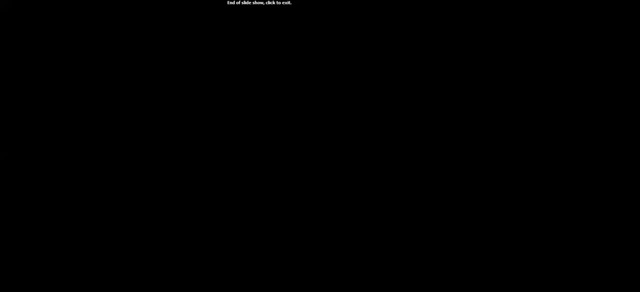 can we build masonry structures in earthquake zone third, fourth and fifth grade? how ductility is provided to masonry structure to resist lateral loadings, because masonry is brittle in nature. well, yeah, that's a very valid question. I think everybody has a concern about masonry structure being very 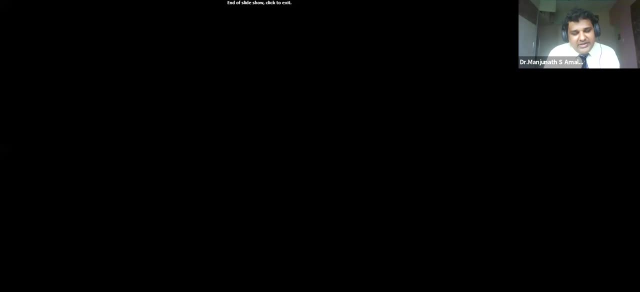 brittle. well, yes, by itself, you know, it is a very brittle material. but if one have to, you know, design it for taking the lateral loadings, well, just masonry will not be you enough. one has to go ahead with, you know, going ahead with this option of. 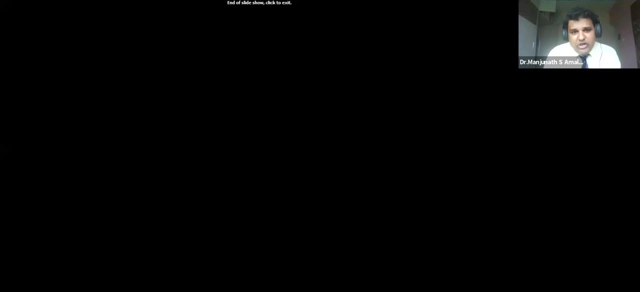 reinforced masonry where, you know, based on whatever is the design requirement, whatever a zone, has the panel as the, as the person has, you know, one would definitely have to go with, you know, designing it as a reinforced masonry. well, reinforcement, along with masonry, will make the element that much more. 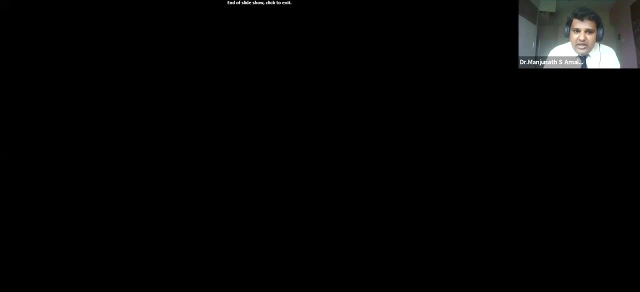 ductile and you know that will definitely be a solution for maybe taking up- you know the earthquake loading as well. apart from that, there have been a lot of, you know, other options also, like you, like they have something called as confinement masonry. well, if one had to go designing a 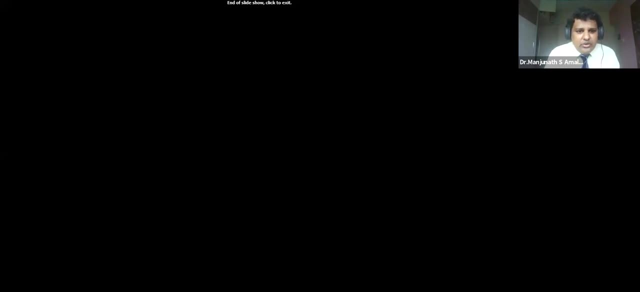 masonry for resisting lateral loadings or earthquake loadings, then well, you know, just a masonry would be the best solution for that. So if the masonry will not be enough, we'll have to go with a little more. we have to, you know, add a little bit of reinforcement with it, or maybe have 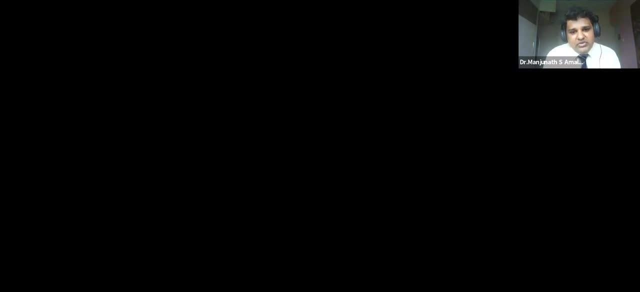 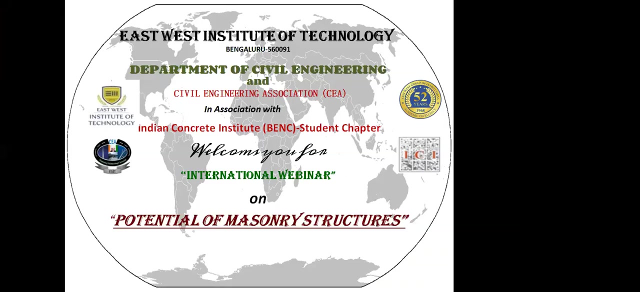 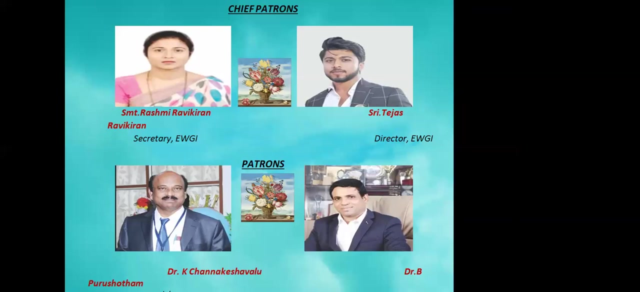 some more options, like the confinement masonry, which will be good enough in resisting the lateral loadings also. Okay, sir, the second question is from Tushar Patel. What is meant by bimodulus composition of motor? Well, you know, like you know, concrete, concrete. we assume that the material is homogeneous. 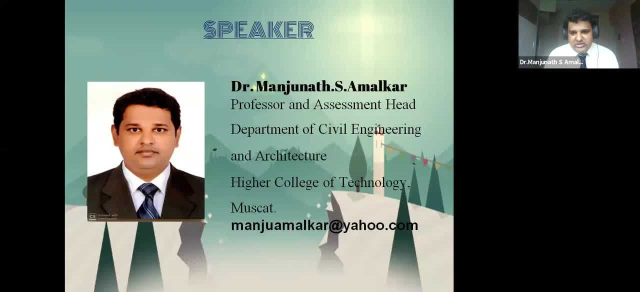 isotropic. you know material because you know that's, that's what we have, what we assume out of concrete. but when we talk about masonry, as I mentioned, you know it is a composition of two materials. one is a concrete, not necessarily concrete block, but any masonry unit. the other one is that of mortar. so each one have a. 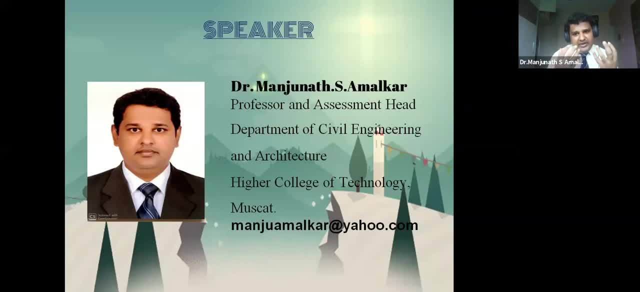 different modelness. Well, there is a different model of masonry. That is one reason why we look upon a masonry which is a constituent of these two materials, giving to having two different modelers. that is why we would look at it as a bimodulus material. 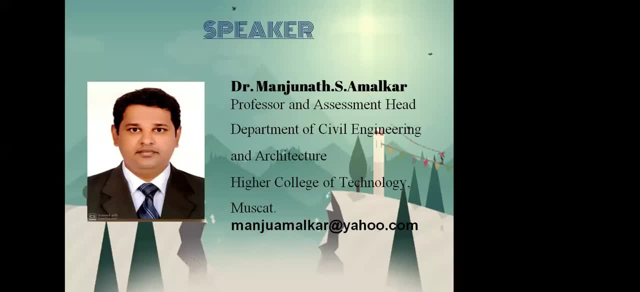 Okay, sir. the third question is from Sunny. sir, For masonry work with solid bricks, what should be the consistency of mortar: Solid, solid bricks? Yes, sir, Well, you know, big bricks are not going to be solid bricks. Yes, sir, Well you know, big bricks are not going to be solid bricks. 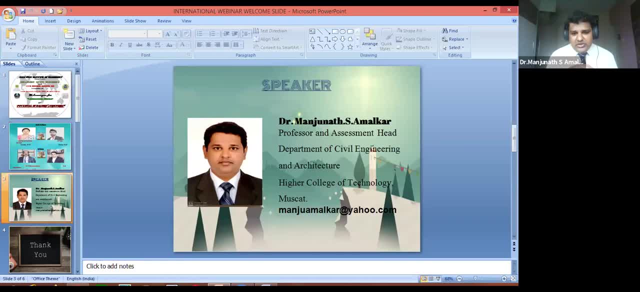 Yes, sir, Yes sir. Well, you know big bricks or any block or any other masonry. well, you know the mortar is a very important parameter. well, you know there are this one can perform the flowability tester from the flow table. and as for the literature, 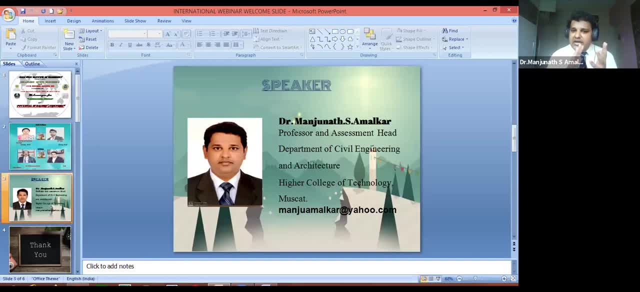 anything in the range of 95, let us say 100 to 110 mm, flow is, is is believed to be ideal, which can be used for the masonry. so any, anything between anything between you know, let us say 100 to 110 mm, slump the flow using the flow table. I think it would. it would be good enough for any masonry, even if it means for a brick masonry as well. 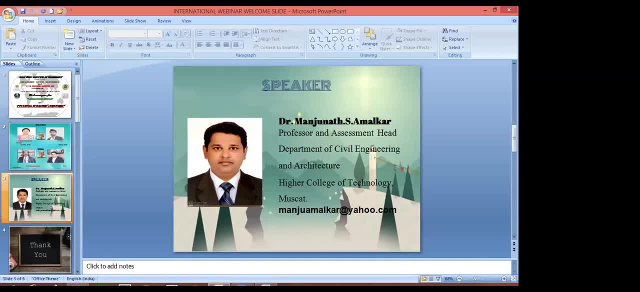 Okay, sir, thank you. The next question is from Shridevi ma'am: what about the water retentivity proportion in masonry construction? Well, that sometimes you know, in masonry that would maybe go as a hands on work. Okay, so the next question is from Shridevi ma'am: what about the water retentivity proportion in masonry construction? 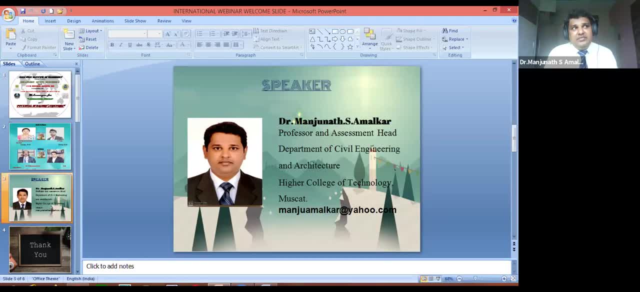 Well, that sometimes you know in masonry that would maybe go as a hands on work, as a drawback, because you know if, if the blocks are having a high water absorption, you know that would maybe one one drawback of masonry. but that can be, you know, that can be addressed, i think. 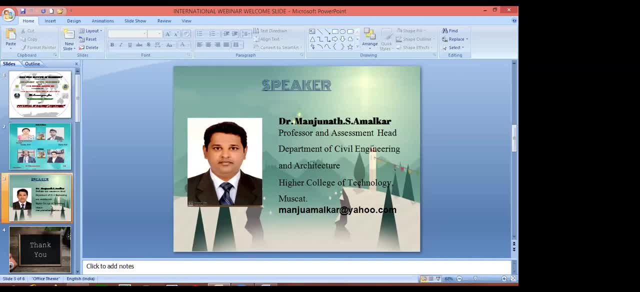 the, the, the kind of technology we have in the block making, one can manufacture good quality blocks which have a very low water absorption, be it water absorption or even be it the initial rate of absorption. and with the kind of technology we have, the kind of manufacturer players we have, 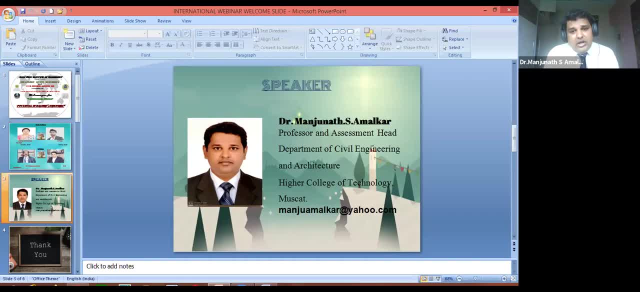 i think they are. they are able to make blocks which are which are very good in terms of its water absorption and, to that extent, even the retentivity of the water or the moisture within the blocks. okay, sir, one more question: masonry dome structure linkage will occur due to rainfall in clay brick have more moisture content? 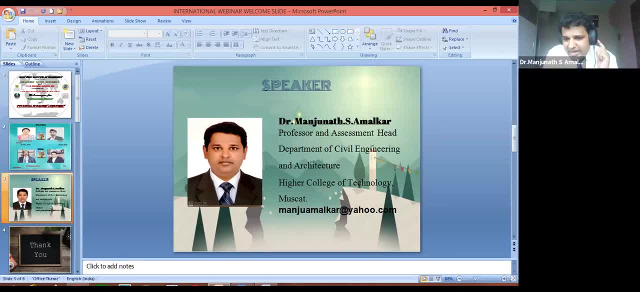 then what is the solution? sorry, i did not understand the first part of the equation. i'll repeat. i'll repeat, sir, in brick masonry dome structure linkage will occur due to rainfall. in clay brick have more moisture content. then what is the solution? uh, what? what would occur? because 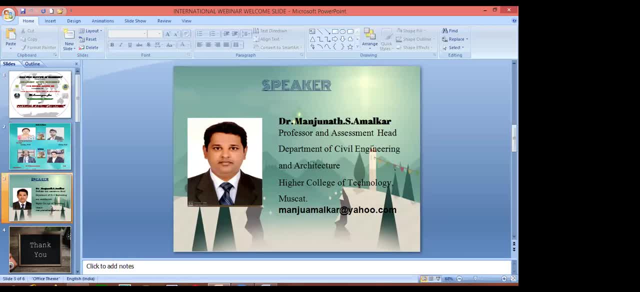 of the rainfall leakage. is it leakage? uh, well, i think i i doubt you know if it would. you know, leakage would be an issue in a doom. uh, well, i don't know if i have understood your question right, but uh, uh, you know definitely. uh, you know there would not be any leakage, uh, and it would be quite strong with the. 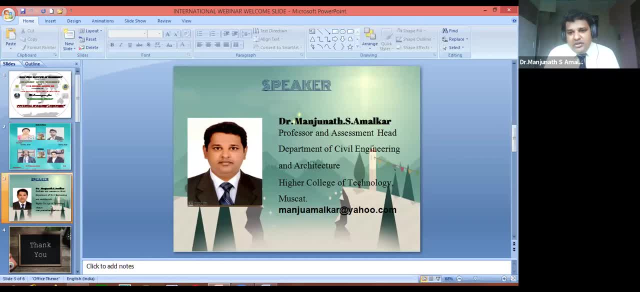 kind of blocks. of course you know when we choose the block for the uh, you know the doom construction uh will have to be a little bit careful about the kind of blocks. so, uh, with the good quality blocks, i'm sure you know uh what even that that can, that problem of leakage or the retentivity of water uh can be addressed. 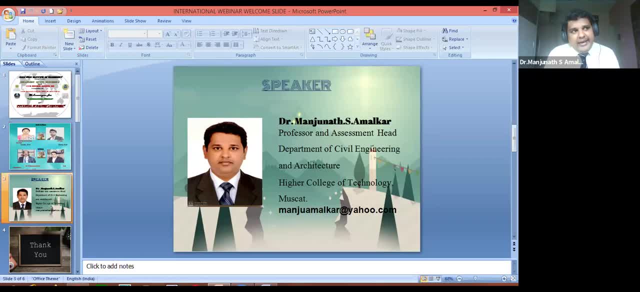 it. it again depends on what is the type of block and uh, of course, you know what is the kind of matter. uh, well, you know, the, the, the joint and the will will be uh quite strong and i don't, i don't think, you know, there would be any uh issues with the leakage, uh, unless the quality of the 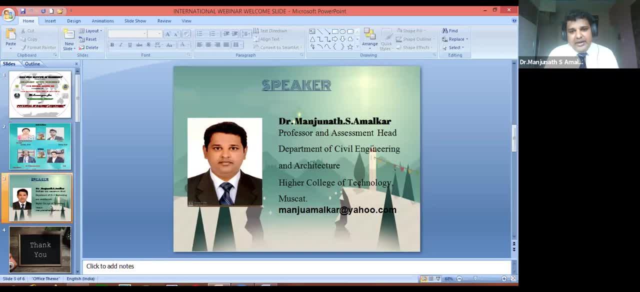 block itself is, uh, it's, it's quite bad, but you know, there is also, yeah, if you look into, uh, the southern, uh, india, southern portion of india, uh, well, uh, you know, and, and concerning the bricks, to be specific, uh, not, not strengths are achieved as compared to the north indian. 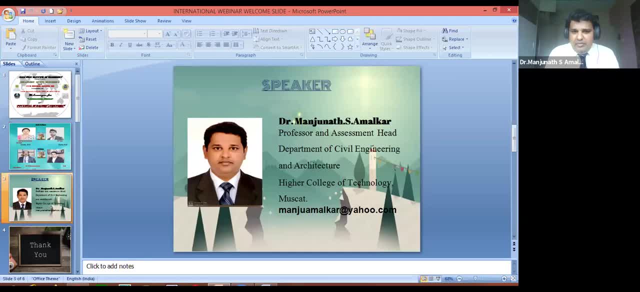 part because of the geometrical properties of the soil. but, yes, one has to be uh sure about the strength. it is audible, sir, it's not audible. uh, hello, are you? yes, yes, now, oh, it's audible. is it audible? yes, yes, okay. so the next question is from sahana: what is masonry white? 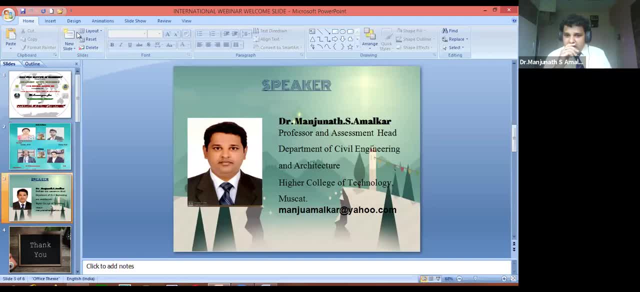 masonry: white, white, w y, h e earth, if i'm not wrong, i think i, yeah, i, i, i also come across this term. If I'm not wrong, it is the rammed earth, basically what one can understand with masonry. Okay, sir, One more question. Which joint should be avoided in brick masonry? Which bond is stronger in brick masonry? Which- sorry, Which joint should be avoided in brick masonry? And which bond is stronger in brick masonry? Well, you know, for masonry to be effective, the fewer the joints, the better is the performance of the masonry. 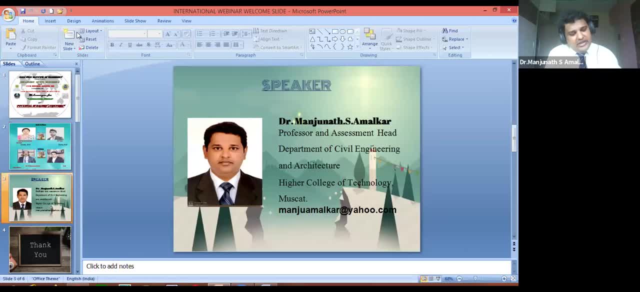 Based on the applications, I think one can go ahead with a particular choice, But if it is, let us say, hollow concrete block, well, one can go ahead with the stretcher bond. I think that is the best One, which will be the most effective, as per my understanding. 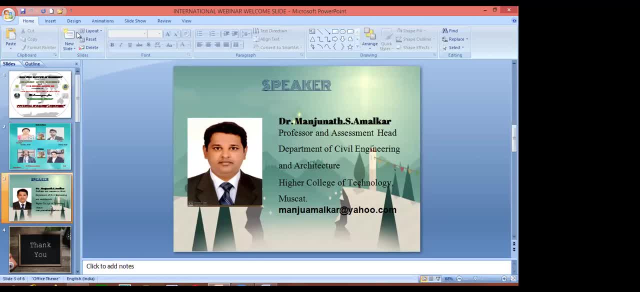 Are the geopolymer soil bricks cost effective? Well, the geopolymer blocks are the new addition which is, although you know you have geopolymer concrete, but then there have been a lot of research which has been done in geopolymer blocks. 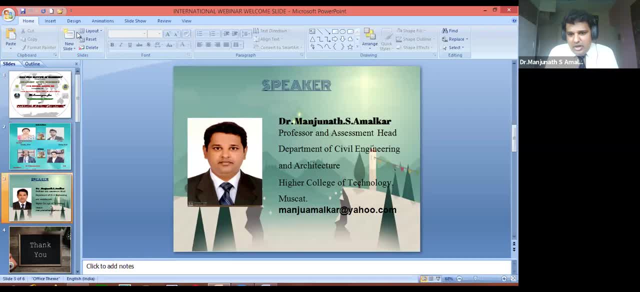 well, to be honest, you know I do not have much of a data about the geopolymer blocks, But as far as I know, well, in terms of the strength, well, one can achieve five to six MPa quite easily. 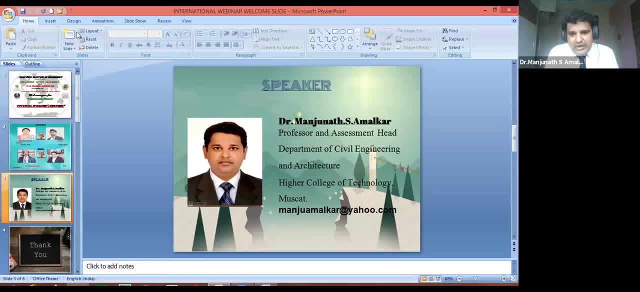 But the durability, their performance and the other properties have to be, you know, evaluated So to have a better understanding about that. So that is the, that is the key aspect of this new addition to the masonry unit. Okay, 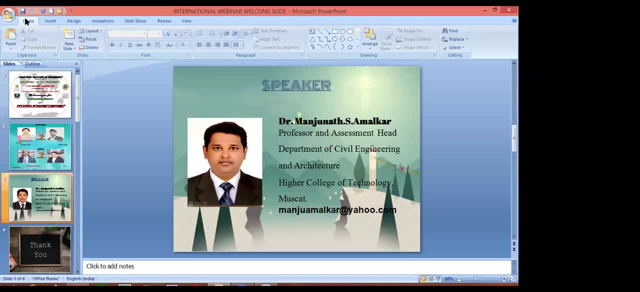 So last question, This question raised by KV Vijayendra, Sir, BIT College. So, rather than precise consistency of mortar, workability and pre-wetting of bricks is more important. I'll repeat once again: Yes, Rather than precise consistency of mortar, workability and pre-wetting of bricks is more important. 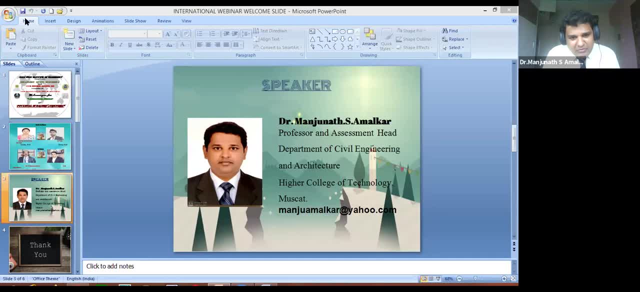 Yes, yes, I totally agree. I totally agree with Professor KVV, who happens to be also my teacher at BIT. Well, you know, the pre-wetting of blocks is a very important aspect, Because if the blocks are, you know, very dry, you know it so happens that whatever moisture is with the mortar, 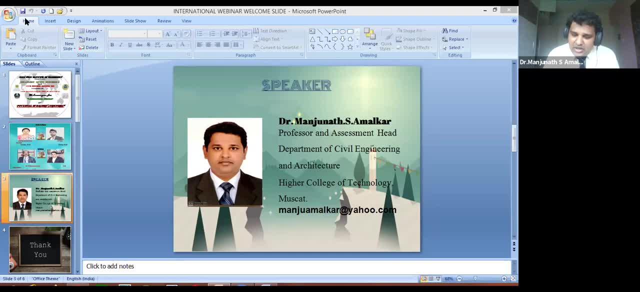 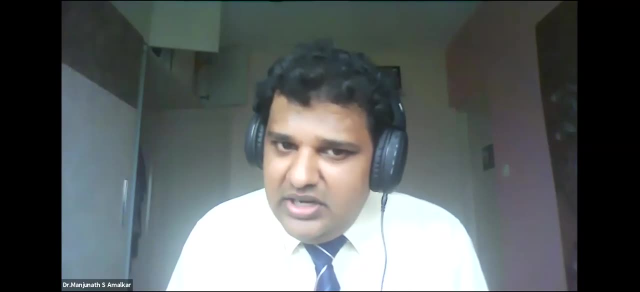 there is a tendency that the blocks, would you know, try to, you know, dry up. Yes, Yes, try to, what I can say, try to absorb a certain amount of moisture, so making the masonry bond a little more, what you can say, brittle. so that would definitely you. 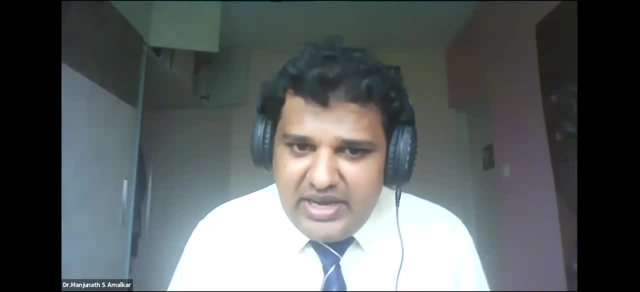 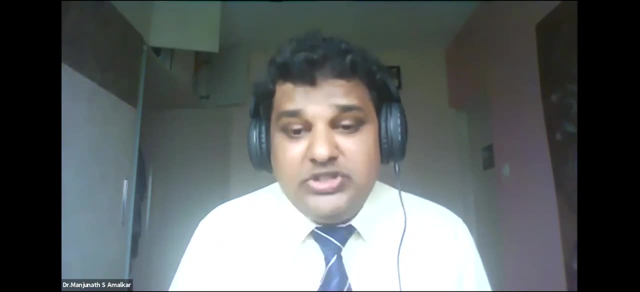 know, affect the, the strength of the masonry. yes, I totally agree with what professor said, that it has to be prevented, so that you know, you know it does not absorb any water from the Martin. so what water the matter has enough water with it to you know, for the process of hydration, but that's another. 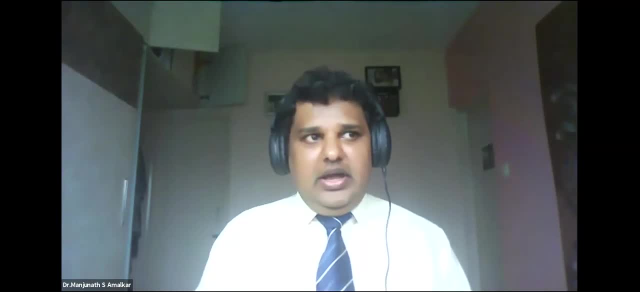 that that's a that's important point when one has to be absolutely sure that the blocks have to be pre-wet and then used for masonry. but yes, when I said a hundred to 110 consistency for the matter, well, that is as per the literature. 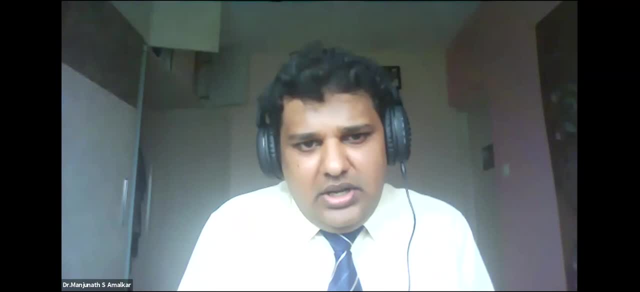 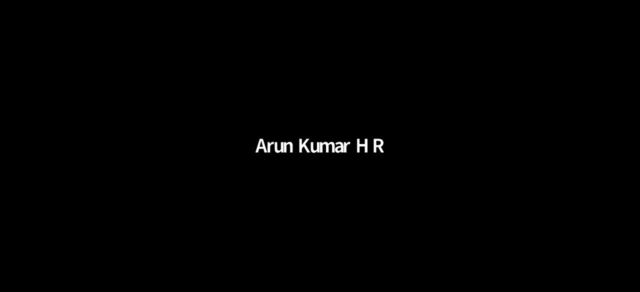 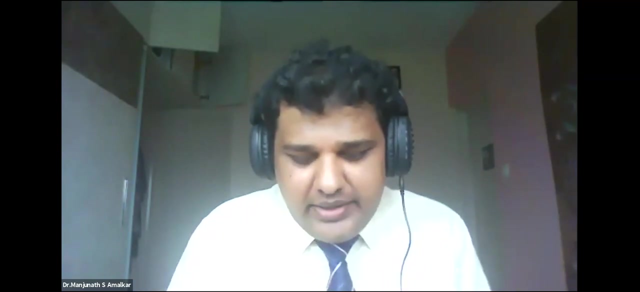 okay, thank you, sir. sir, one more last and final question. it's from Indra Sharma. so which is the most cost-effective, masonry or concrete work? well, you know, it depends on what is the, what is the kind of project which we are, which we are dealing with. well, you know, concrete, no doubt you know. 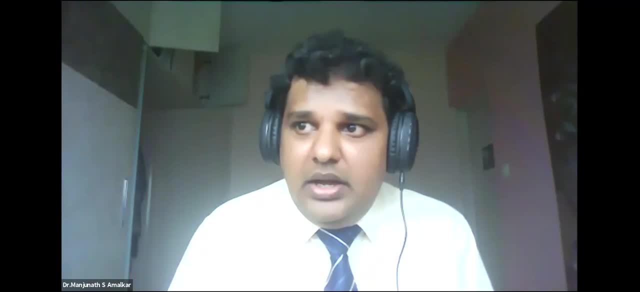 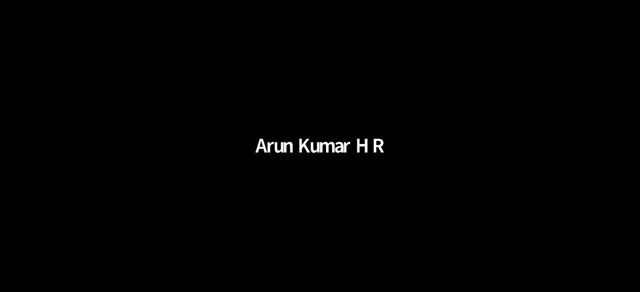 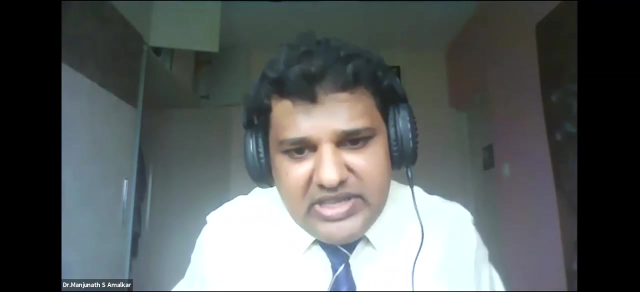 there are. there is a lot of what I can say, advancement even in the production of the concrete and its constituents. hello sir, kindly unmute, sir, it's not audible. yeah, I think someone has muted it anyways, so I whatever saying is well, the concrete also. it all depends on what. 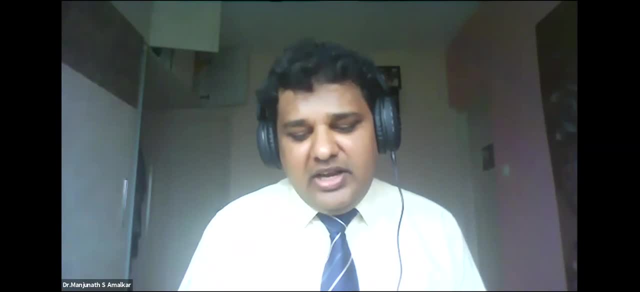 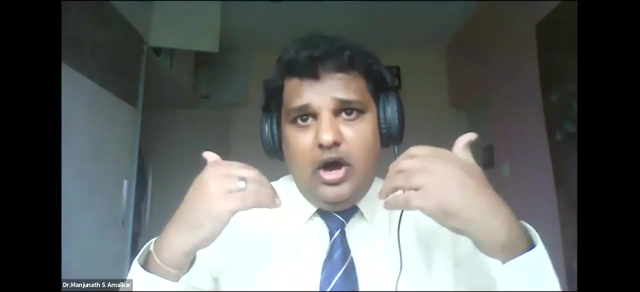 is the purpose of usage, although concrete, or there are a lot of advancement in the production of the ingredients of concrete also. which were they they? they play, they are also very, you know, very. they are taking a lot of care in getting down the product, the energy consumption or maybe the CO2. 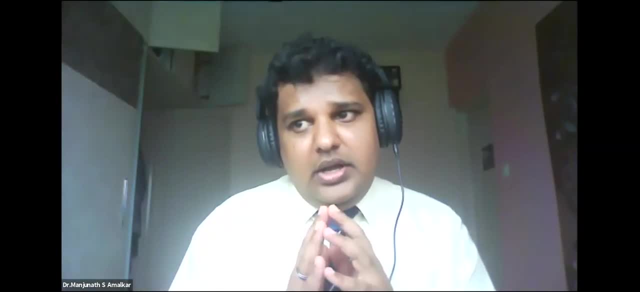 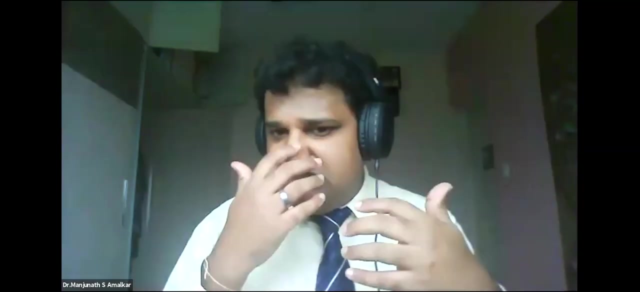 emission in the production of concrete also. so you know, it would be like a like it will all be dependent on what is the kind of project. Well, you cannot conclusively say, yes, this is better and that is better. Well, even the presentation is not that to do. 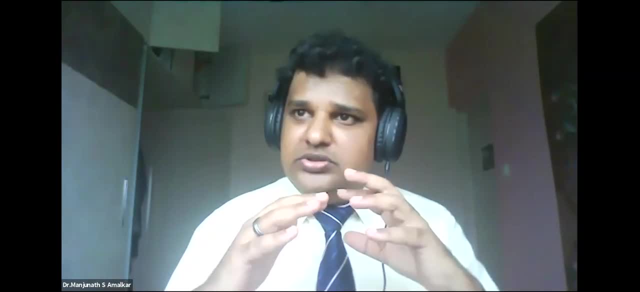 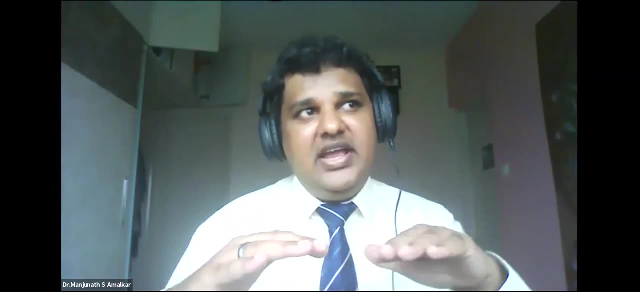 It would not be a fair comparison between the two. The idea was to just project, because everybody tries to fancy RC structures for even, let us say, a one-story building or even two-story building. So I think when there is an alternative technology, 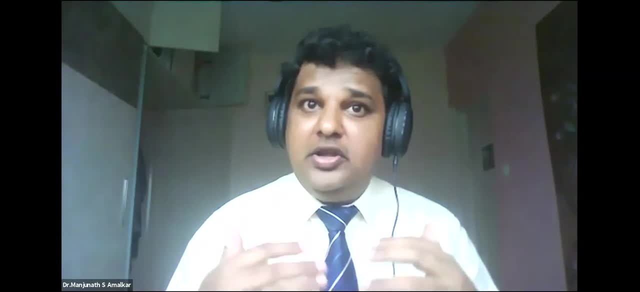 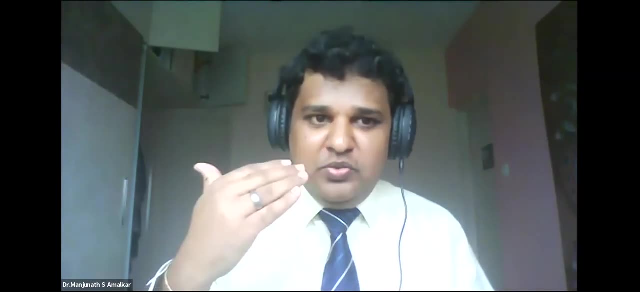 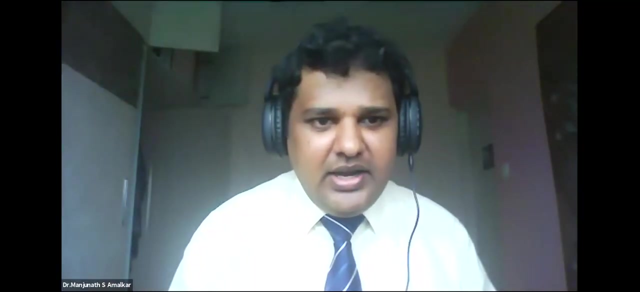 like you have it in masonry structures, then why not Sometimes the buildings, if it has become a trend? like the son does not want to live in the plan which the father has created, He would want to demolish the building and again go about constructing again a new one. 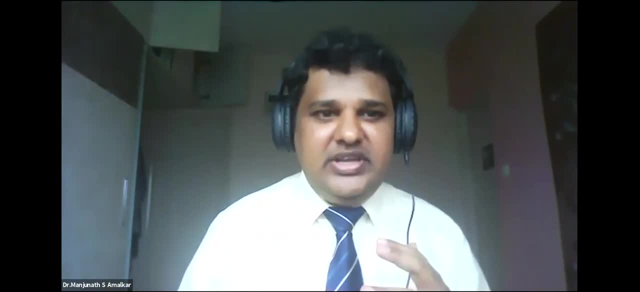 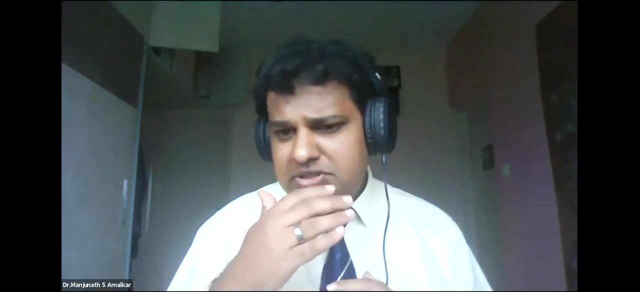 So if this is the kind of thing, why do we want so much of steel, so much of concrete, which is a little more energy-intensive material? rather, we can have such materials, such alternatives, which have been proven right from so many hundreds of years. 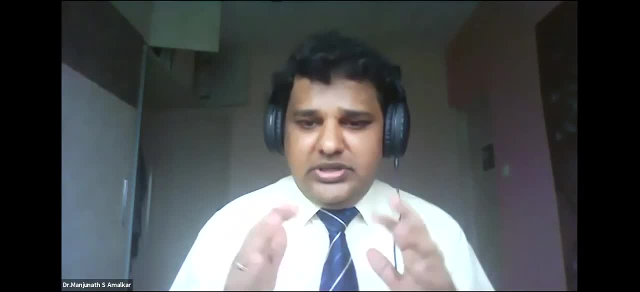 and it has the technology, it has the potential, then why not use it? But to answer the question again, it is very specific to the project. All I can say is perhaps with the dome construction which we tried, the ellipsoidal dome- we 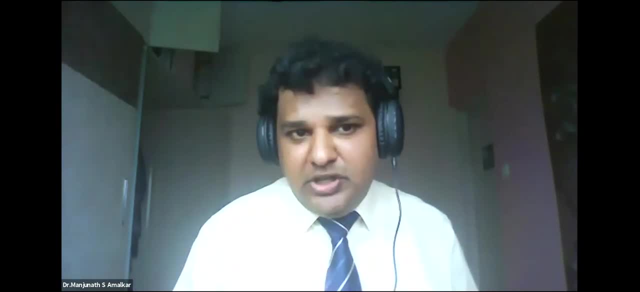 could straightaway get about, let us say, 40% reduction in the cost. Well, that was the idea, That information I can share, because this is what we calculated for the ellipsoidal dome We wanted, if we had to complete a concrete dome. 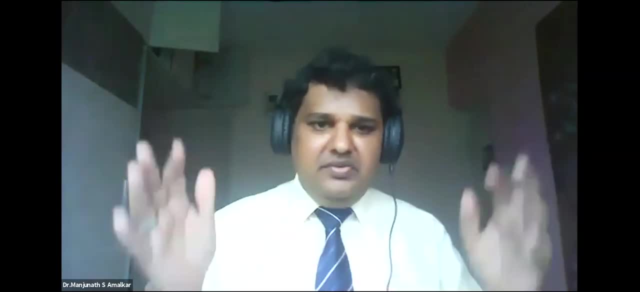 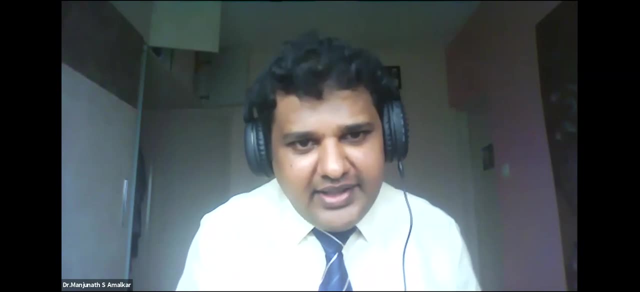 and compare it with the ellipsoidal dome which we have constructed, we could evaluate to have it as straight 40% reduction. I hope that answers the question. Yes, sir, Thank you. Thank you very much, sir. I think there are many more questions. 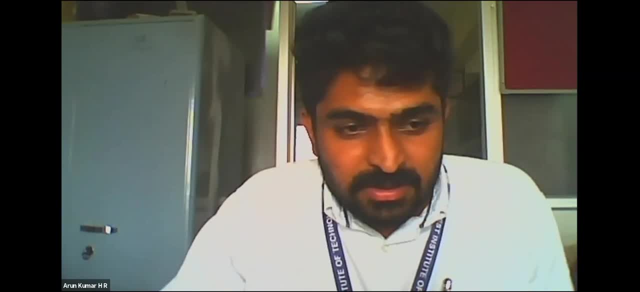 but due to time constraints, we can't be able to cover all those questions. Thank you. Finally, I would like to thank you once again for giving your time, sir. Now it's time to go. Thank you very much. Now it's time to conclude today's webinar. 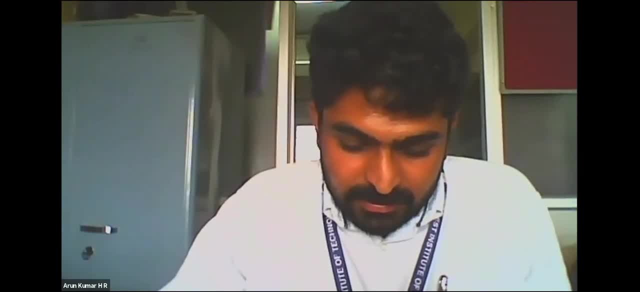 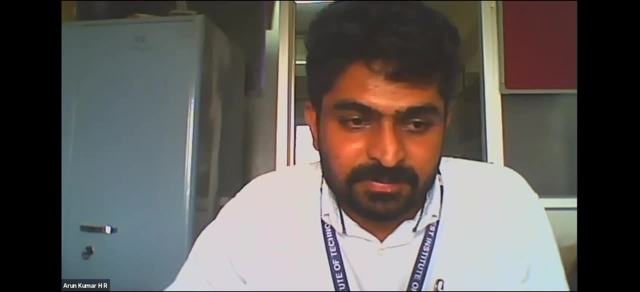 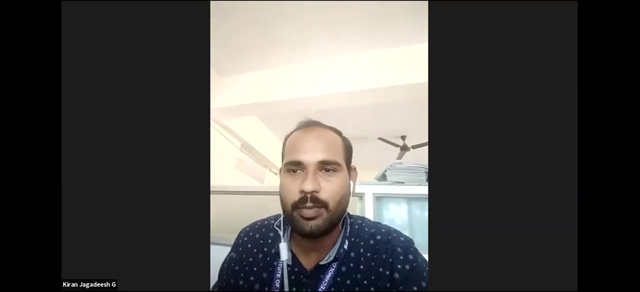 I kindly request our colleague, Mr Kiran, to propose the word of thanks. Kiran, unmute, Unmute, Kiran. Thank you, sir. Good afternoon, Anandal. Thank you for giving me opportunity for entering the vote of thanks, Honorable Chairman Srimati. 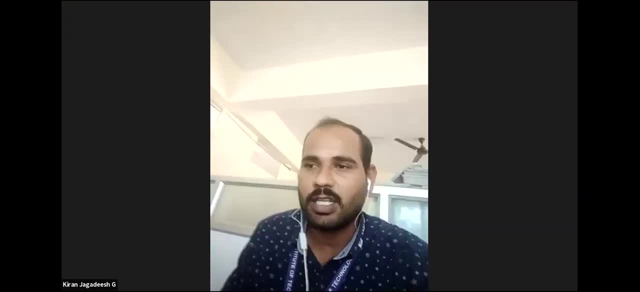 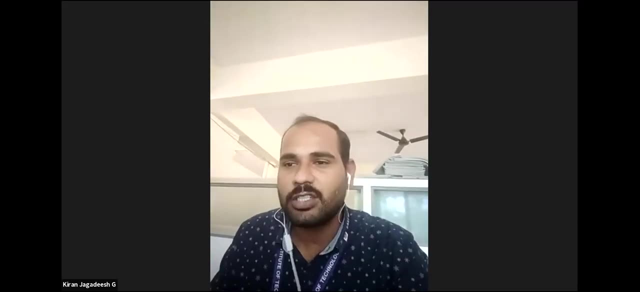 Rashmi Ravichiran. Madam Secretary, Mr Tez Ravichiran, Sir and Director, Dr Prashantham Sir, East-West Group of Institutions, Bengaluru. Respected and most distinguished chief guest of the day, Dr Manjunath. 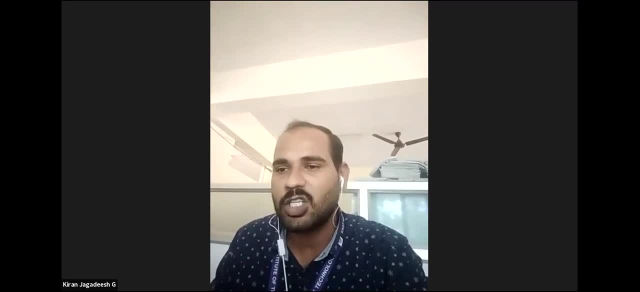 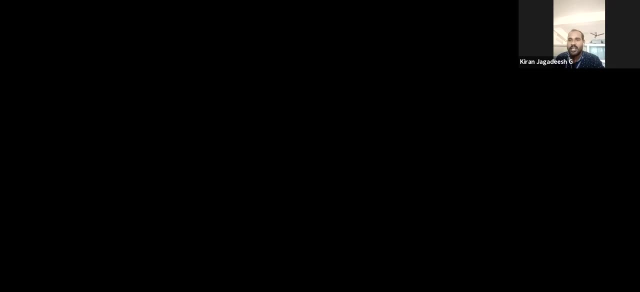 Samalkar, Sir, respected principal, Dr Chandrakash Ulu, Sir, our beloved HOD, Dr MS Nagraj Gupta. Sir, Honorable Professors, participants and my colleagues, It's my honor to propose a vote of thanks to all. 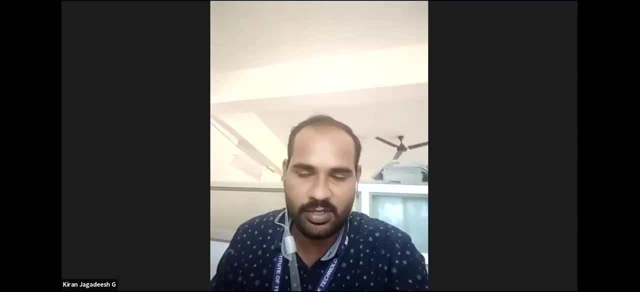 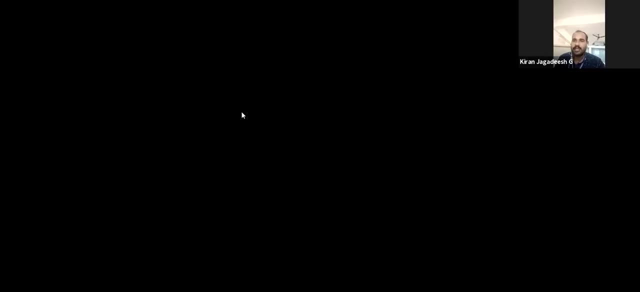 who have helped us in making this event grand success. First of all, I would like to thank our guest and speaker, Dr Manjunath S Samalkar, Sir, for making excellent presentation and making this webinar interesting. Thank you, sir, for your informative. 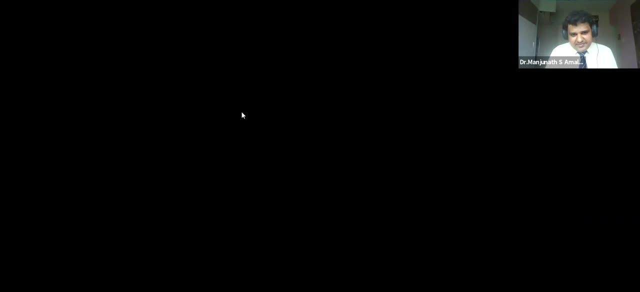 session. I would like to express my profound gratitude to our management director and principal for their continued support for conducting such event. I extend my special gratitude to Indian Concrete Institute Bengaluru Student Chapter for their support. I would like to thank the chairman, Dr LR Manjunath Sir. 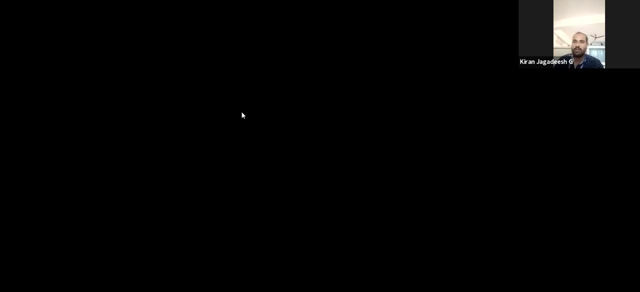 and secretary Dr Ariel Ramit, Sir Indian Concrete Institute, for their support. I extend my special thanks to Professor TVL Rangnath, Sir, Department of Sew Engineering, Higher College of Technology, Sultanate of Women, Muscat. I extend my big thanks to my colleagues for their 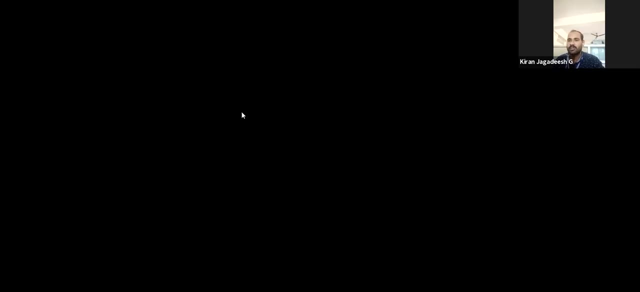 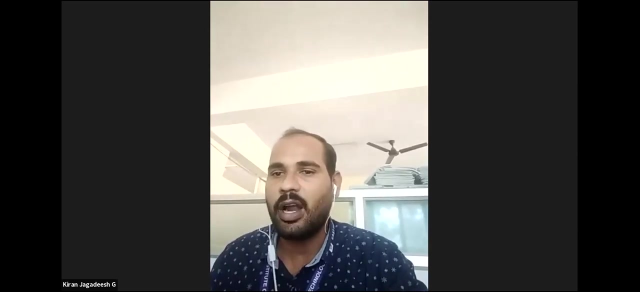 support and contribution for making this event successful, And also I thank our beloved HOD, Dr MS Nagraj Gupta Sir, for his continuous encouragement and guidance. I especially thank the convener, Dr MS Nagraj Gupta Sir, and coordinator, Mr Arun Kumar, and. 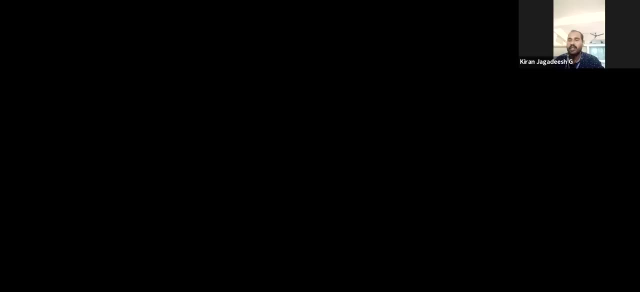 Mr Sunny K, who were the backbone of the event. Thank you, sir. Finally, the wonderful participants who have turned up in such great numbers from various places. Thank you so much for your cooperation. Once again, I thank you all for your cordial cooperation and precious listening. Thank you, Arun and all. 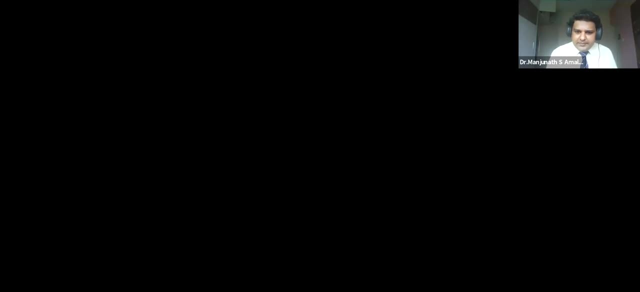 Thank you, sir. Over to you, Arun, sir. Thank you, Thank you. Thank you once again, Mr Kiran, for rendering you a vote of thanks. Thank you, all the participants, once again for attending, for your patience for so much, and I would like to thank once again. 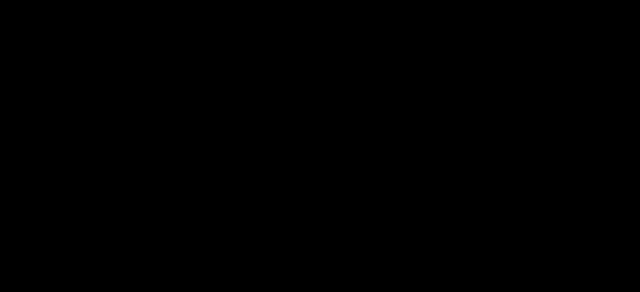 Dr Manjunath Amarkal Sir for giving your time and for sharing your knowledge. Thank you, Professor Arun. The feedback will be shared in the webinar group as well as the chat box. now, Thank you, Thank you.